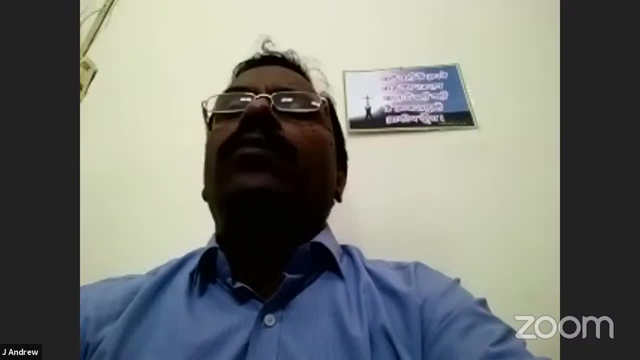 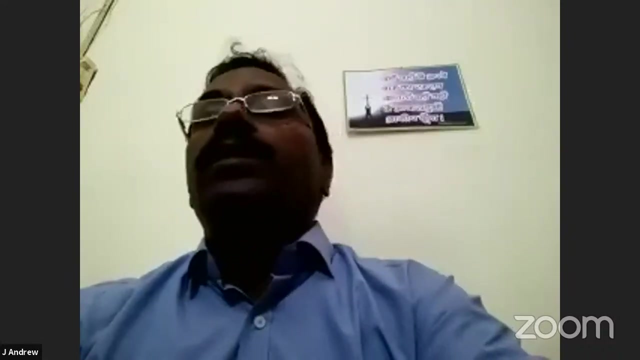 equity and allow all people to have equality lives, quality lives. Let our land have peace and be relieved from calamities. Bless the patrons, organizers, speakers and all the participants of this program. Bless St John's College and make it a beacon of light to this nation. 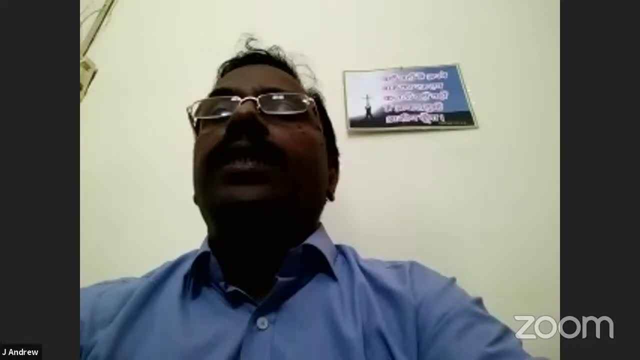 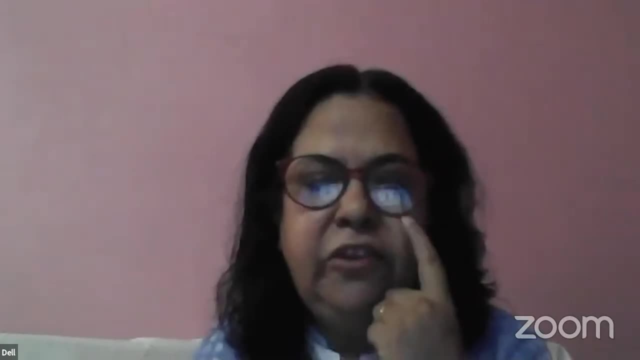 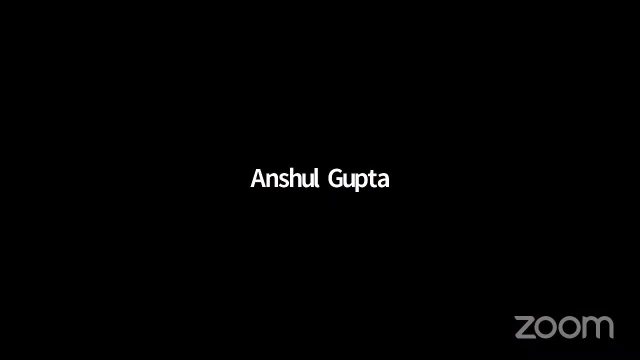 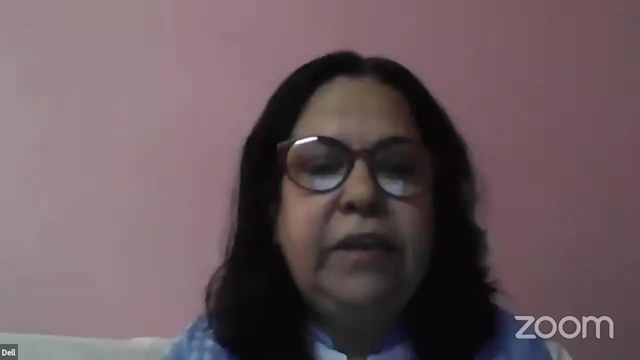 Thank you for hearing us. In the name of Jesus, we pray Amen. Thank you, Dr Andrew. Respected Vice Chancellor, Please mute yourself. Respected Principal Professor SP Singh of St John's College, Agra. 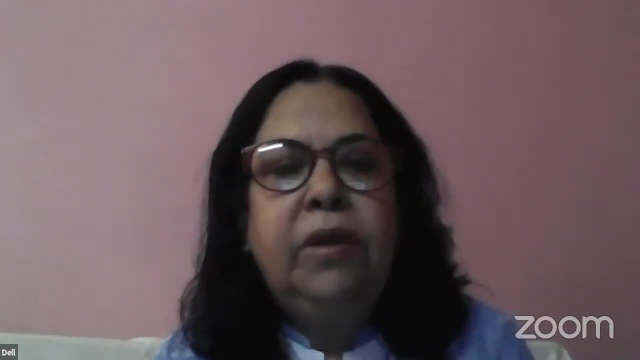 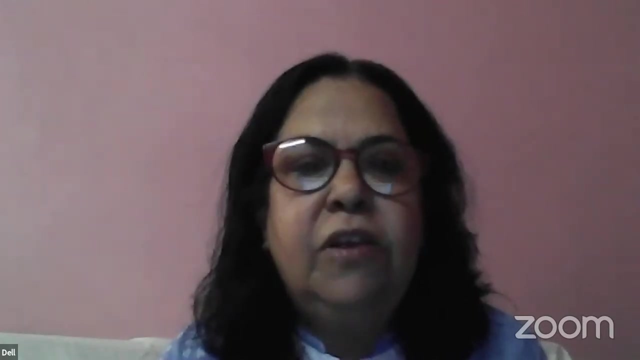 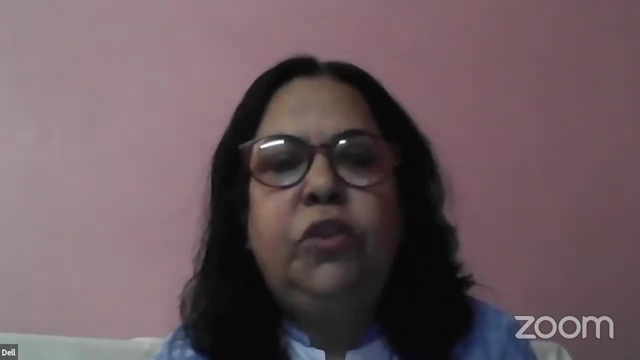 Respected Resource person: Dr Philip Muthulu, Head of Department of Geography and Chairperson of the webinar series. Dr PA Majeed. All the co-conveners: Dr Vidhur Grace, Dr Rohan D'Souza, Dr Shalomin Massey, Dr Preeti Massey. 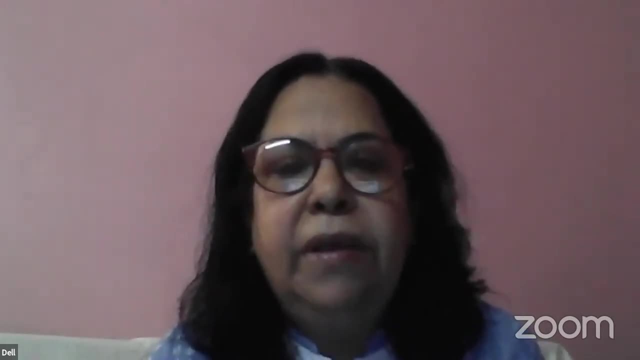 Dr Mahima Haabel And Dr Rohan D'Souza, Dr Shalomin Massey, Dr Preeti Massey, Dr Mahima Haabel and Mrs Bo-Daro Bandar. 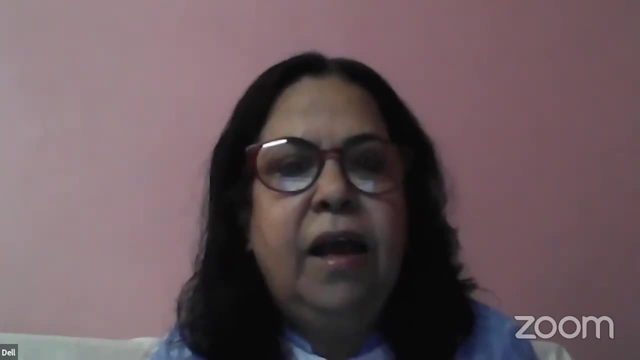 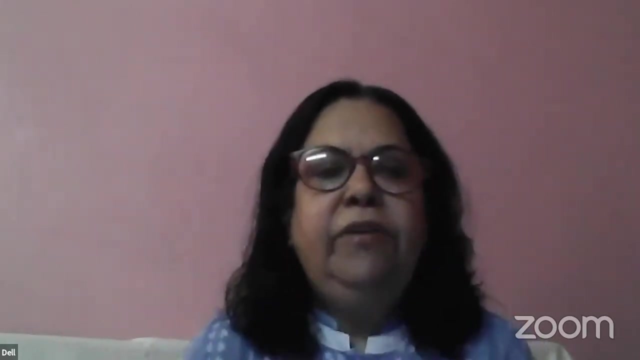 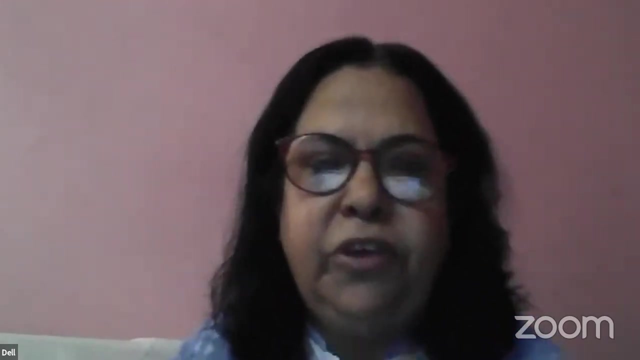 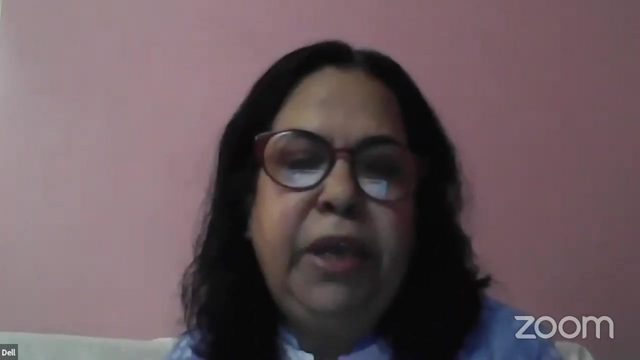 Barkha Bains-Single. A very good morning to you all. Today's topic is flood forecasting, and we have Dr Philip Muthulu to give us a talk on the same subject Now. flood forecasting, I feel, is the right topic to discuss. 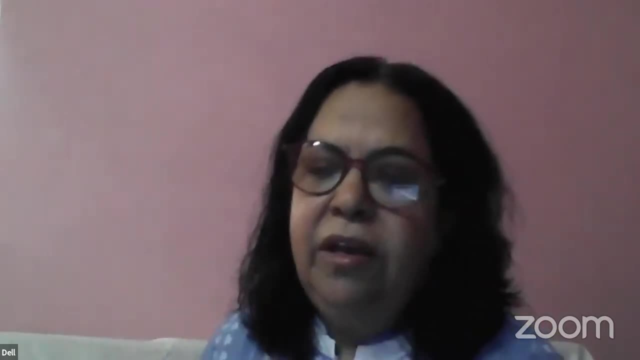 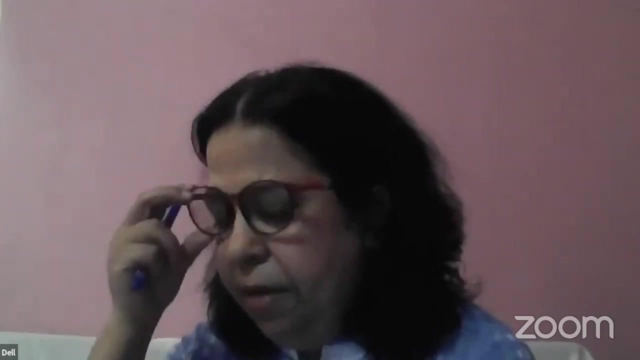 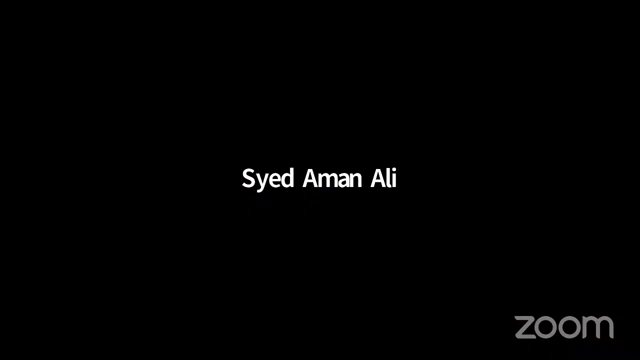 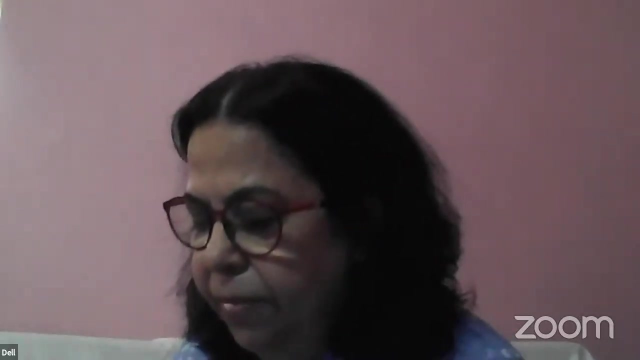 at this very hour of the year and the time of the year, as several parts of North East and Eastern India are experiencing a flood-like situation, As multiple weather stations in Assam, Sikkim, Meghalaya, Bihar and sub-Himalayan West Bengal. 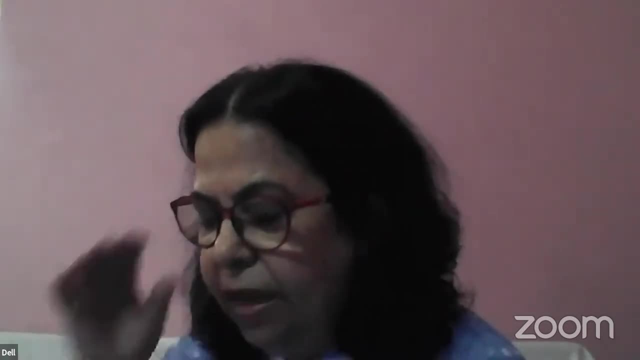 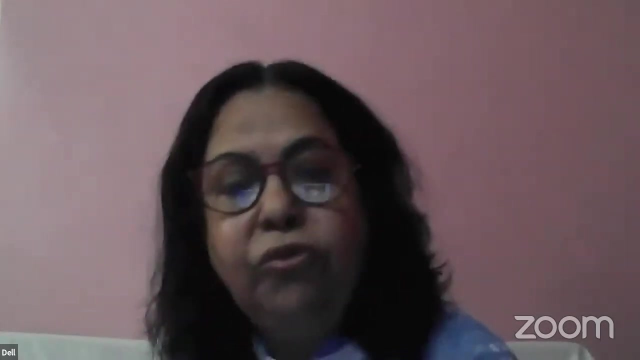 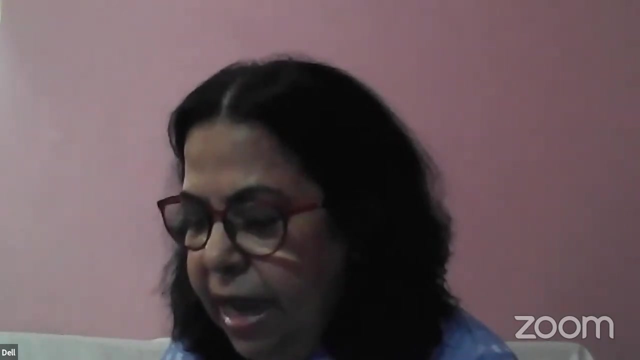 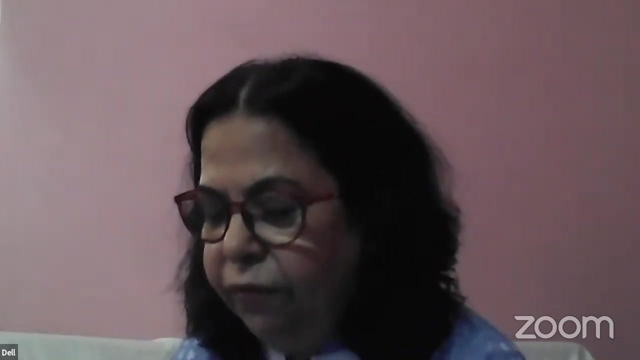 have reported extremely heavy rains that is, above 20 centimeters in the last two to three days. According to officials from the IMD, the eastern end of the monsoon trough continues to run along the Himalayan foothills with the convergence of strong southerly and southerly winds. 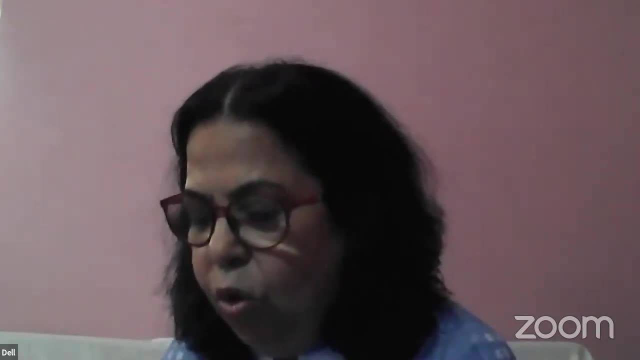 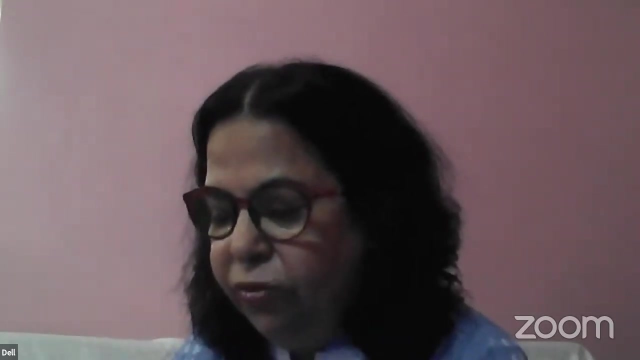 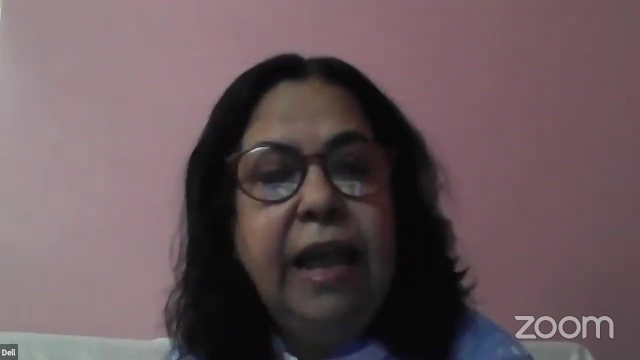 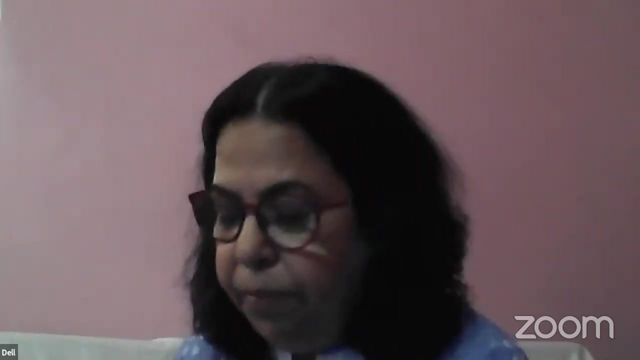 The south-westerly winds from the Bay of Bengal over Northeast and East India. This is likely to lead to heavy and widespread rain in many parts of Northeast India in the next four or five days. Assam is reporting floods. Bihar is also in a flood-like situation. 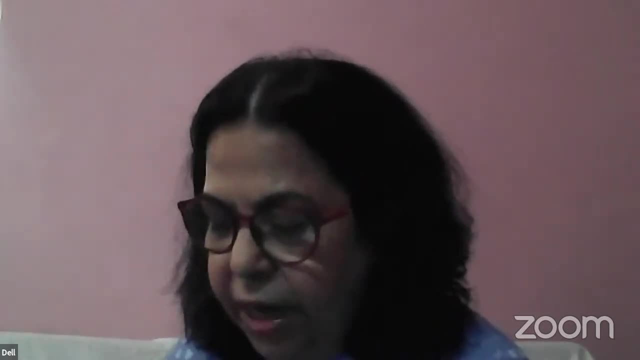 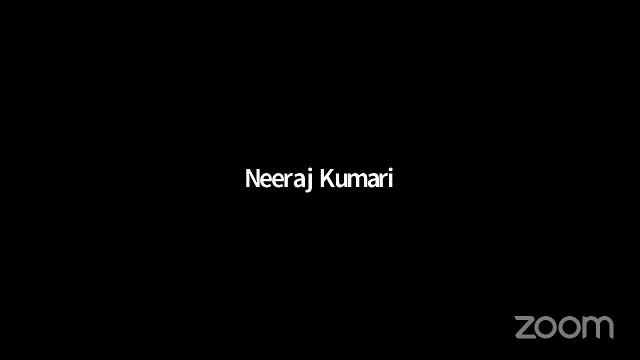 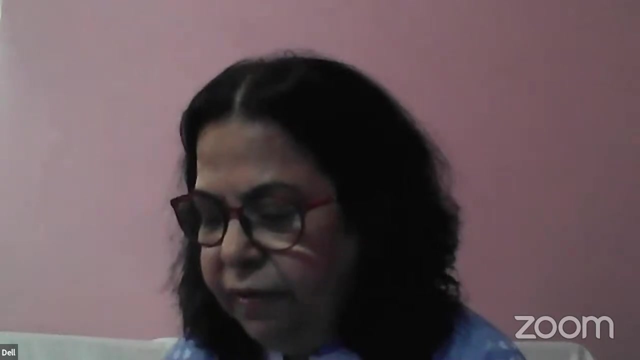 Siddhapunji, which is known to receive a lot of rain at this time, has reported as much as 50 to 55 centimeters in a day. This pattern of continuous heavy rain will gradually reduce from today to the 9th second. 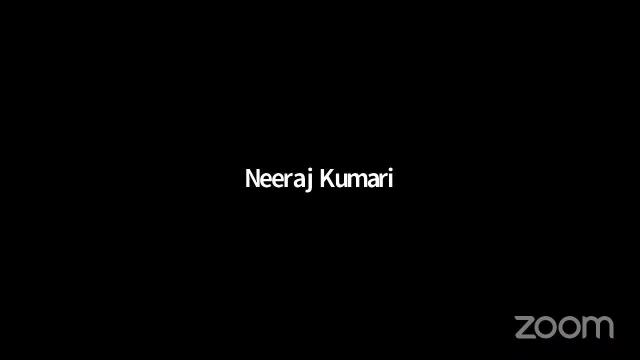 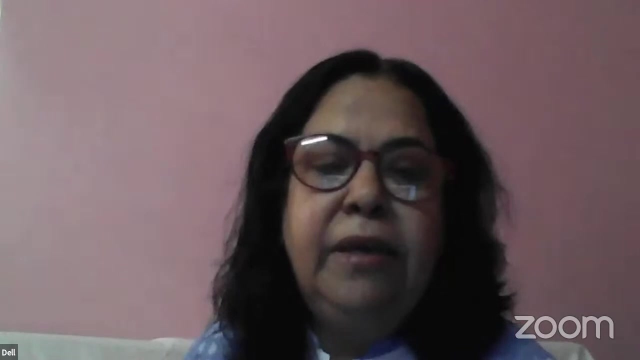 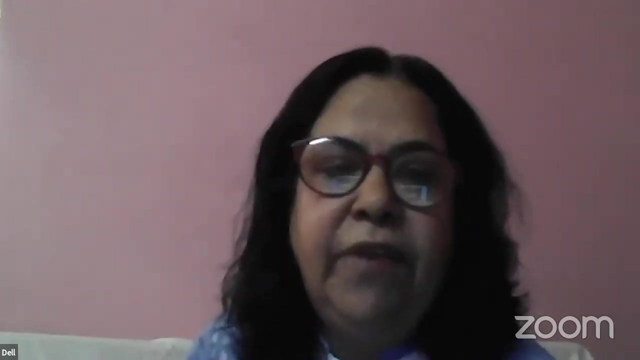 Rains will increase over central India and West Bengal, And from July 5th we can expect rains to resume over Northwest India. And when the rains will resume, we have to be prepared for floods And for this, flood forecasting is very important. 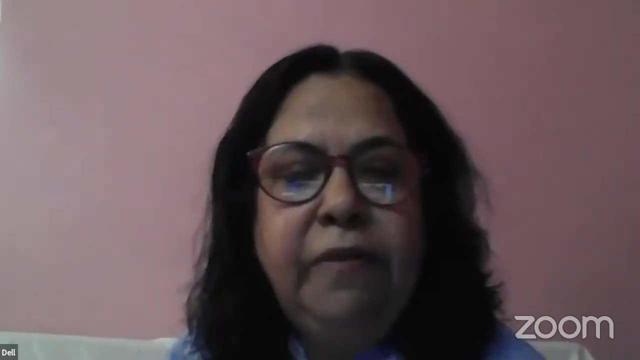 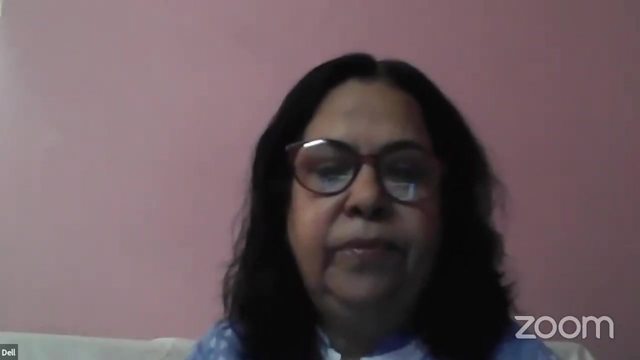 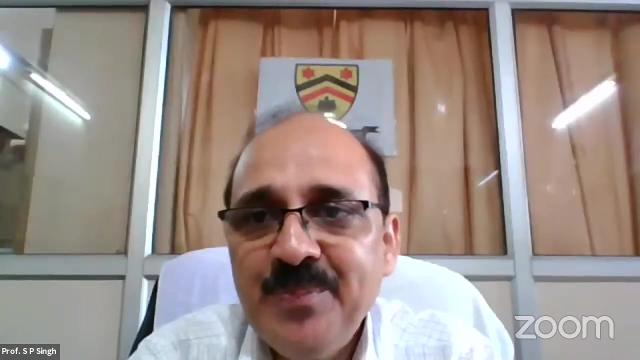 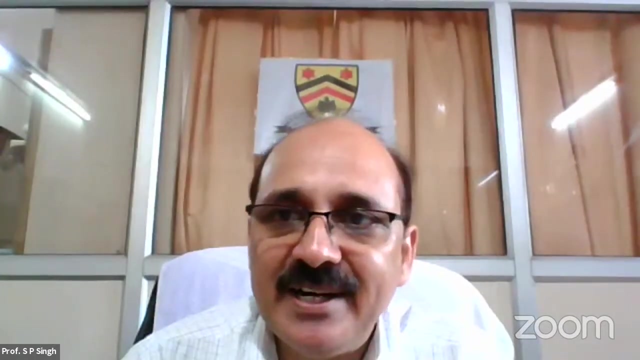 So now I will request our principal Professor, SP Singh, to say a few words. SP Singh is the resource person of the day. Dr Philip Muturu, convener of the program. Dr Neelia J Chauhan, Dr Jay Andrew. 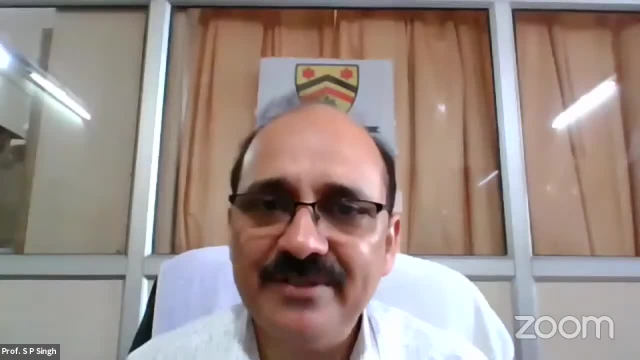 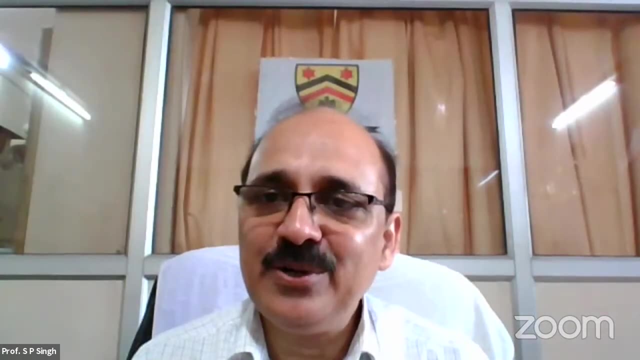 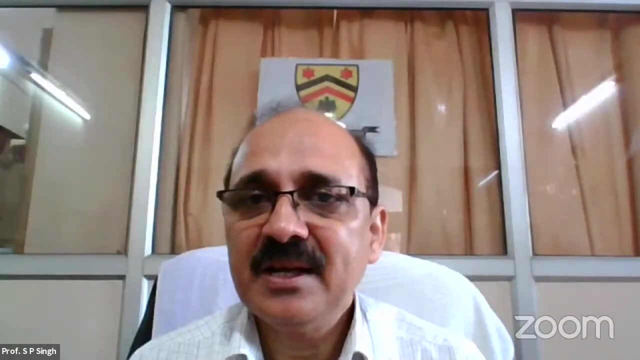 and various co-conveners of the program and dear participants, It is indeed a pleasure to have you here today. Thank you very much, delighted to be part of this program on flood forecasting. Earlier we had another webinar in which Dr Philip was the person and we were thoroughly enriched. 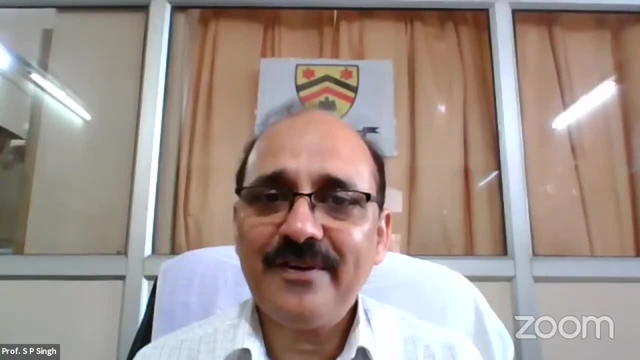 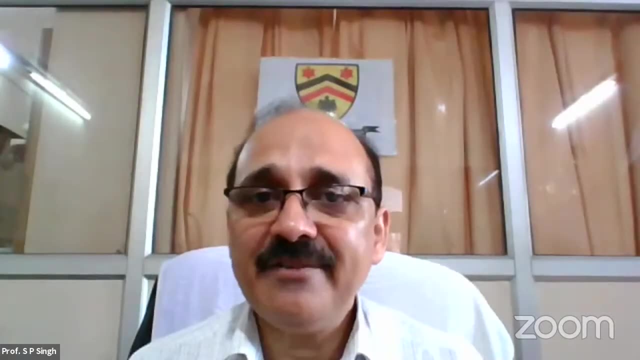 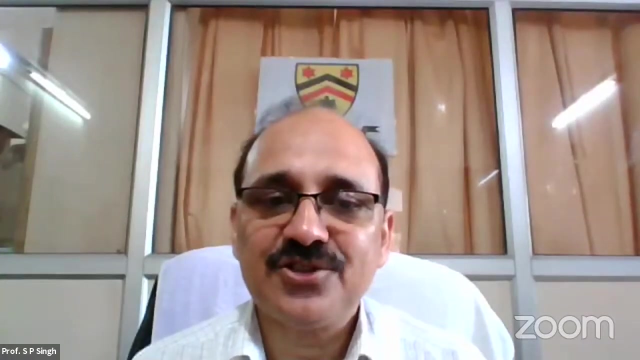 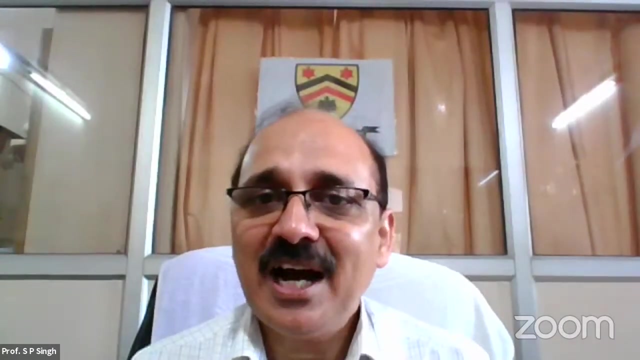 by his wonderful presentation and lot of ideas he provided us on the process of flood mitigation and today we expectantly look forward to this conversation, his talk or deliberation on flood forecasting. On behalf of St John's College, I extend the resource person and everyone a very 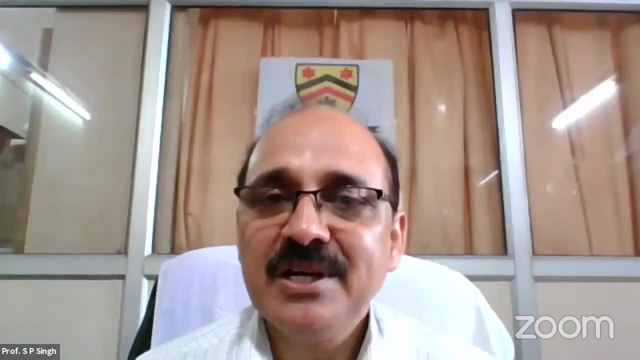 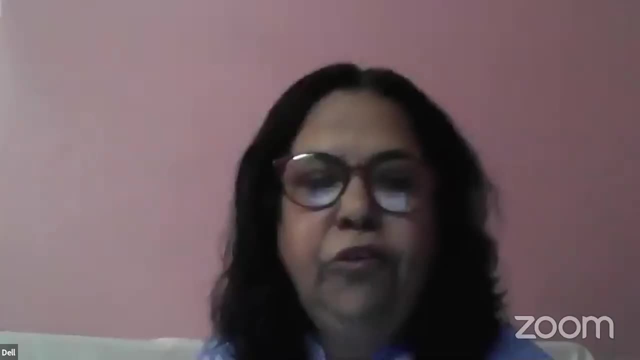 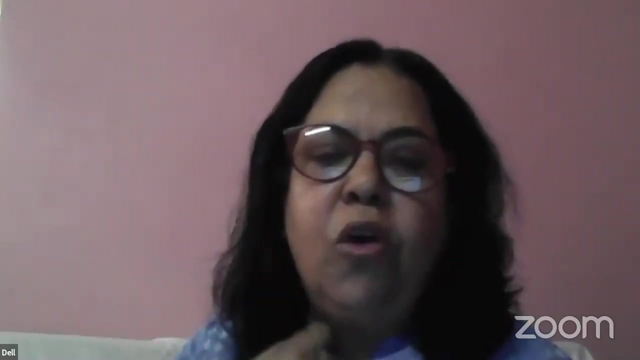 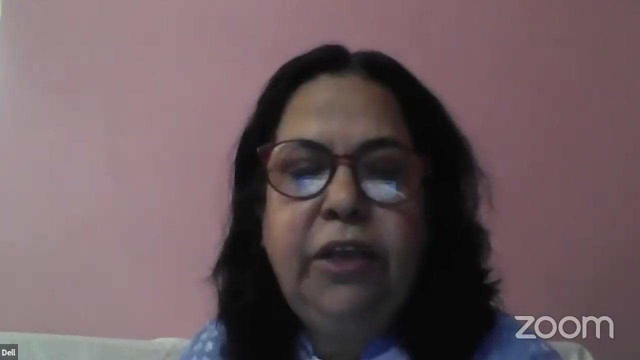 hearty welcome and wish everyone a very enriching and meaningful time. Thank you, Thank you, sir, And thank you, Dr. Your encouragement, your support and your constant help is the one, is the power behind all that we can do. Thank you so much, Sir. now I will. 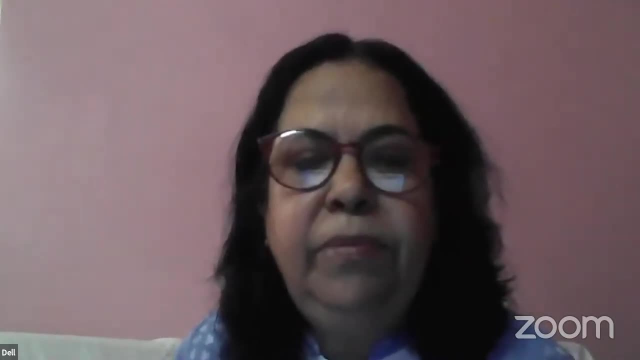 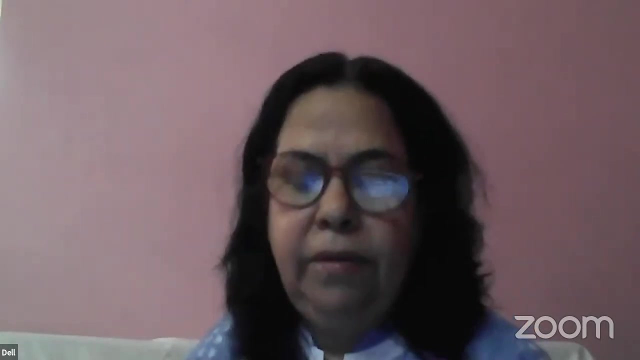 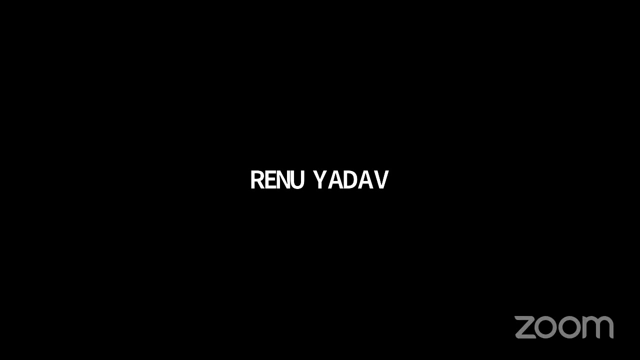 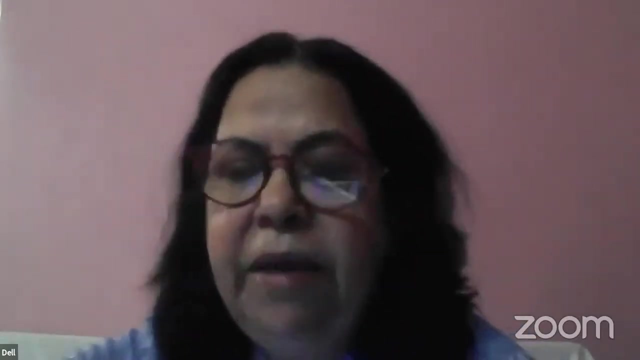 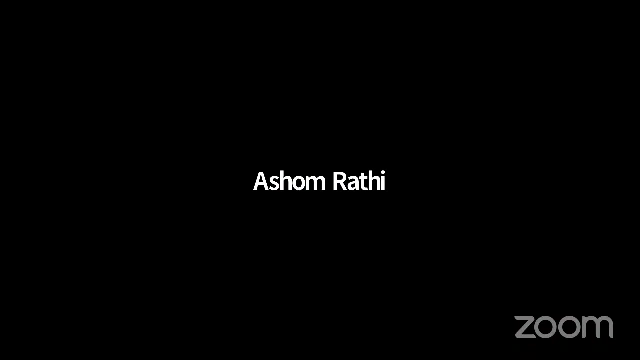 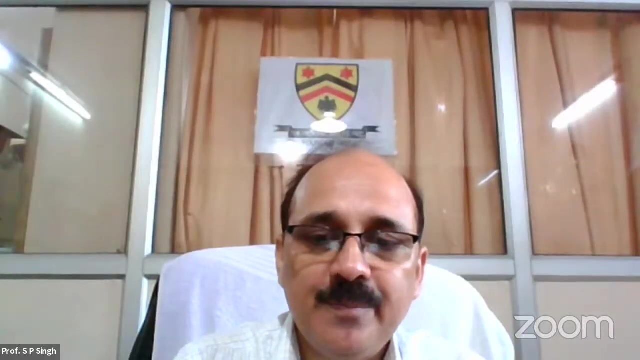 call Dr P A Majid to please welcome the keynote speaker for the day, Dr P A Majid. Can we connect to Dr P A Majid please? Dr Majid is not here, So probably you could do. 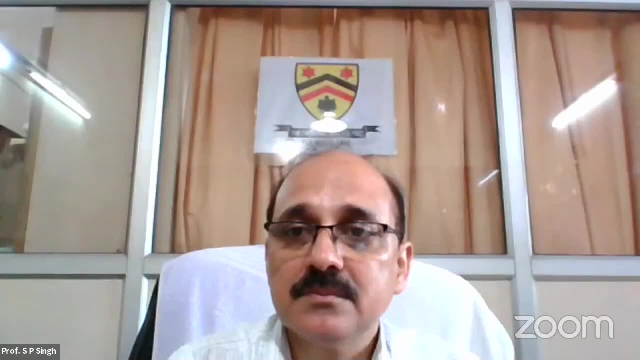 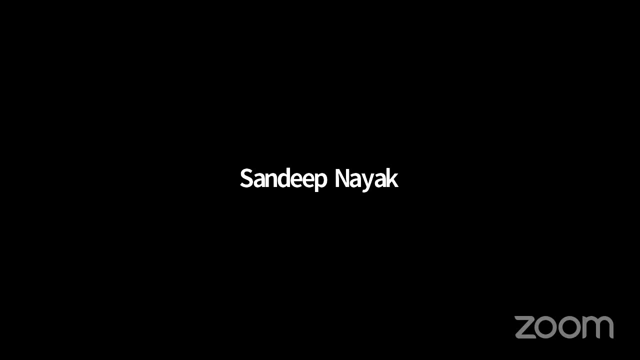 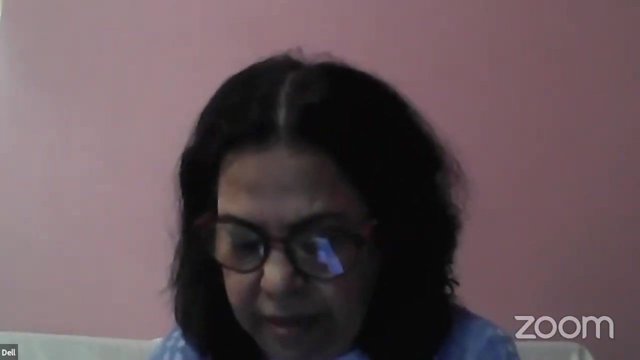 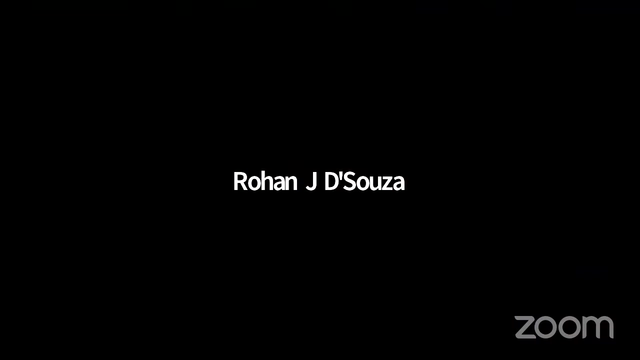 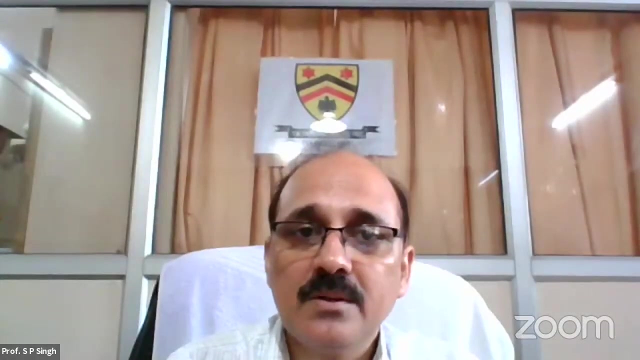 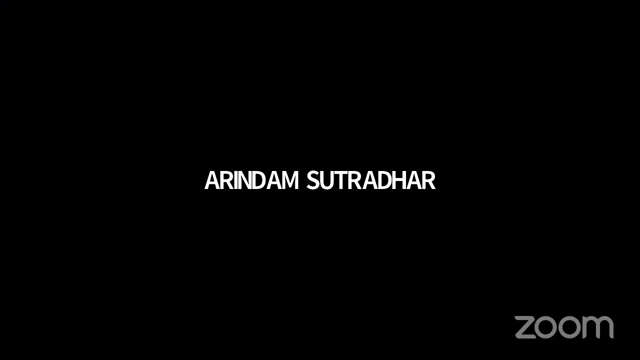 Dr PA Majid. is he there? I don't think he's there. He seems to be there, but I think he's on mute. Just a moment, I can't see him. Majid sir, please unmute yourself. 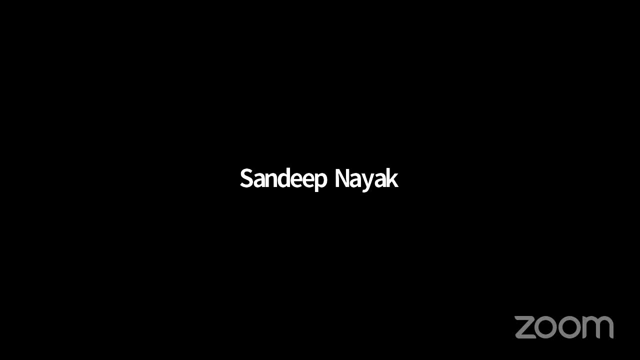 Majid sir has not connected today, I think. Okay, Monsoons and network connections: No, he is connected, but there is some problem. Hello, Good morning. Yes, We can hear you, sir. Yes, He's muted again. 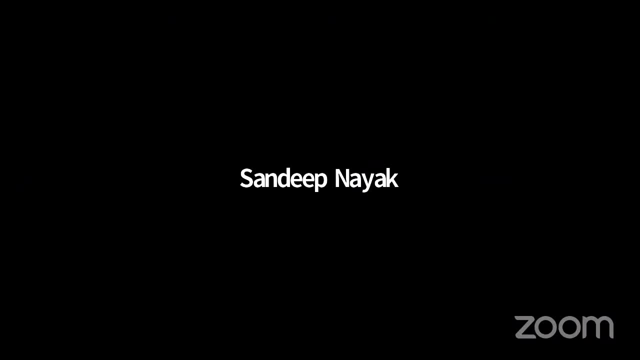 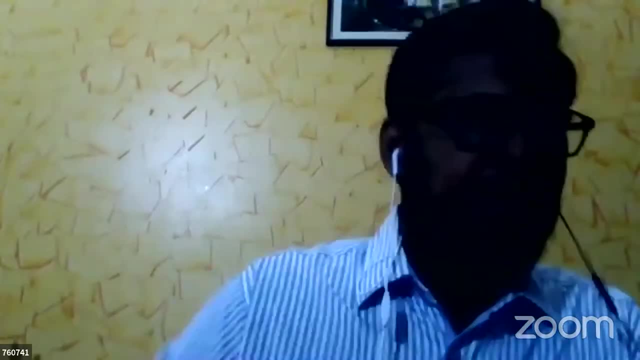 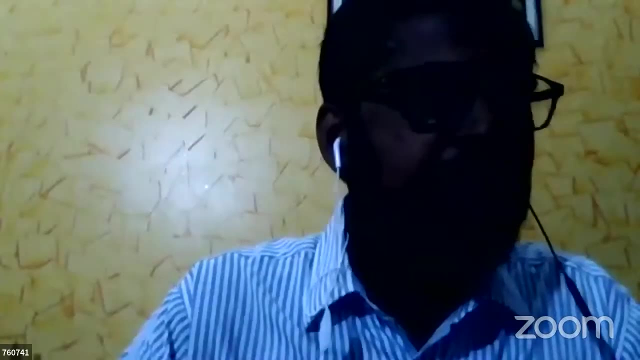 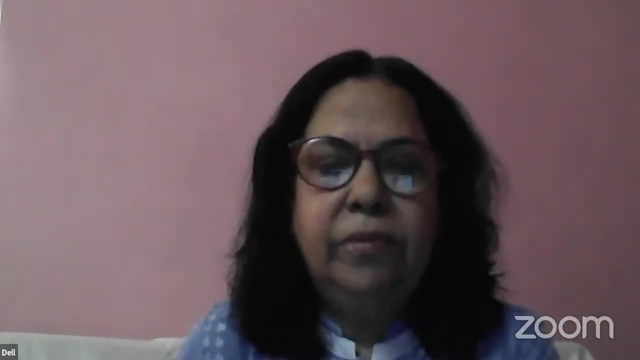 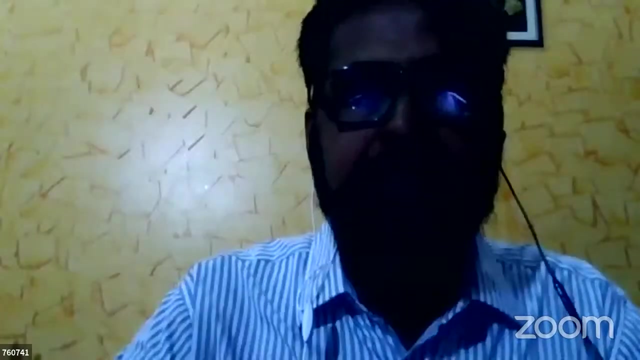 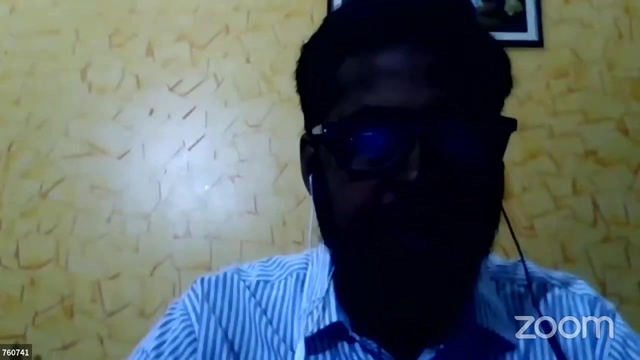 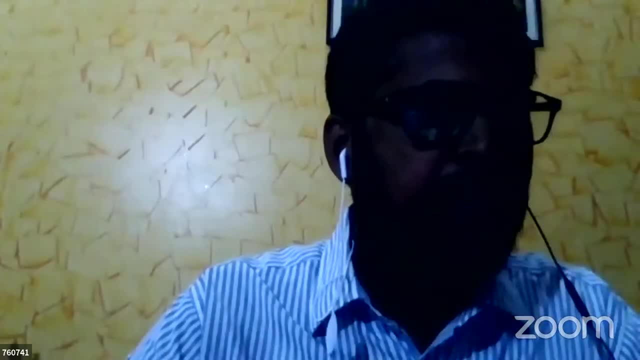 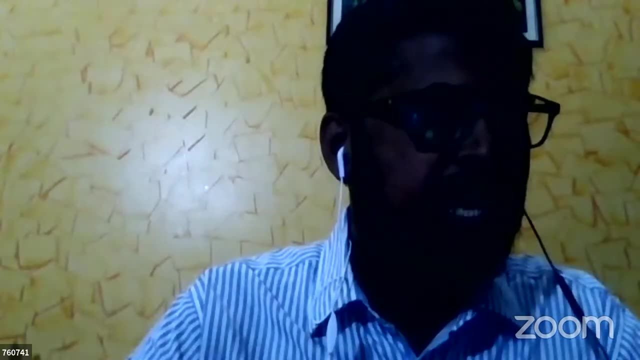 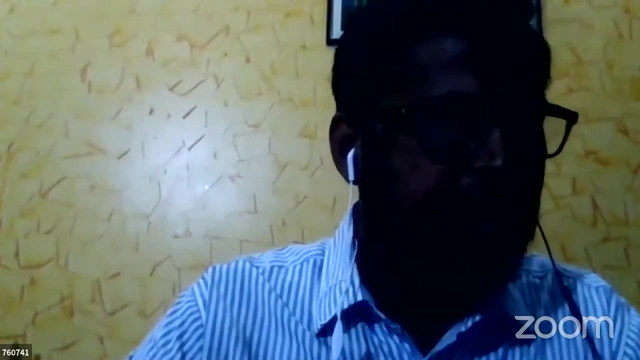 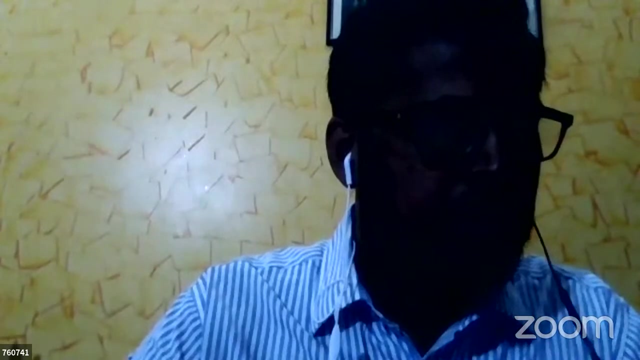 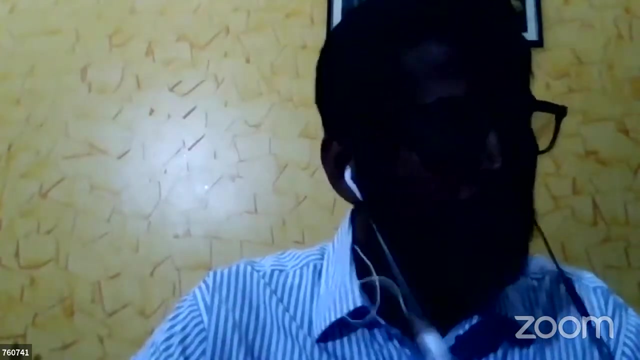 Dr Philip Muthulu is a principal hydrologist with more than 20 years of combined experience consulting and teaching in the area of flood mitigation, flood forecasting, climatic change, climatic change assessment and modeling. His notable previous roles include the position of Director of Flood Forecasting 2010-2013,. 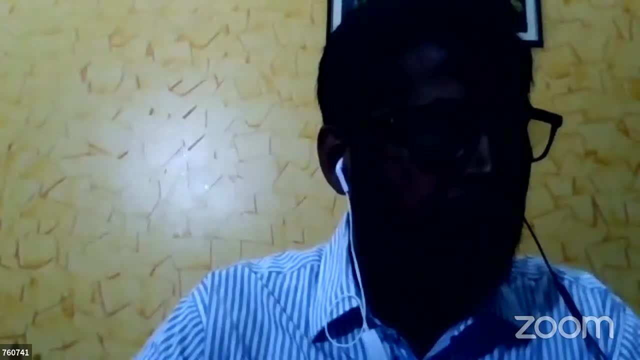 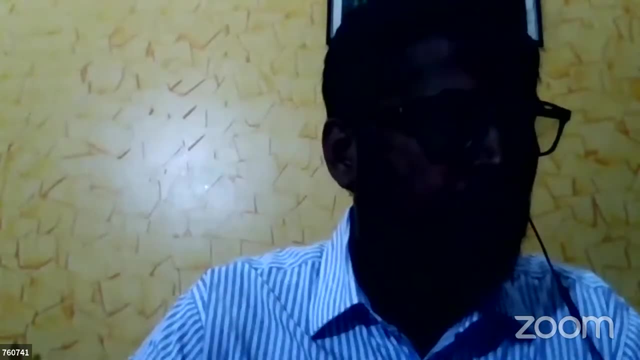 coordination and response for the province of Minnetonka, Canada. This role entailed providing technical guidance and leadership for the flood management of the area of flood mitigation. Dr Philip Muthulu is a principal hydrologist with more than 20 years of combined experience consulting and teaching in the area of flood mitigation. 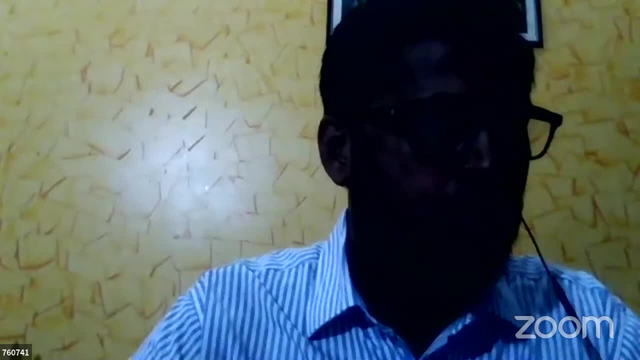 This role entailed providing technical guidance and leadership for the province of Minnetonka, Canada. This role entailed providing technical guidance and leadership for the province of Minnetonka, Canada, In land subdivision and flood protection zoning operation of flood control structures. 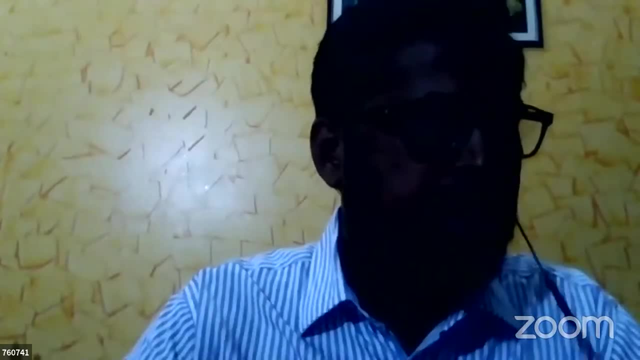 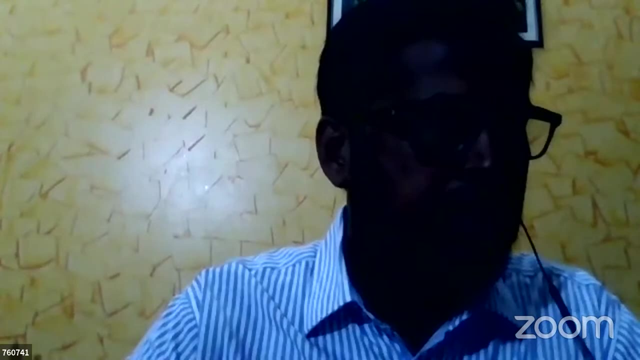 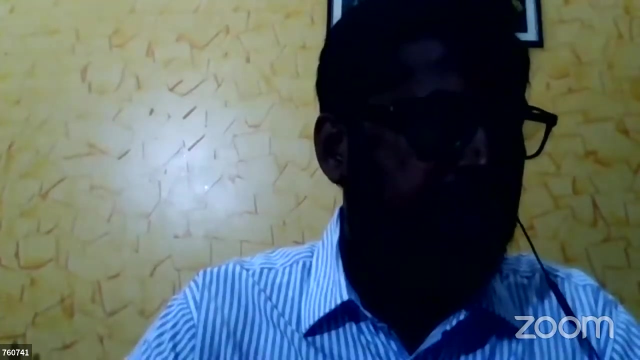 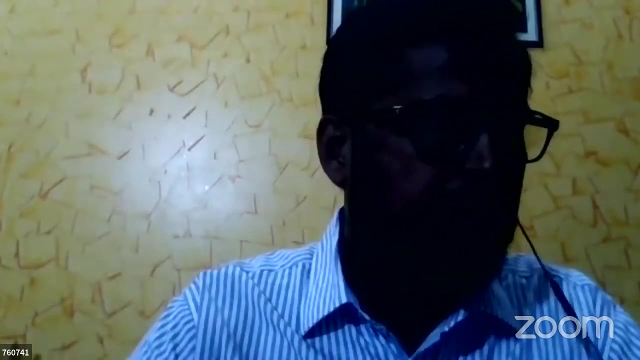 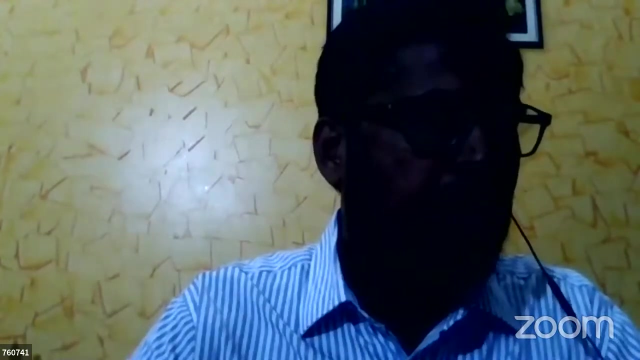 flood warning, flood response coordination and working within various state holders and assume optimum flood preparedness structure were in place at the right time in 2011.. Dr Philip led the province of Manitoba in preparedness and effective response to one of the worst floods in the province's history. 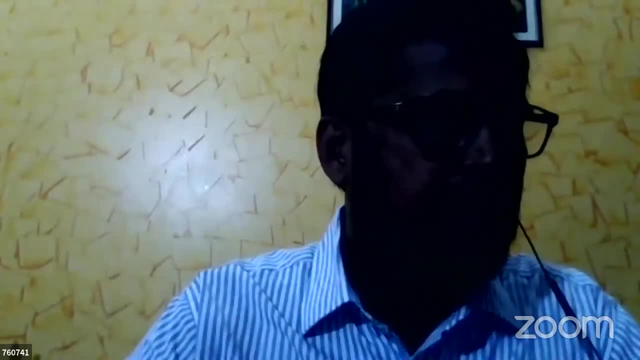 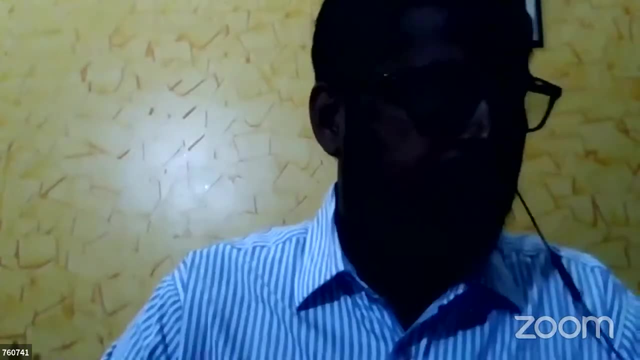 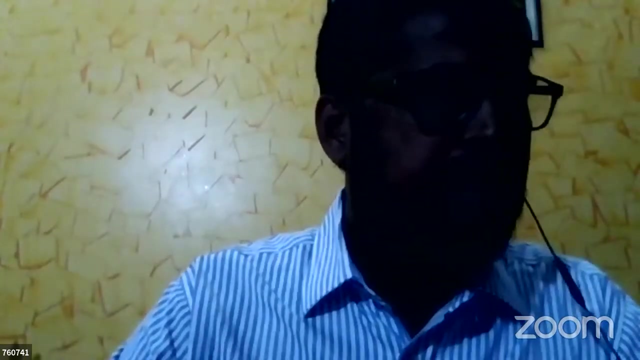 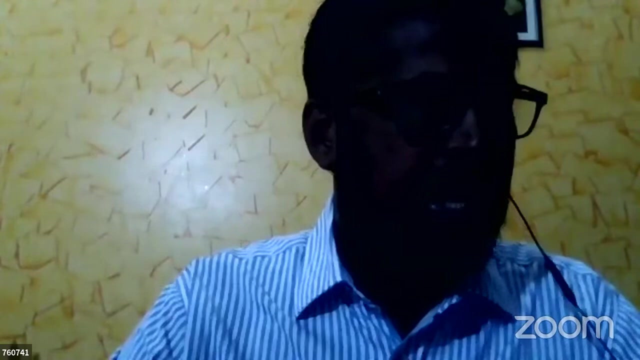 Dr Philip has been an active member of the Canadian Prairie Regional Adaptation Cooperative Programme, PRAC. Dr Philip has been an active member of the Canadian Prairie Regional Adaptation Cooperative Programme, PRAC, and has amended to improve the resilience of the prairie region to a changing climate through collaborative activities. 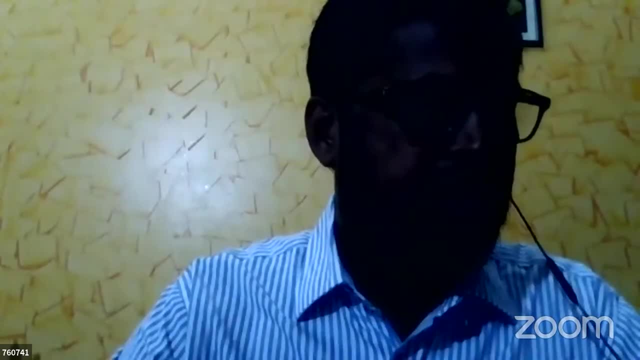 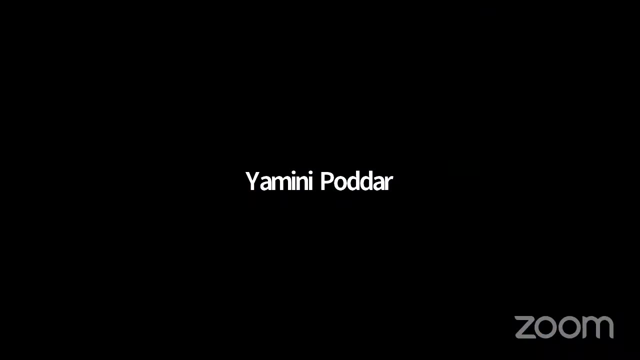 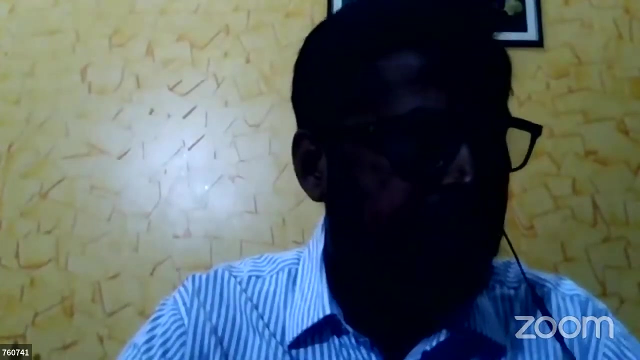 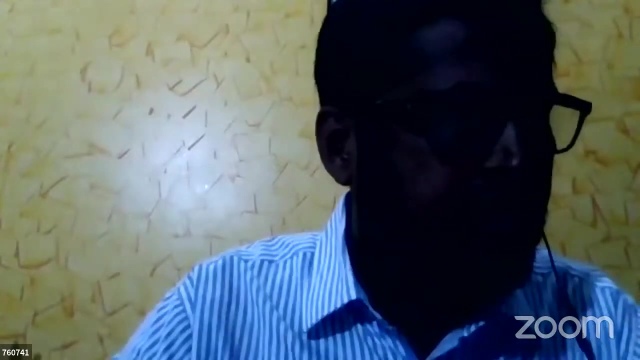 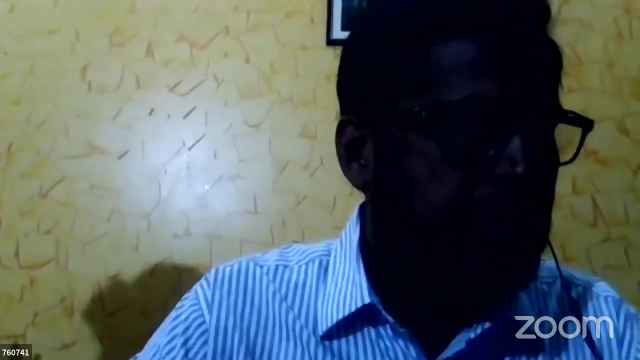 advancing adaptation and decision-making. In his previous role at the Stentec Council Consulting, Philip conducted several stormwater design including stormwater design studies for different municipalities, including the city of Calgary. He has also contributed to several major flood-related projects in Canada. 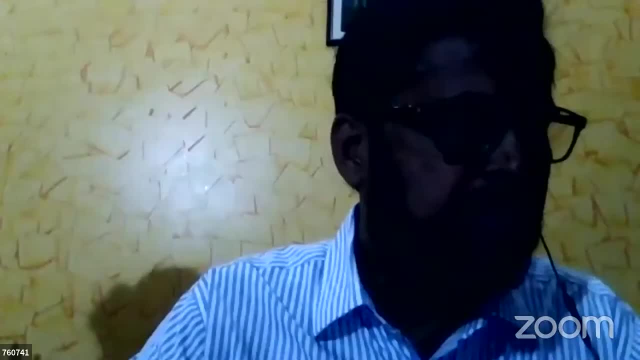 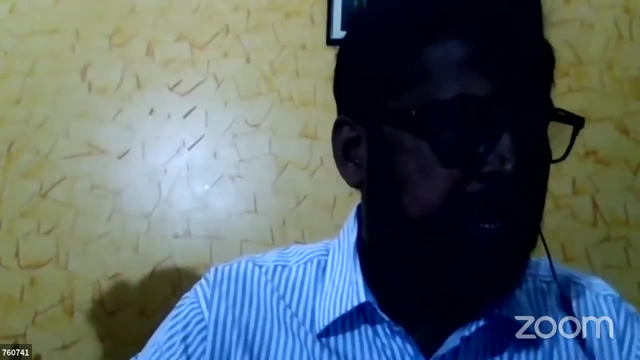 Dr Philip has recently completed a study on modeling flood sensitivity to climate change. Dr Philip has recently completed a study on modeling flood sensitivity to climate change. In his previous role at the Stentec Council Consulting, he has implemented cidade-level water management in a medium-sized watershed. 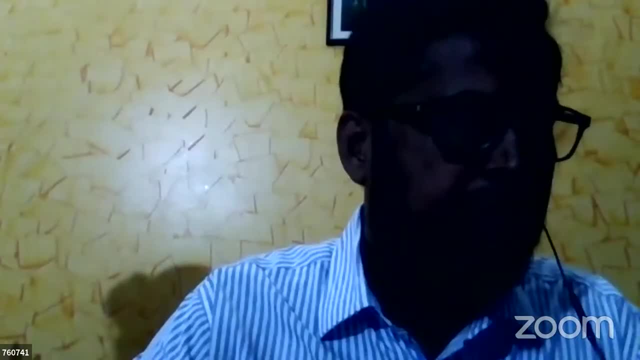 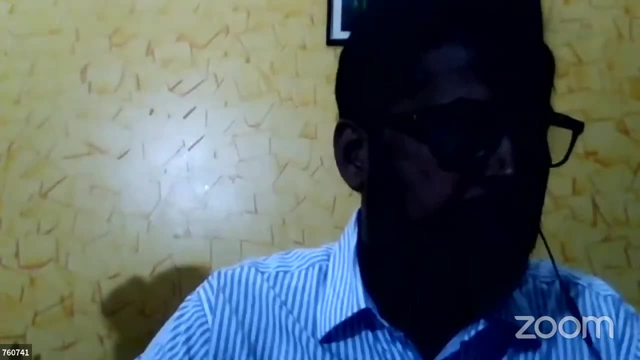 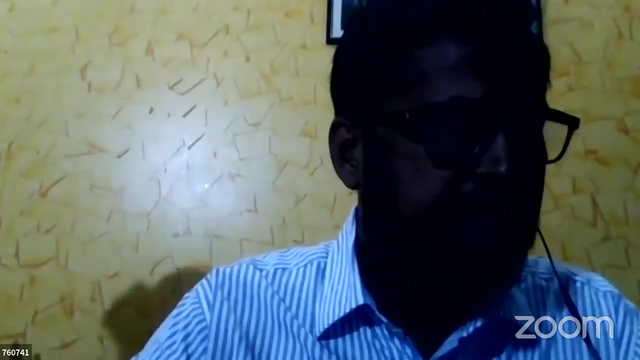 in a medium-sized watershed, based on the Upper Red Deer Basin. He has been conducting research in flood stimulation for a changing climate for the Upper Elbow River Basin. based on the Upper Red Deer Basin. He has been conducting research in flood Simpson for a changing climate for the Upper Elbow River Basin. 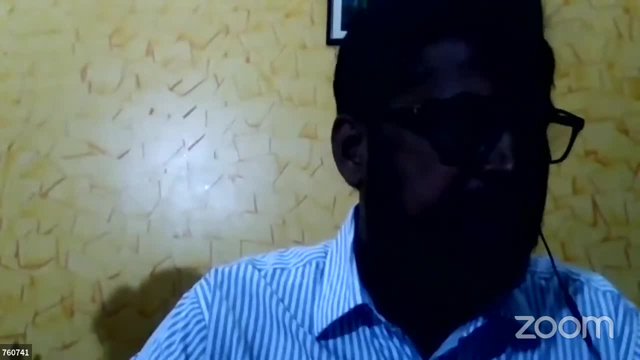 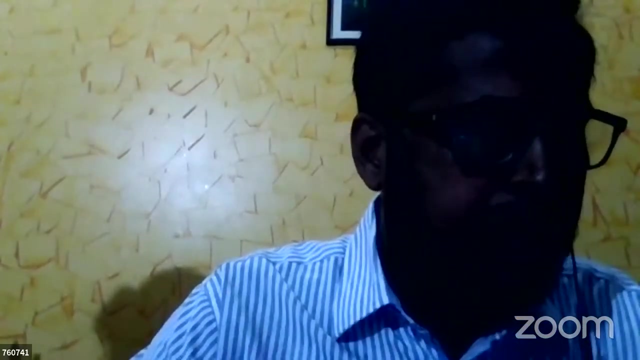 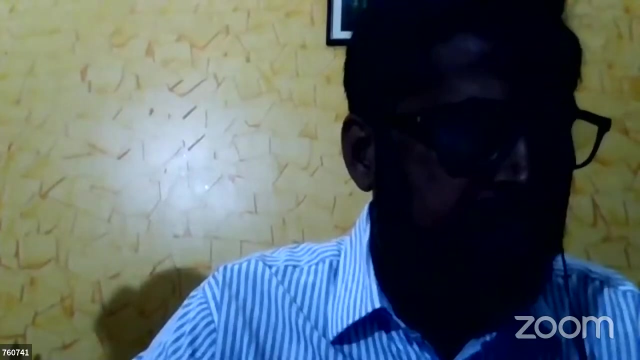 under sponsorship of Aquaclimб EnviroSolution Ltd. member of National Disaster Mitigation Program- NDMP technical working group on flood mapping, whose primary function is to support the implementation of the National Disaster Mitigation Program NDMP and has the mandate to develop national guidelines and best practices. 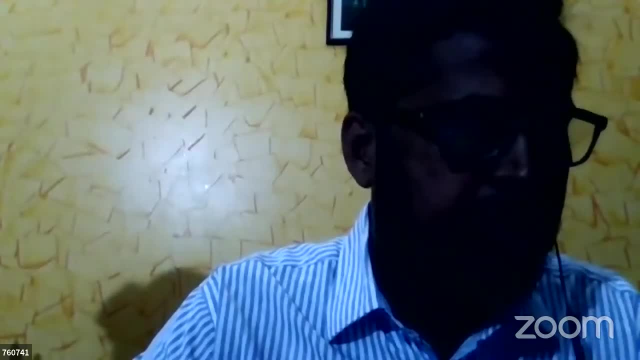 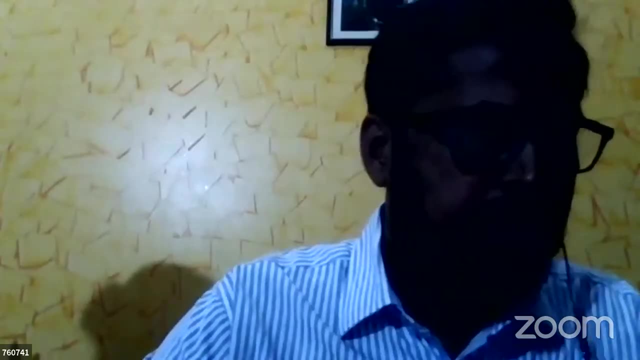 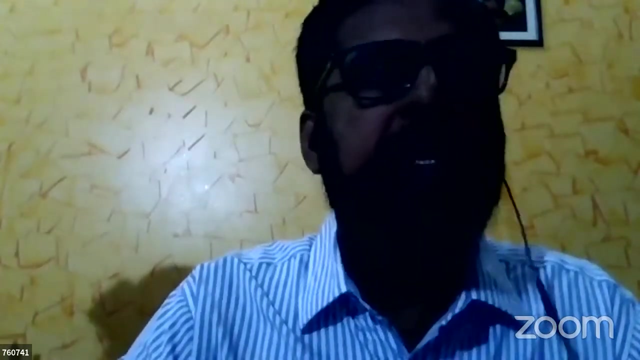 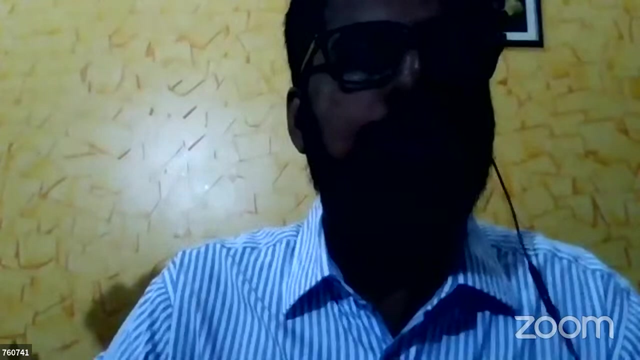 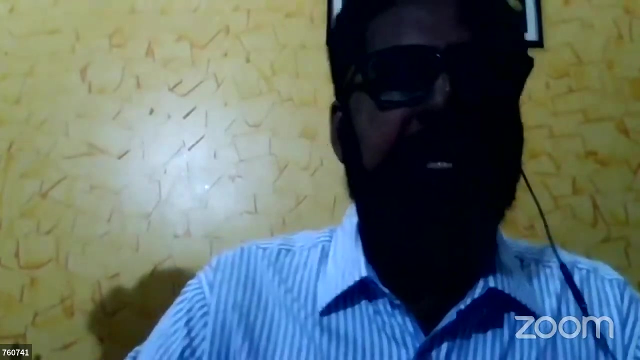 to meet the national requirements for flood risk, for flood risk assessment and flood mapping and monitoring. On my own behalf and behalf of entire geography department, I welcome Sir Dr Philip Muthulu in our midst this morning, and now I'll request him to tell something about the forecasting. 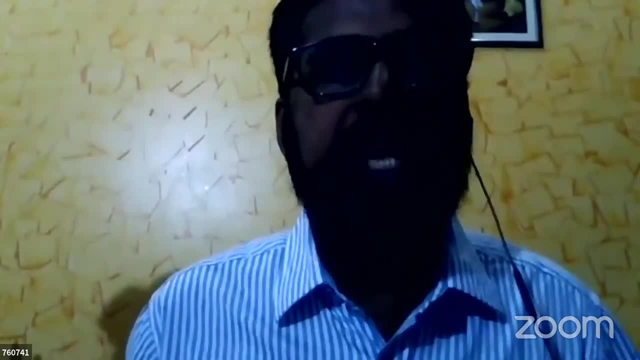 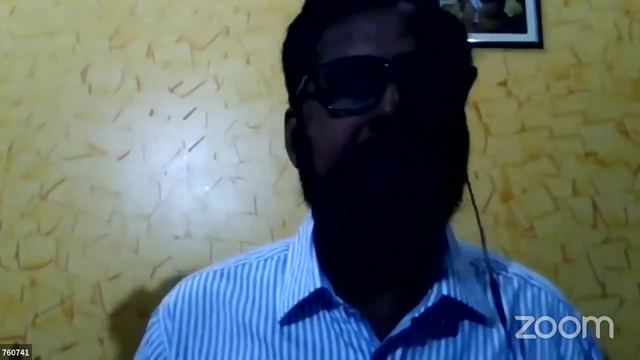 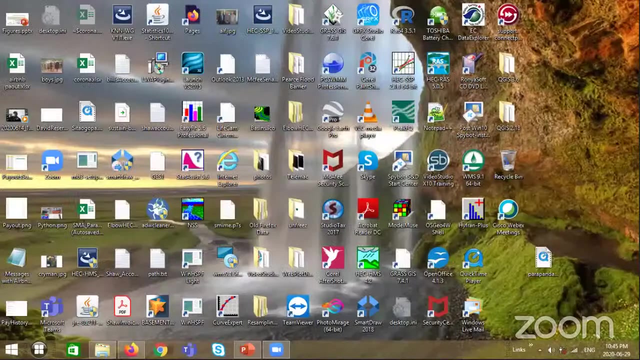 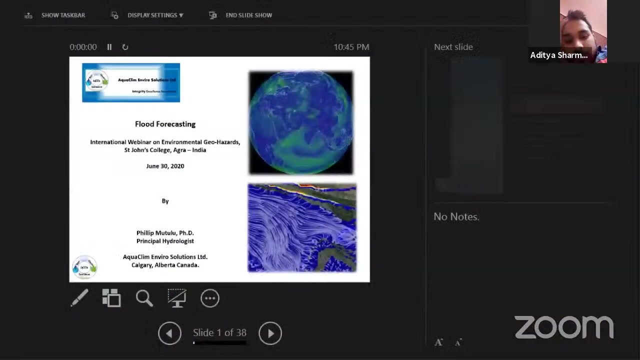 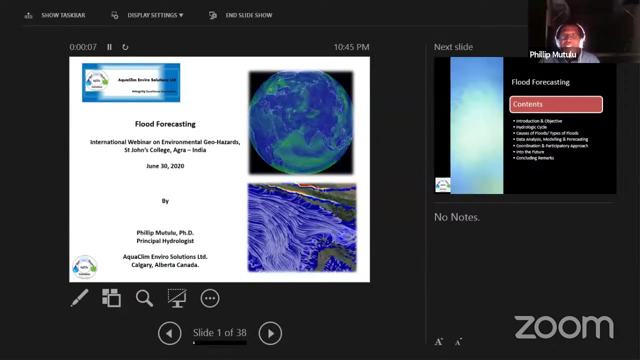 of flood to save lives and to save public property in the same earth. Thank you very much. Thank you, sir. Thank you, sir. Thank you Good morning, good evening, good night. Thank you very much for this opportunity. It was again. 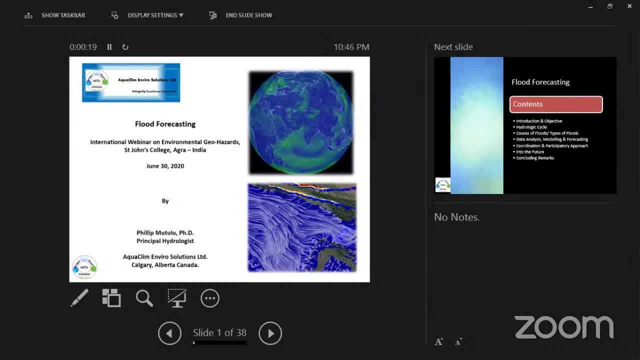 Good morning sir. Good morning sir. good morning, Good morning sir. Thank you for the opportunity to talk to you once again. this is the second time that making a presentation and I counted a privilege and an honor to share my thoughts on flood forecasting. 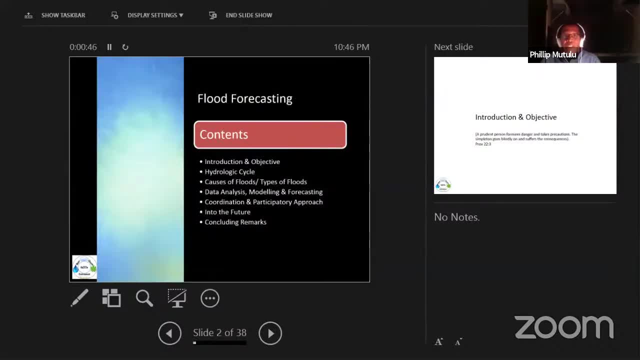 So today we shall divide our presentation into seven components. The first one, I will cover an introduction and provide an objective of the presentation, Then I'll talk briefly on hydrologic cycle, then the causes of floods and types of floods, then spend some time on data analysis. 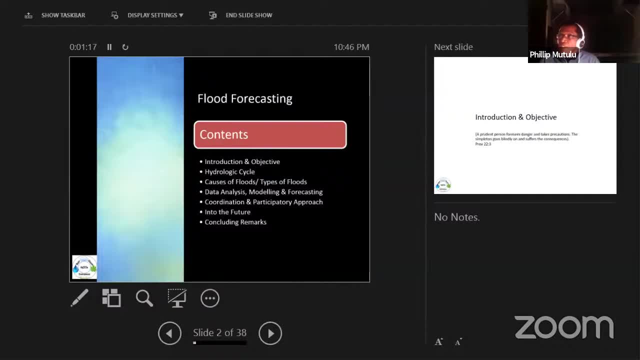 modeling and forecasting, then coordination and participatory approach and some future trends, And then I'll conclude. You bear with me because I'm going to be repeating some of the slides that I showed last time, though there will not be many, but I think they will help us in some sections. 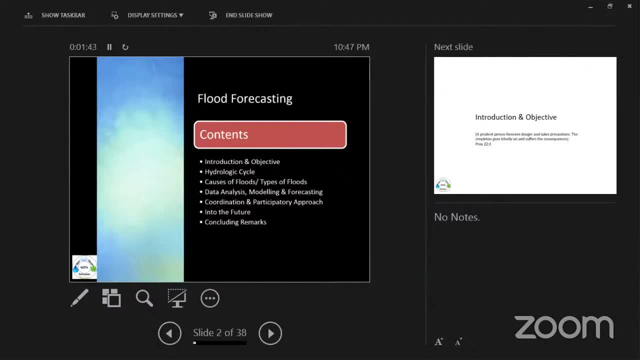 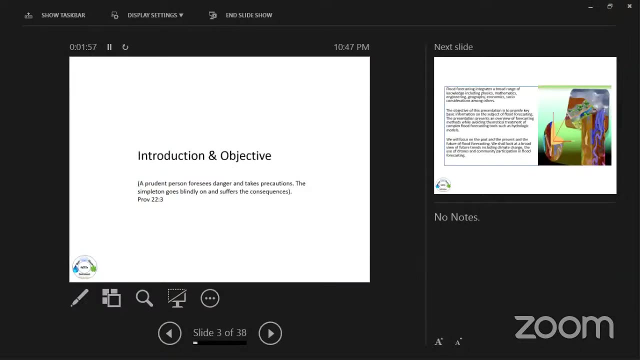 to clarify their presentation. Hello, Yes, sir. Yes, I will start with a quote from the scriptures. We say: a prudent person foresees danger and takes precautions. The simpleton goes blindly on and suffers the consequences. Proverbs, chapter 22,, verse three. 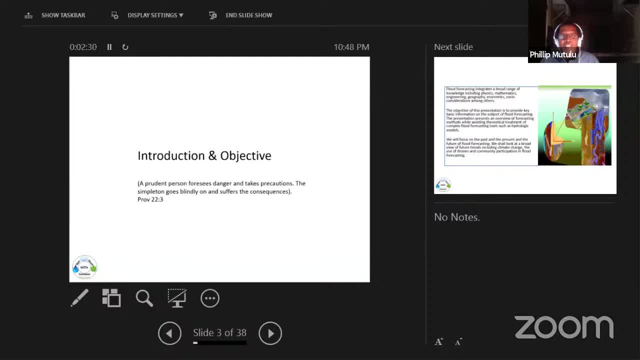 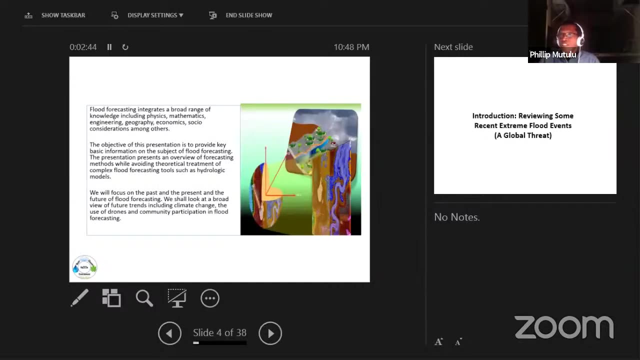 It's, in that, a challenge to a forecaster. A forecaster is supposed to foresee the danger with the knowledge that has been provided to him by the almighty. So flood forecasting integrates a broad range of knowledge, including physics, mathematics, engineering, geography. 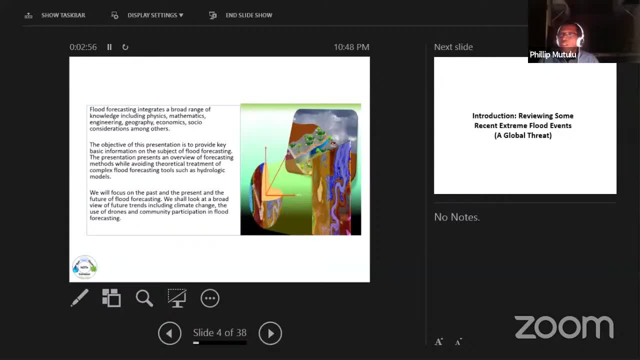 economics, social considerations, among others. So flood forecasting integrates a broad range of knowledge including physics, mathematics, engineering, geography, economics, social considerations, among others. So flood forecasting integrates a broad range of knowledge including physics, mathematics, engineering, geography, economy and social conditions. 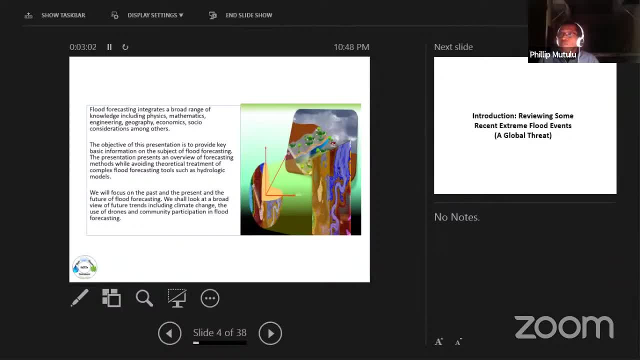 The objective of this presentation is to provide key basic information on the subject of flood forecasting. The presentation presents an overview of forecasting methods while avoiding theoretical treatment of flood forecasting tools such as hydrological models- So I'll try to avoid it- or the mathematical implications. 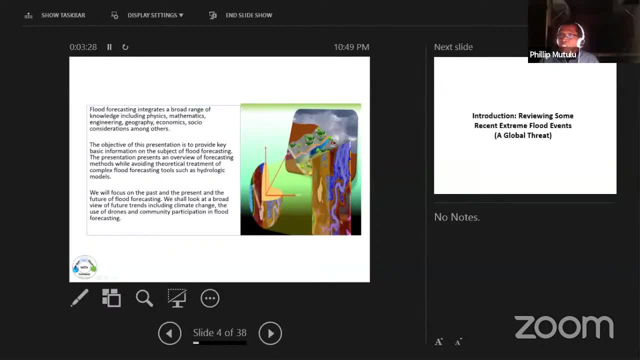 so I don't think they would exist. help us today, and there's not much time for that. we will focus on the past and the present and future of flood forecasting and also look at a broad view of future. trends include including climate change, the use of drones and community participation. participation in flood. 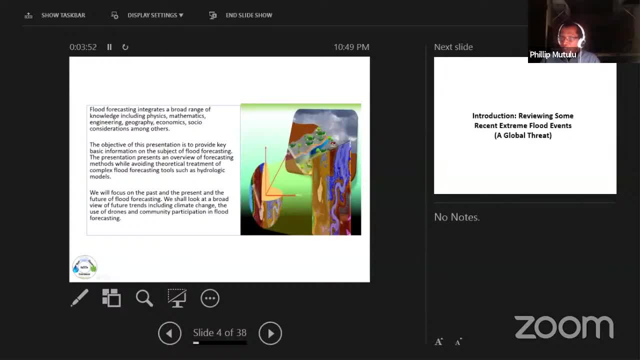 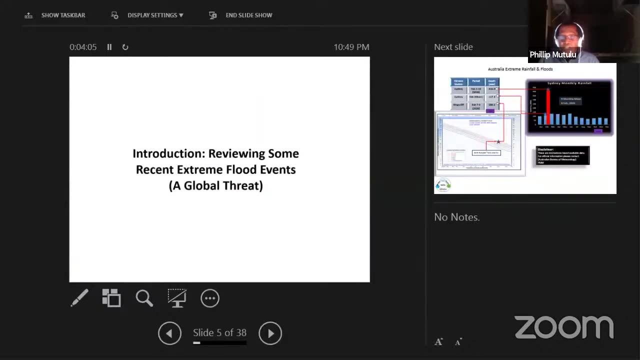 forecasting. so you like, you'll excuse me. once again i'll be talking about climate change, but today in the context of uh flood forecasting. so as an introduction, i'm gonna just run quickly through some of the recent uh extreme flood events. uh, probably for for you people in india, of course, this is a frequent threat and so i'll just provide. 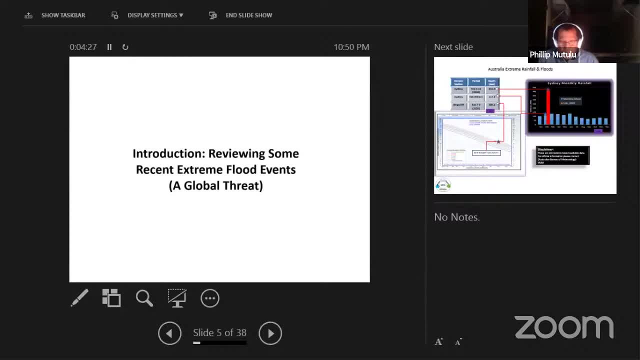 a brief overview of what's going on in north america, just kind of to drive a conviction in your hearts as we discuss this topic today and see yourself as a person who needs to have a part to play in preparedness. it's a global threat. uh, almost every week we are hearing uh. 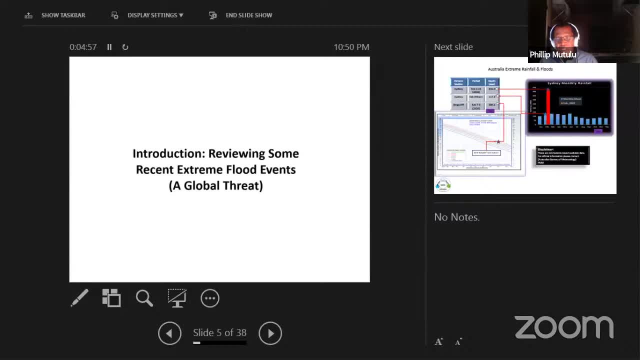 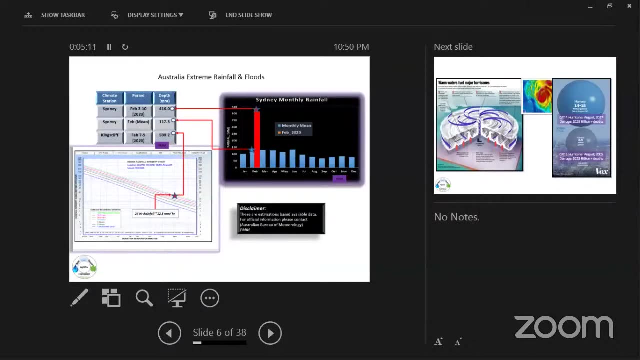 flood episodes and flood events happening across the globe and they seem to be more frequent and more extreme, like we discussed last time, potentially due to uh climate change. so one of the recent uh flooding happened in australia. it's a very recent um occurrence in memory and this happened in february, early this year. 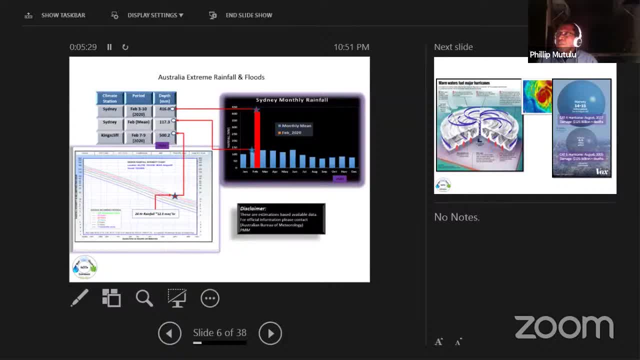 uh what you see. on the right hand side there is a graph just to show the extremity of the event. you can see the month of february actually received more than half, actually more than twice, the normal rain that they get during that time. these patterns are repeated over and over again. 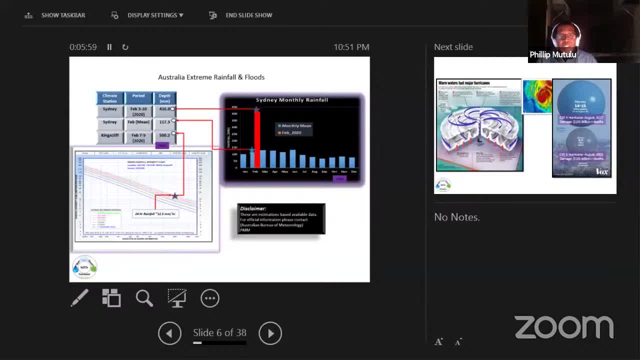 in diverse places where, in a day, you get a total rainfall of of six months, three months, and so they are. they are pretty extreme, and this is just an example from australia, because it's fresh in our memories: uh, what happened that time? we had nearly 500 millimeters in some places in australia. 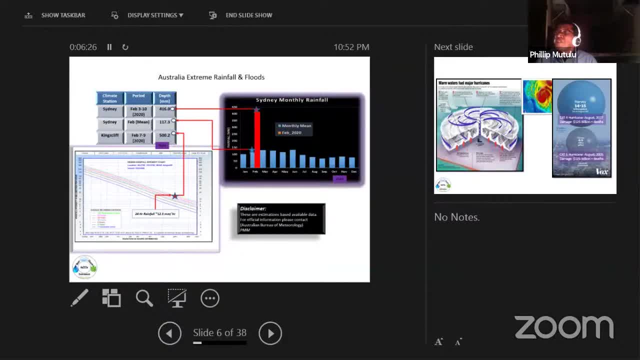 while actually the month of february- of february is- is less than 150 millimeters um. the chart there that i'm showing there is just to show that the return period of that event for 24 duration was somewhere between 50 years and 100 years. 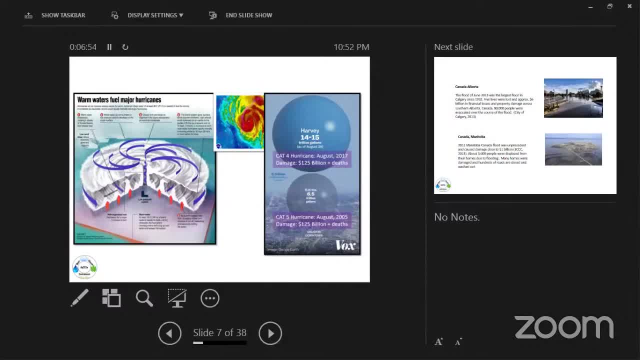 so the other recent, uh um example from north america was harvey. i particularly wanted just to talk about this a little bit because it was very extreme, with total damages of 125 billion dollars plus several deaths, and harvey actually had a lot of water. you can imagine that. 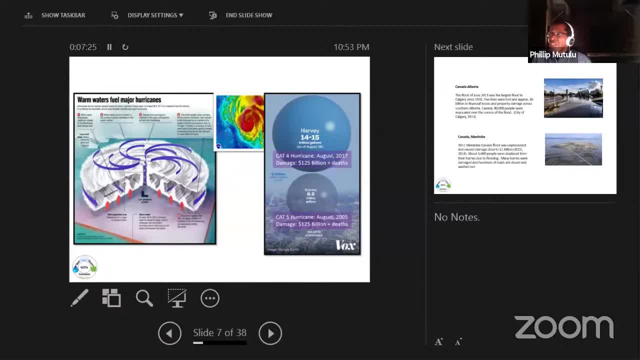 There were 14 to 15 trillions of gallons of water that came out of that hurricane. It was Category 4.. Compared to Katrina, which caused a lot of deaths earlier on in 2005,, have it happened in 2017,, by the way, for those that may have forgotten, 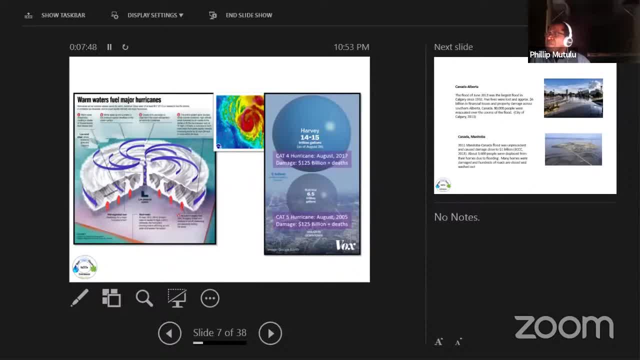 Katrina happened in 2005.. And, incidentally, although it caused more deaths, actually the amount of water produced by that hurricane was 6.5 trillion gallons. So that was also quite huge, but not as much as Harvey. Katrina was Category 5 and Harvey was Category 4.. 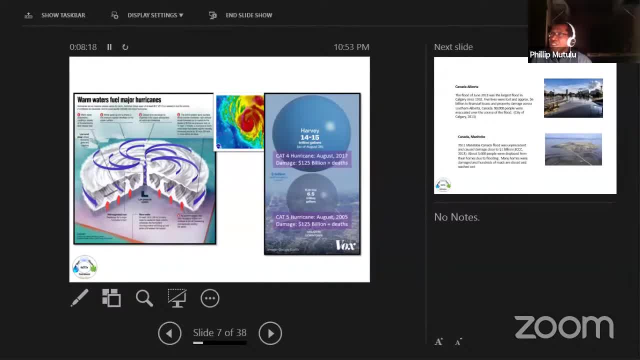 So these are recent systems, And in India, of course, you have to deal with tropical cyclones. By the way, in North America they call them hurricanes, In India they call them tropical cyclones. I think in China they are typhoons And in Australia they are willy-willy. So it depends on where you come from. 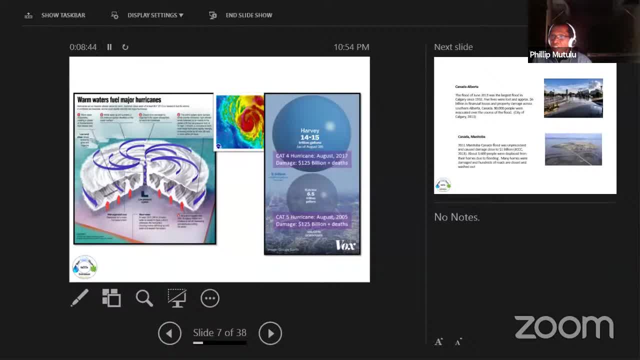 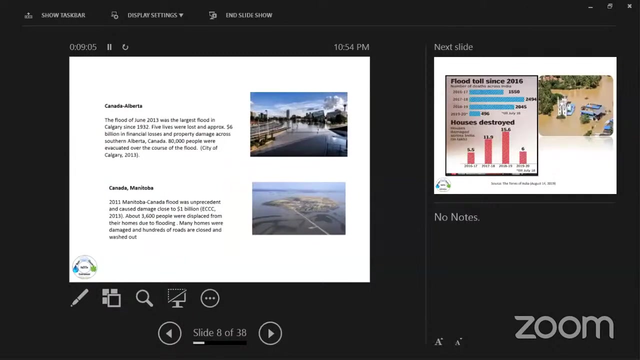 On the left-hand side. I just provided a three-dimensional figure of what a hurricane looks like. You can look at the details much later. It's a whole representation of a thermodynamic system like an engine of a car, And then these are examples that I provided last time that I was making a presentation close to home here in Canada. 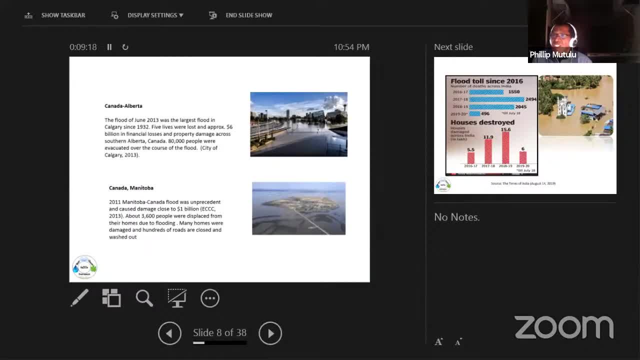 And where we have also seen extreme flood events: in Mandova Province in 2013.. And then where I used to work as a flood forecaster in 2011 in Manitoba, where we saw damages due to flooding of close to 1 billion. 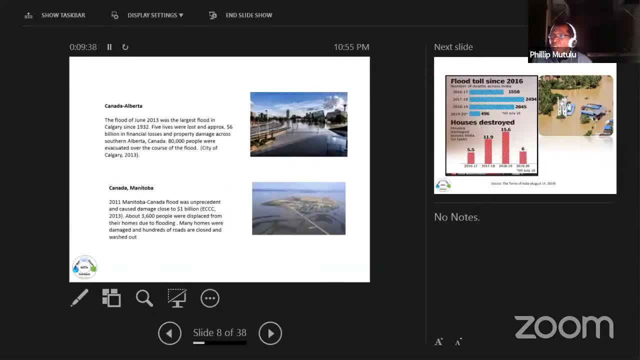 And about three thousand and six people were displaced from their homes and up to today actually, they are still being settled. They are not completely taken from their homes, completely recovered from that flood. So these flooding episodes can be very devastating and the effect can last for a long time. in many ways, 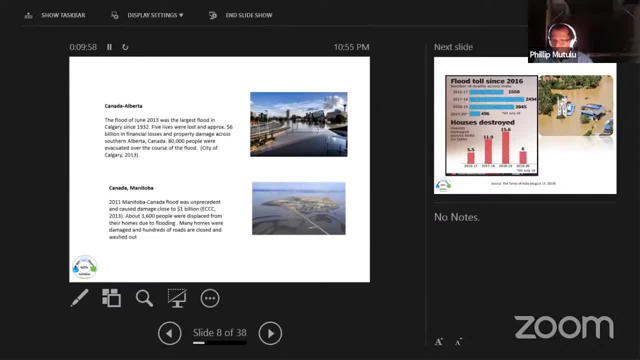 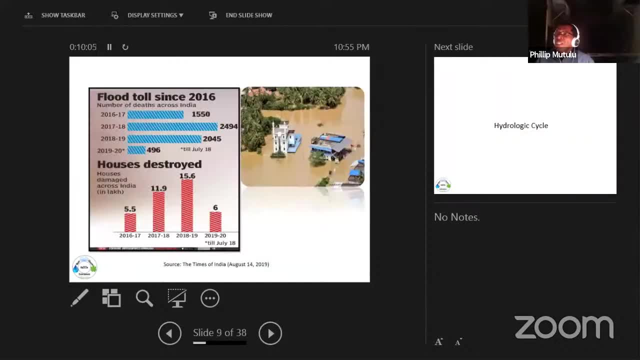 And the effects can be physical, infrastructural, can be emotional, different types of effects. And then that's a chart again I showed for India that I pulled out of the Times of India where they made a summary of some of the recent flood damages. 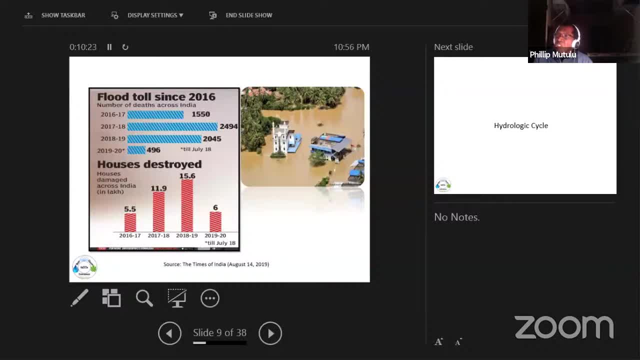 You can see that quite a number of casualties, especially in 2017 and 18,. they were 2,494. And we have a responsibility to make sure that we are prepared and that our forecasting systems are working well So that whoever needs to be evacuated. 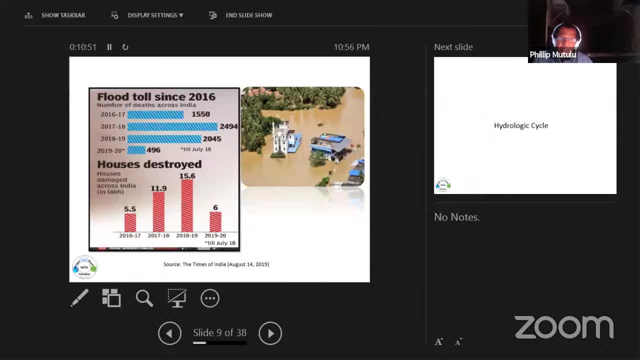 whoever needs to move to a different place or whichever place. flood control structures need to be operated. they need to be operated in timely manner, And these operations and evacuations can only happen, These evacuations can only happen, if we have proper forecasting techniques. 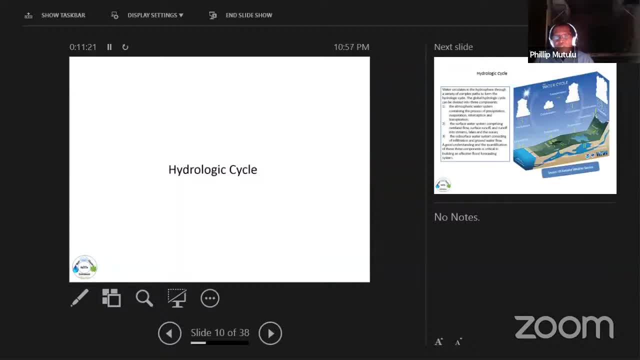 And before I go into more details, I want to recap hydrologic cycle, which is a very well known cycle to most of you, especially coming from geography background, because this is a basic knowledge of the water cycle and provides the knowledge that we need to have. 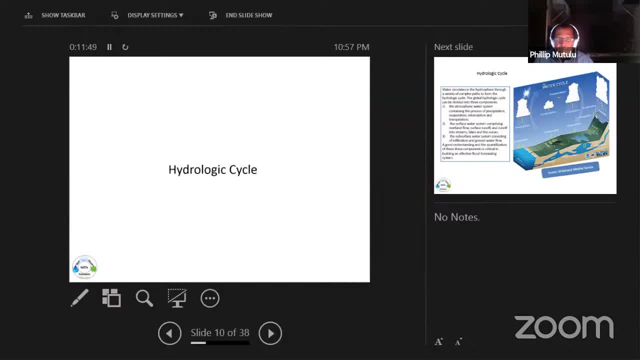 to be able to build forecasting tools and to be able to apply them. So all the building starts from an understanding of hydrologic cycle, And it could be a global hydrologic cycle or just a cycle that is locally based in a local catchment or watershed. 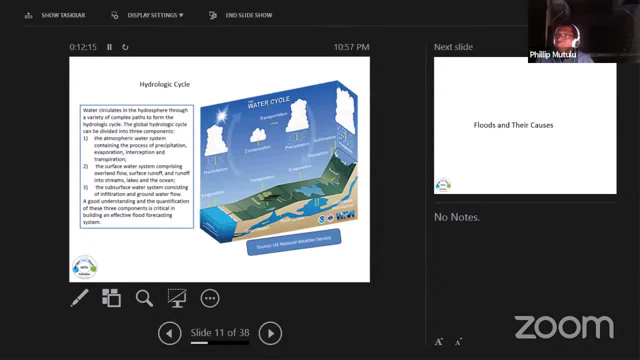 That's some good picture there of a water cycle And, as a summary, water circulates in the hydrosphere through a variety of complex paths to form the hydrologic cycle. The global cycle can be divided into three components. The first one is the atmospheric water system. 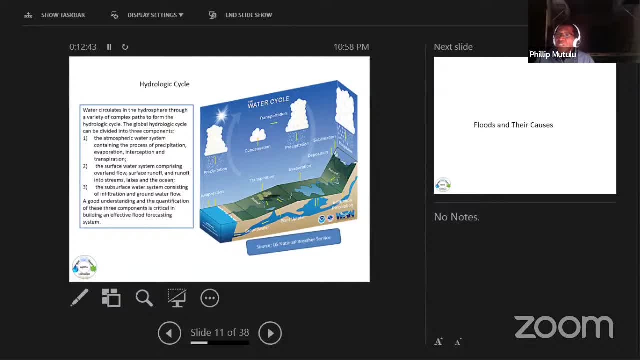 which constitutes the process of precipitation or rainfall, evaporation, interception and transpiration. The second component is the surface water system, comprising overland flow, surface runoff and runoff into streams, lakes and the ocean, And the third one is the subsurface water system. 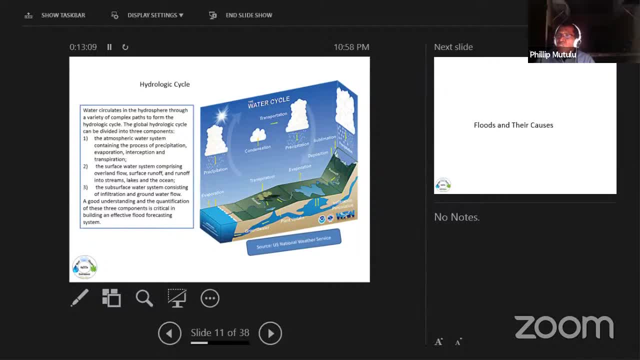 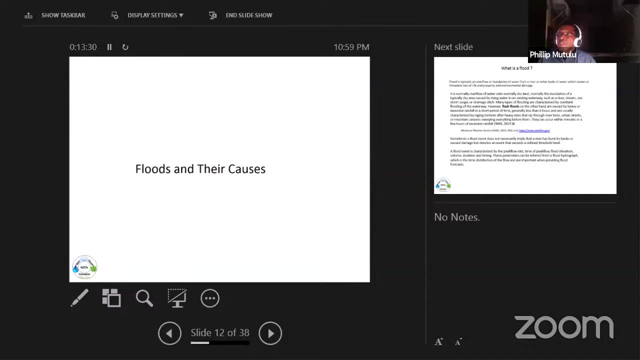 consisting of infiltration and groundwater flow and seepage as well, And a good understanding and quantification of these three components is very critical in building an effective flood forecasting system. So a recap again of something that we talked last time. I just go through this quickly. What causes floods And we saw that first. what is a flood? Typically it's an overflow or inundation of water from a river or other body of water which causes or threatens loss of life and property and environmental damage. It is normally an overflow of water onto normally dry land. Usually the inundation of a typically dry area, caused by rising water in an existing waterway, such as a river, Streams, sea storm surges or drainage ditch. Many of these floodings are characterized by overbound flooding or off the waterway. 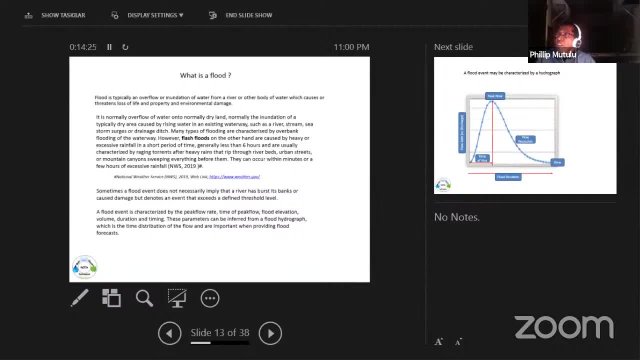 However, flood floods, on the other hand, are caused by heavy, excessive rainfall in a short period of time, Generally less than six hours, and are usually characterized by raging torrents after heavy rains that rip through riverbeds, urban streets or mountain canons. 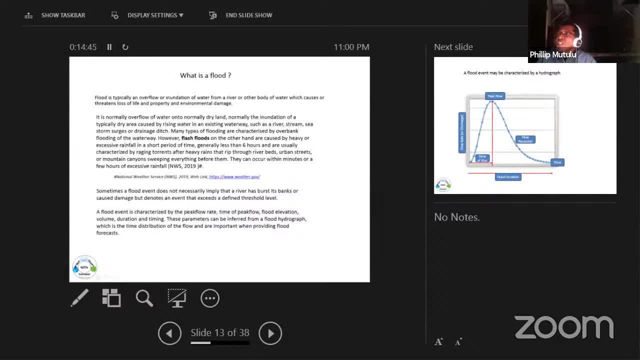 everything before them. They can occur within minutes or a few hours of excessive rainfall. Sometimes a flood event does not necessarily imply that a river has burst its banks or caused damage, but denotes an event that exceeds a defined threshold level. So probably an example in that line is sometimes, when you have elevated groundwater levels, that 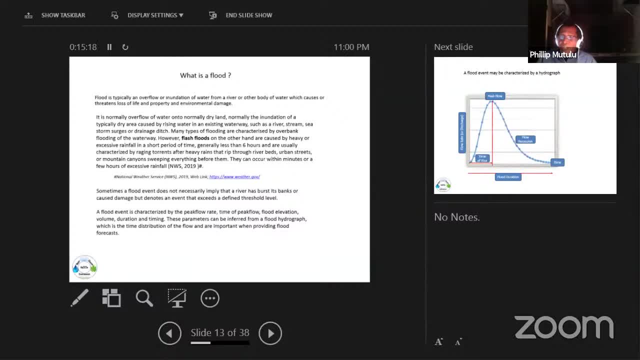 intersect with ground surface, you can actually have flooding in an area, and so this flooding is not necessarily coming from a river. Even now also, flash flooding also does not emanate from a river channel, so it's good. it's important to understand that flooding does not necessarily have to emanate from a river system. It could also be a tide from a lake. 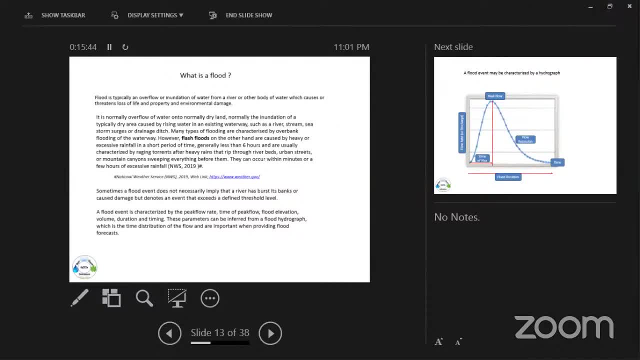 or from the ocean. In terms of flood forecasting, there are a few basic components that one needs to understand, because these components are the things that you provide to the consumer of a flood forecast in order that they can prevent guests or Denton, and also flood residents, from flooding. 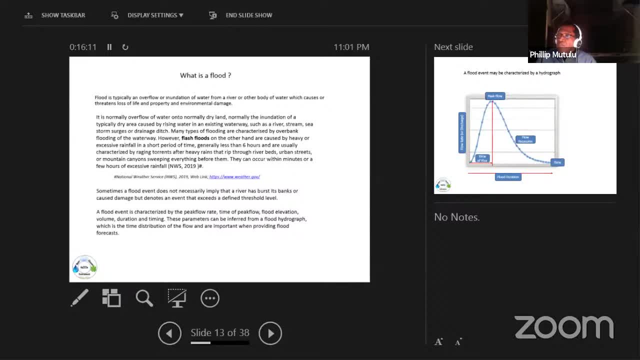 One of the first critical components for flood prediction is the time of it. The time of a flood is the time of the flood event, and it can vary depending on the water flow in the system. The time of a flood is the time of the flood event. 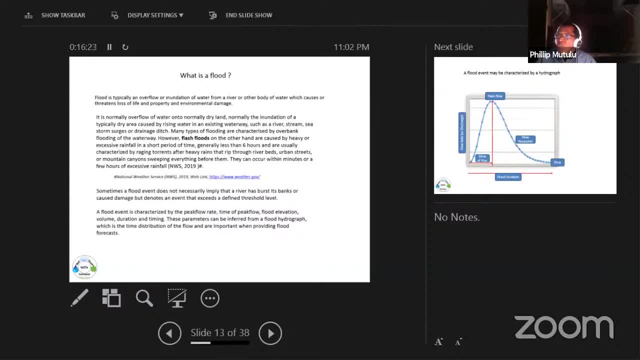 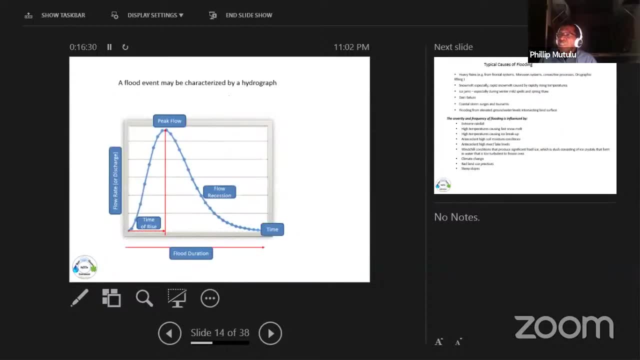 It is an even greater significance for a flood when we prepare adequately And therefore a flood event is characterized by the peak flow rate, time of peak flow, flood elevation, volume, duration and timing. These parameters can be inferred from a flood hydrograph, which is the time distribution of flow, and are important when providing flood focus. 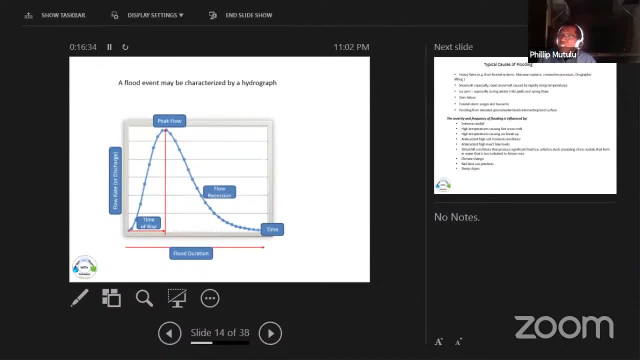 This a pictorial presentation of the above stage, Sweden. The example I have shown you is a photo of a small. Other ones are in the upper left, the first one in the upper left which shows the bottom line of the river. this is just a graph of time distribution and again it's the vertical axis, the flow rate, or 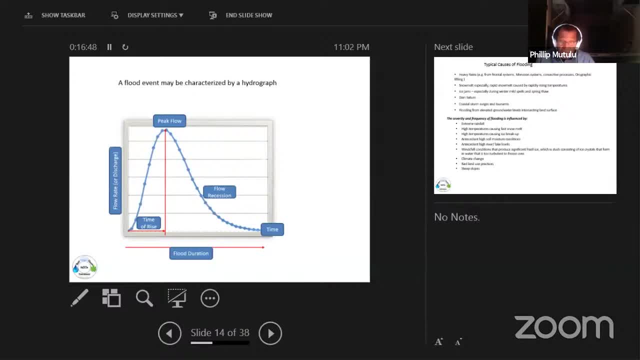 volume or water level, whatever parameter you're looking at, and one of the important thing is peak flow. we want to know the maximum volume that you're gonna get so that if we are preparing a reservoir to receive water or to release water, then we know how we are going to operate a reservoir. 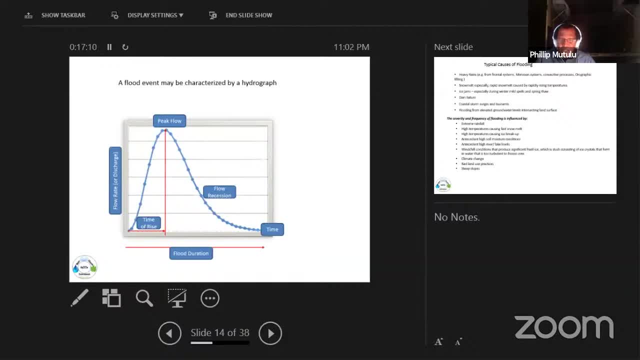 or a flood way, or if we know that the flooding is going to encroach a wide area in the flood plain and probably affect people, then we can evacuate people that are within the close to the flood zones. so the peak flow is very important in determining the maximum amount of flow and 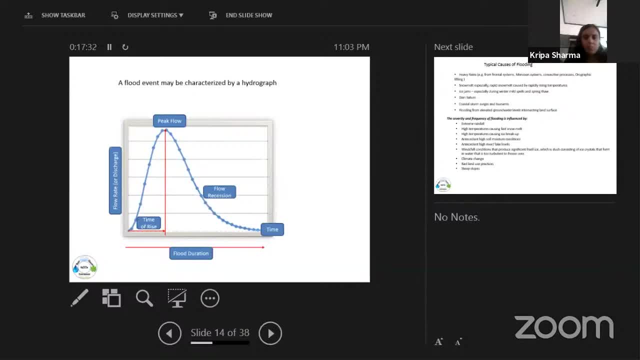 also the time of rise, that is, the the time between when the flood starts and the peak time, is very important in terms of timing so that you can provide the vacation. or the emergency manager should know this, so that they can know they have enough time to evacuate, or the operators of flood control systems. they 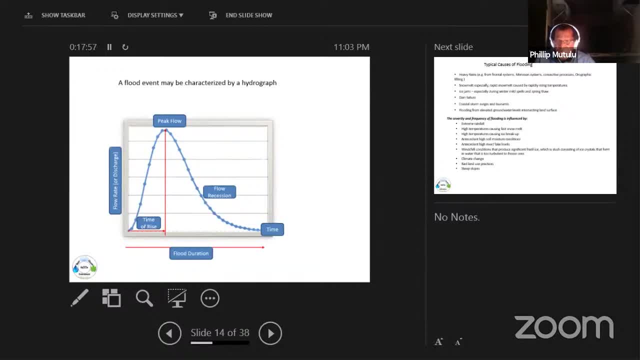 have enough time to operate their water flow water control structure so that they are not overwhelmed by flood when, when the it comes to the peak, the peak flow, and right there on the, on the bottom, there, on the horizontal axis, you also have the flood duration. we also want to. 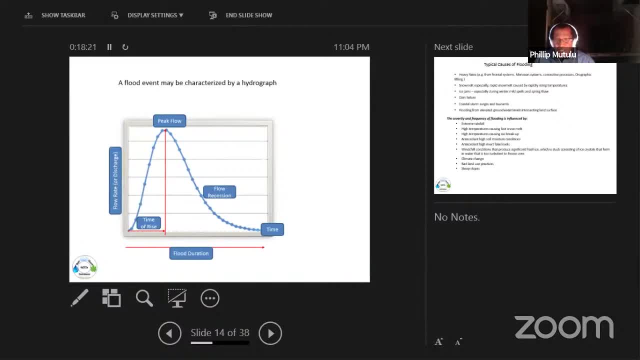 know how long this flood is going to last, uh, so that, um, we can have a good picture of how we are going to operate our flood control system that up, we have de acceleration set up. it should allow the flood, so we can also do, you know, major. 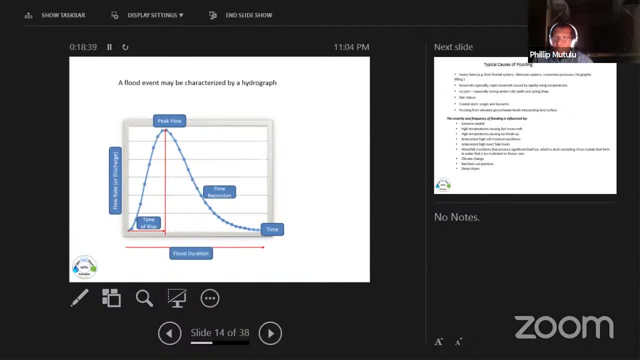 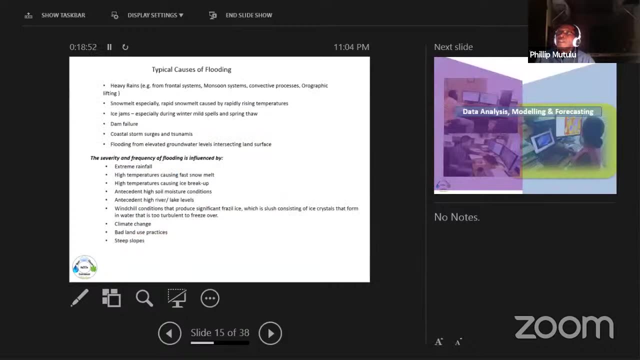 Ladner is familiar with the flow. if flood can go like, however you can see, here we have the flow, we can also do. you know, we can operate the flood meanwhile by альные um, so, um. so I think that's a kind of a recap, a repeat again, but I just want to focus on the second portion of 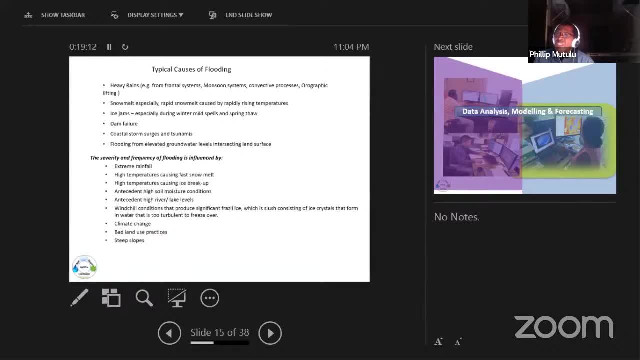 that slide. What causes severity of flooding? Because I think this is very important and these factors, actually they need to be taken into account by our flood models. They need to be able to take into account possibility of extreme rainfall temperature preceding, high soil moisture conditions and dissident high river. 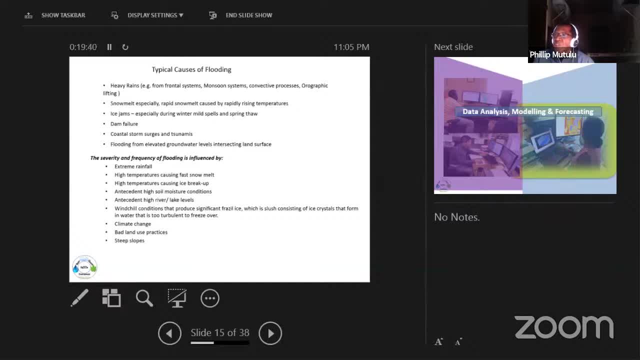 lake levels with chill conditions that produce fragile ice, like in Canada. Maybe you may not have that problem in India, but probably near the mountains you could have this problem of fragile ice. Then, of course, our forecasting tool should also be able to factor in climate change. 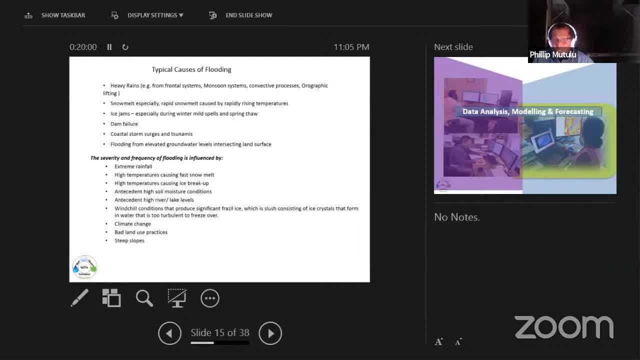 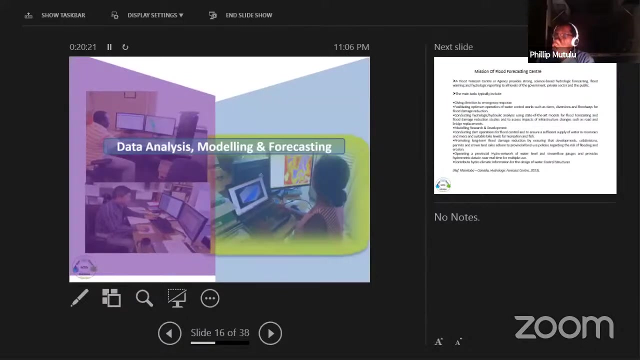 And then land use practices needs also to be accounted for, and land slopes as well. How these characteristics, all these patterns are formed, or the way they are, will encourage or discourage extreme flooding episodes. So that was kind of introductory. Now I want to go and just talk a little bit about 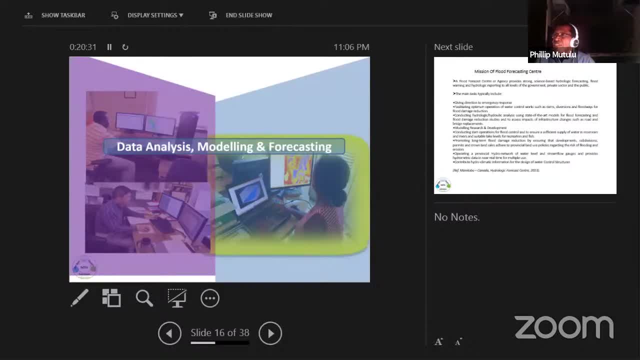 data analysis, modeling and forecasting. Sometimes the difference between data analysis and modeling may not be very distinct, because modeling is a kind of analysis but it's a specialized type of analysis. So analysis is more general, but modeling is a specific component of data analysis. 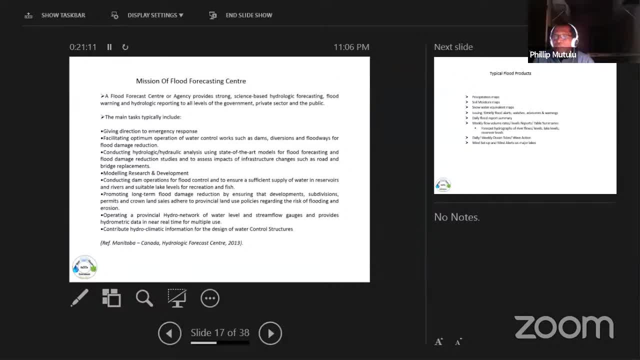 So we are now into the realm of forecasting, but I wanted to kind of reiterate what the mission of FLAD Forecasting Center is. I have looked at the Indian mission and you know what their centers are focused on. Some of these are captured in this mission, which is cut from Canada. 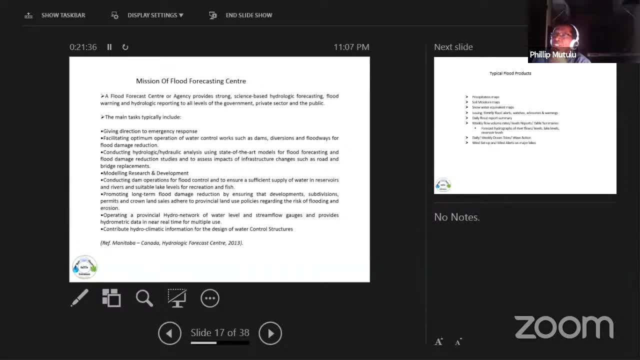 And typically the FLAD Forecast Center provides strong, science-based hydrologic forecasting, flood warning and hydrologic reporting to all levels of the government, private sector and public. Actually, at this point I need to mention that in some places, forecasting for FLAD is done together in the weather forecasting agencies as well. 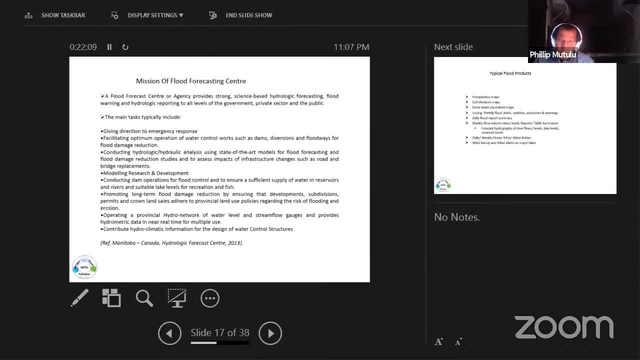 In Canada they seem to be separated. So our FLAD Forecasting Center is here separate entities, although they link up with the meteorological centers who provide data to them. But if you look at a place like Australia, actually you have weather bureau which actually houses the FLAD Forecasting or Hydrologic Forecasting. 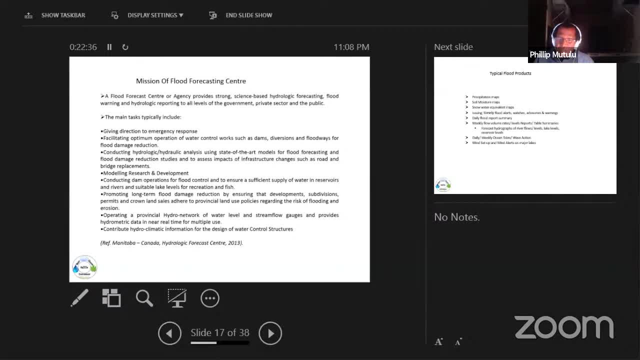 So this arrangement varies from one nation or state to the other. I think similarly in India as well. So the main task of a FLAD Forecasting Center should include the following: Giving direction to emergency response. facilitating optimum operation of water control works. 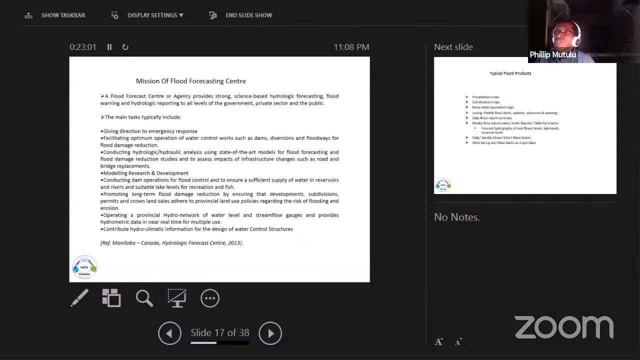 such as dams, diversions and flood waste for FLAD damage reduction. Conducting hydrologic hydraulic analysis using state of the earth models for FLAD forecasting and FLAD damage reduction Studies, and to assess impacts of infrastructure changes such as road. 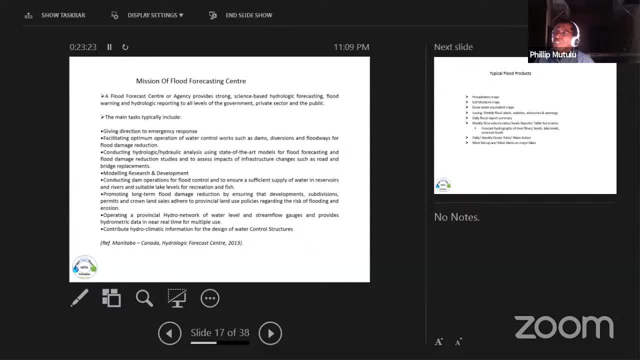 and bridge replacement, Modeling, research and development, Conducting dam operations for FLAD control and to ensure a sufficient supply of water in reservoirs and rivers and suitable lake levels for recreation and fish. Promoting long-term FLAD damage reduction by ensuring that developments and subdivisions, permits and crown land sales are there to provincial. 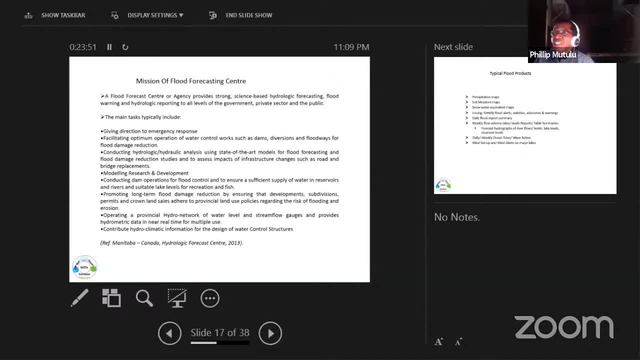 or state land use policies regarding the risk of flooding and erosion. Operating a provincial hydro network or state hydro network of water level and storm gauges and provides hydrometric data in near real time for multiple use. Contribute hydroclimatic information for the design of water control structure. 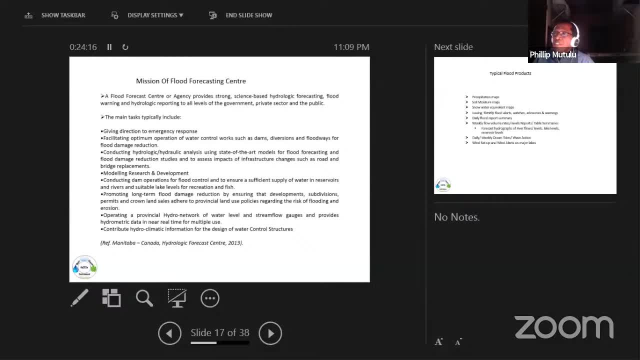 So it's quite an integrated responsibility. So it's quite an integrated responsibility for a forecasting center. they don't just provide uh focus, but they provide customized information to different consumers. of course, all these consumers, this data is a form of a flood, but it's a different process type of flood, like you're not going to provide the same data to an engineer. 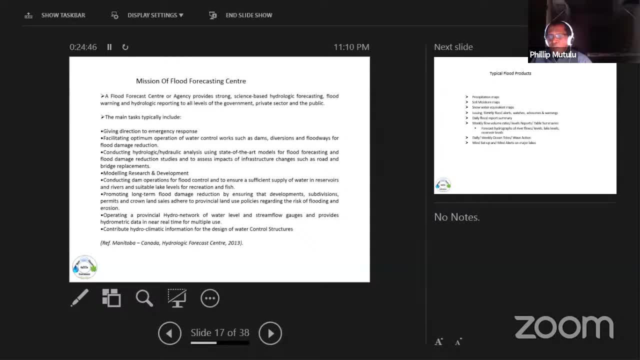 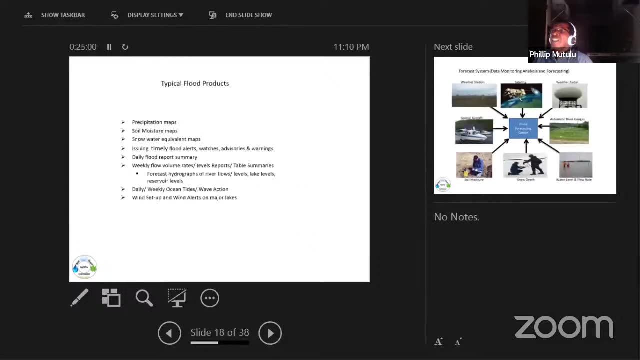 like the data that you're going to provide to a public person or to the communities that need to evacuate, so the data must be, the information must be tailored to the need of the consumer, and there are different types of typical flood products depending on where you come from, where. 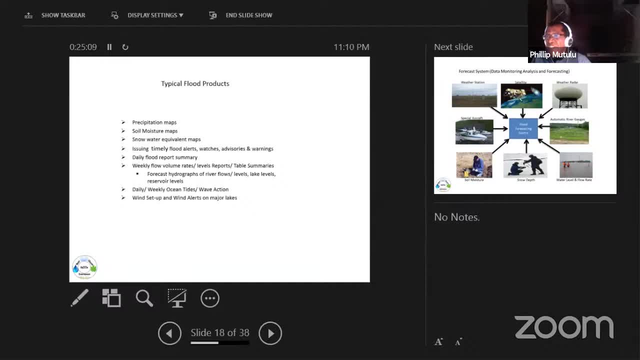 they come from north america, canada or india. um, these uh products change with time and sometimes they are driven by stakeholders. um, you know, they would come and say: yo, we need this type of flood, we need to prepare our, our farms, so can you provide a weekly forecast for you know soil moisture, which is a part of flood forecasting. so they are all different. 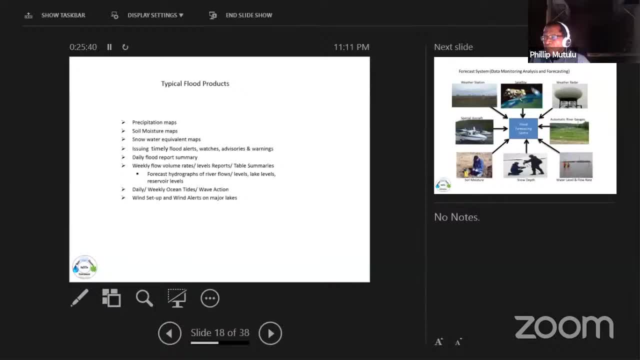 types and in a typical uh flood forecasting center you'll find precipitation maps being prepared on a frequent basis: uh soil moisture maps, snow water equivalent maps in like in canada, where we have problems of snow. we issue also the issue timely flood alerts, watches, adversaries and warnings, providing daily flood report summaries. weekly flow volumes. 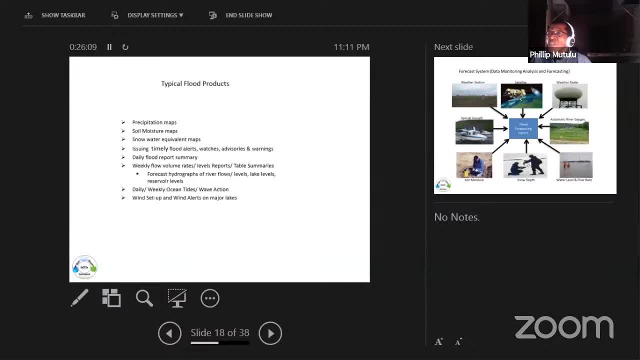 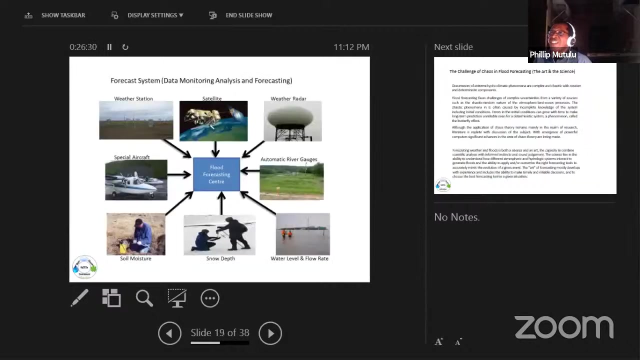 levels forecasting, river flows, lake levels, reasonable levels, daily weak ocean and wave action, wind setup, wind alerts on major lakes and so on. so i'm just trying to show you the wide responsibility that a flat focus center has. it's a lot of data products that are needed and, um, with that introductory uh in uh for what happens in a forecasting center, let us 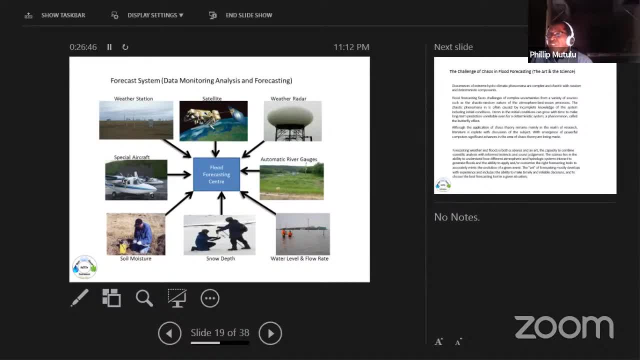 just uh. go now into forecasting tools. in a forecasting tool, you need data, of course, and uh, this data comes from diverse places. um could be from weather stations, from satellites, from weather radars, from automatic river gauges, from space spatial crafts, soil, moisture, snow, depth, water levels and now more modern. 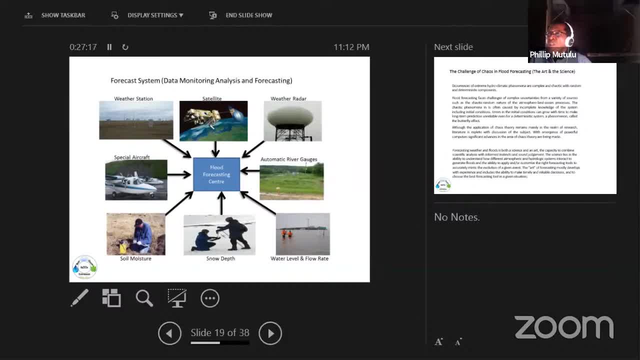 flood forecasting systems are also using data from numerical weather prediction models and also drones. i'll briefly talk about the drones as we towards the end of the presentation. so it's a huge amount of data, and the thing that i would like to underscore here is the need for the government to invest adequately. 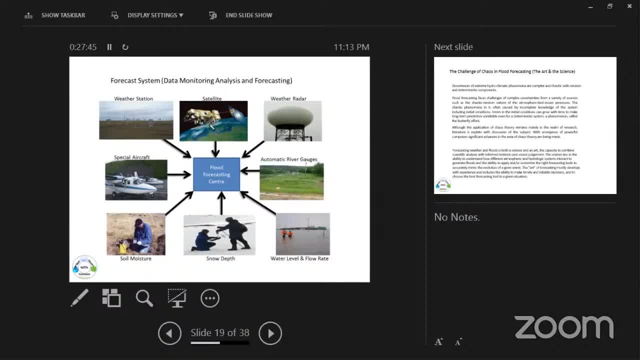 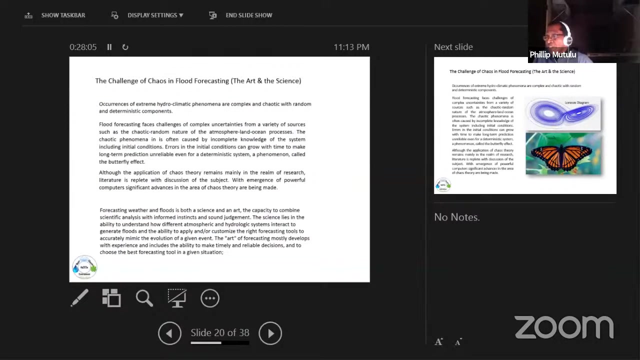 to have monitoring stations that are sufficient to provide data that is required to give accurate focus. yes, um, and once you update that data, what do you do with it? you have to put it somewhere so that, uh, you can provide a forecast, but i want, just before we go there, let me. 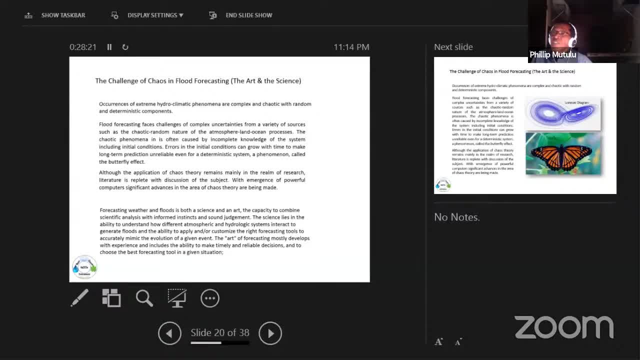 just expose ourselves to some of the challenges in forecasting. like some of you that are aware maybe- i don't know whether you know- he has been involved in weather forecasting. uh, i was a weather forecaster before i became a flood forecaster, so i have backgrounds in both meteorology and flood. 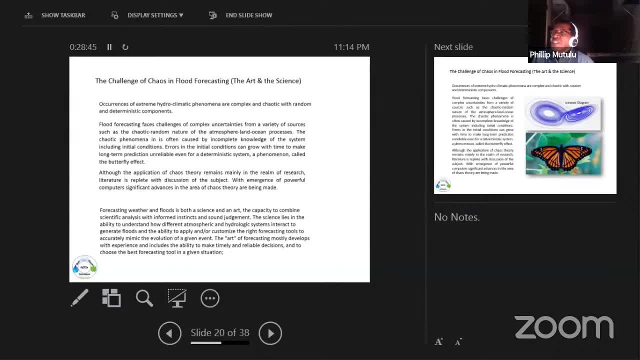 um the occurrence of extreme hydroclimatic phenomenon are complex and chaotic, with random and deterministic components. flood forecasting faces challenges of complex uncertainties from a variety of sources, such as chaotic, random nature of the atmosphere, land, ocean processes. the chaotic phenomena is often caused by incomplete knowledge of the system, including initial conditions, errors in the initial conditions. 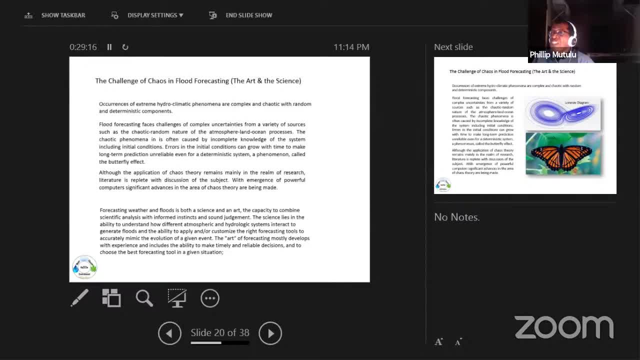 can grow with time to make long-term prediction unreliable, even for a deterministic system. we shall see what a deterministic system. you know shortly a phenomena called the butterfly effect. i guess some of you most likely you've heard of the butterfly effect. although the application of chaos theory remains mainly in the realm of research, literature is 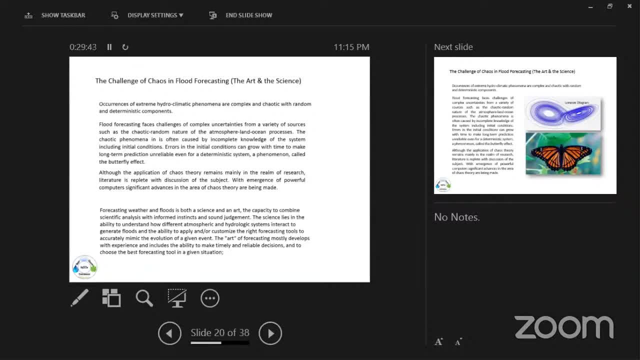 replete with discussions of the subject. for those that are interested, you can search on the internet. and the treatment of chaotic systems requires very huge, uh, computer power. but i think now, with the emergence of powerful computer, significant advances in the area of chaos theory are being made. uh, if you had the, the story of butterfly. 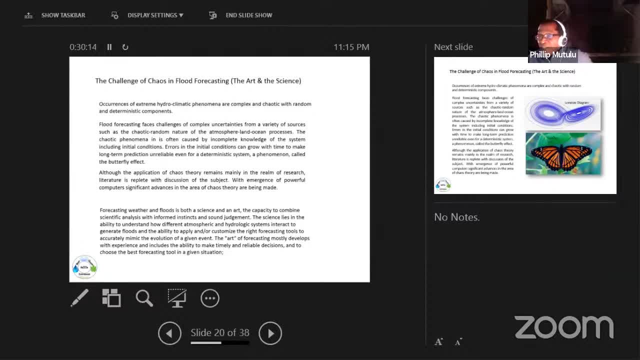 somebody say that a butterfly just flapping its wing, you know the effect might seem small, but that effect can grow and they have a have a an impact somewhere very far away. um, that's called the butterfly effect and this effect usually is problematic in weather and flat forecasting. 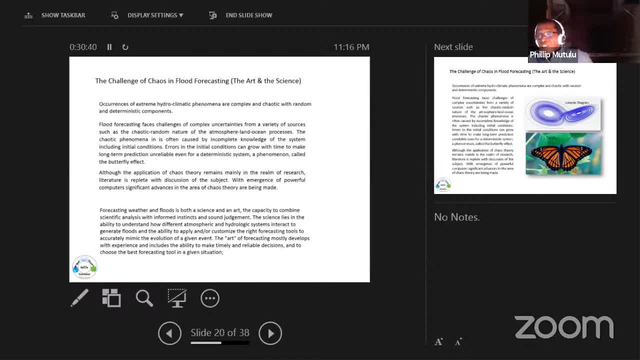 because it means that if the initial conditions of your system are not well known, then you will not be able to forecast your rainfall or your flood very well, because the error, any perturbation or any disturbance of the initial system is not well captured and then you'll not be able to do that forecast well, forecasting weather and flood. 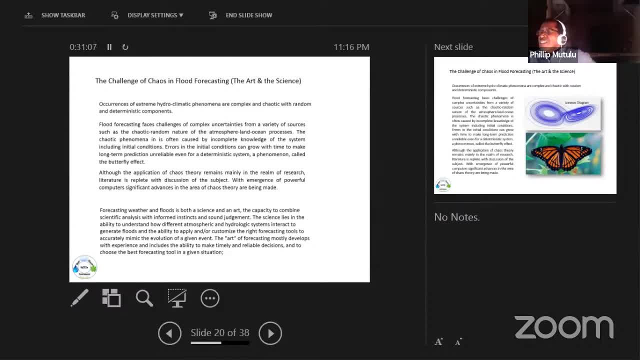 is both a science and a nut. i think i need to say that the capacity to combine scientific analysis and the ability to draw on the facts to create a more accurate and realistic outcome is not only an issue of what the weather is or what the weather is, but it is also an issue of the 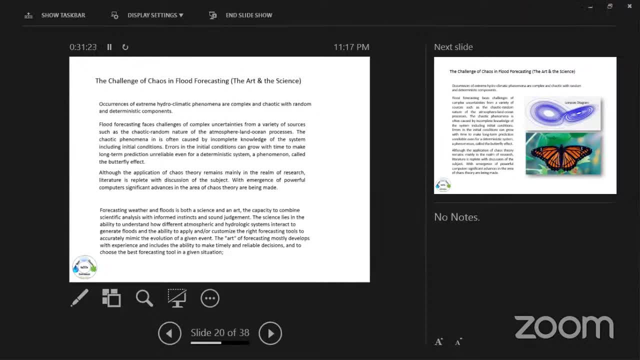 environmental impact that is produced if there is a strong amount of rain and the weather is not good, and so on and so forth, and so forth, and so on. the problem is that it's not so easy to predict what will happen in the future. but i think the problem is that the issue of the weather is 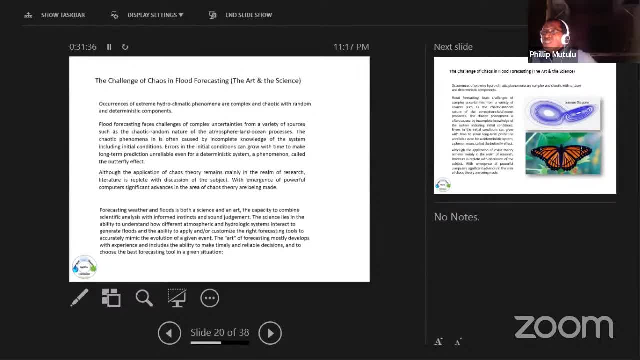 very important. it is not an issue of weather, but it is an issue of what will happen in the future. so, anyway, what i'm saying that, uh, for us, or for our um agencies, to be able to provide good focus, they need both the science and the experience you may have: the science, the knowledge, the mathematics. 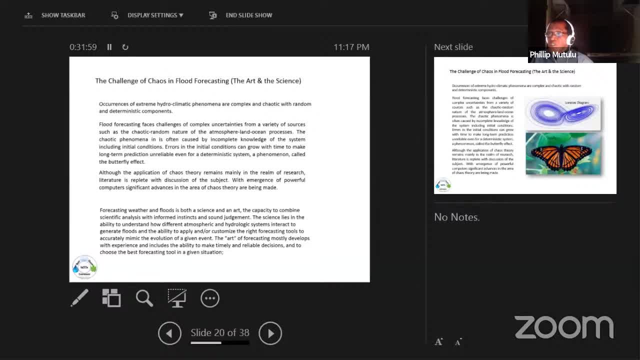 but you will lack the nutrition. sometimes you you'll even find the mathematics don't work at all and you have to make very quickly decision, and that can only come from experience. so for those of you who are students, who are looking to become focused as um, that's something that. 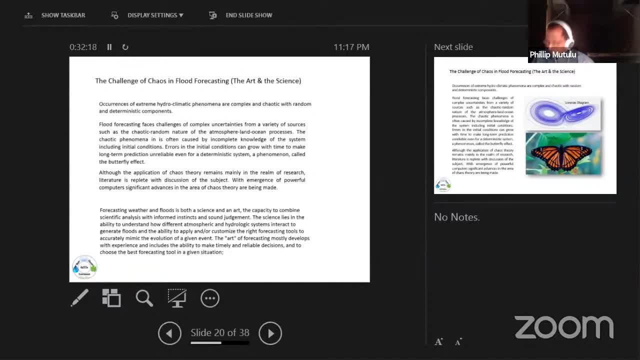 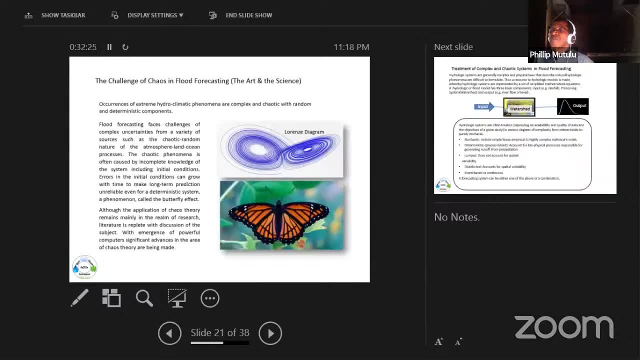 you'll have to learn along the way. um, so those are just an off-site statement, but these are cautionary statements that i wanted to make right from the beginning. um, that's um, just a picture of a butterfly, and they also have a very interesting effect. it's also called lorenz diagram, if you are for those that. 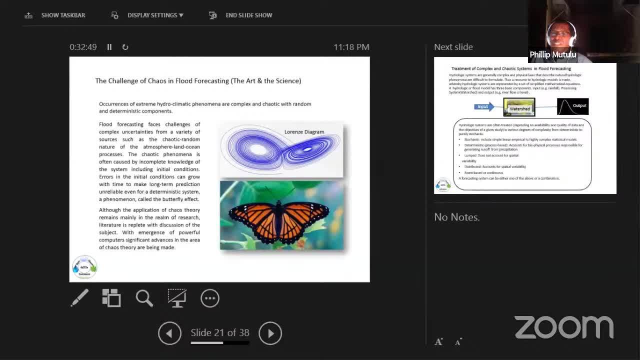 are interested, you can go and do such. there are books on that theory of chaos in the atmosphere, which translates to chaotic processes in flat forecasting, because you cannot separate floods from the atmosphere. uh, without the atmosphere then there are no floods. so disturbances occur in the atmosphere. during a flood event, they will be propagated in your 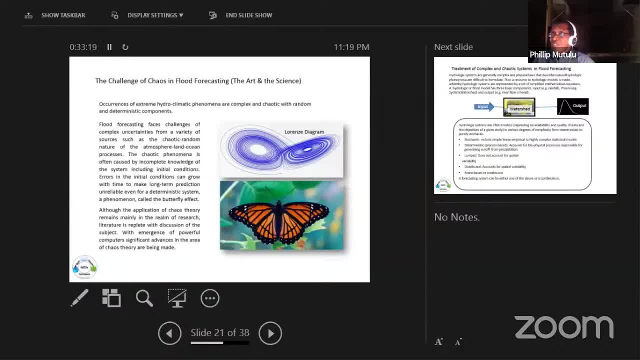 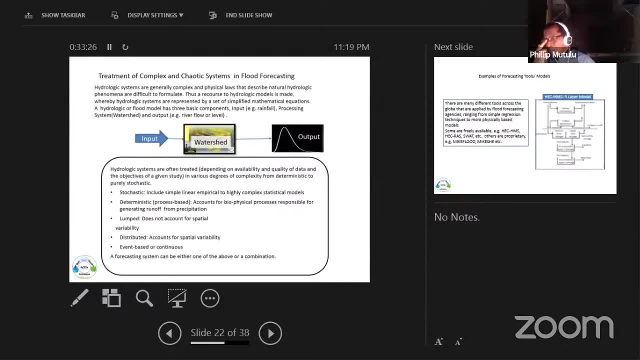 forecast system. anyway, that's a bit aside, but it's a very interesting subject. it's a very complex subject, but some of you might want to explore that. um, so how do you treat these complex systems in flood forecasting? hydrologic systems are generally complex and physical laws that describe natural. 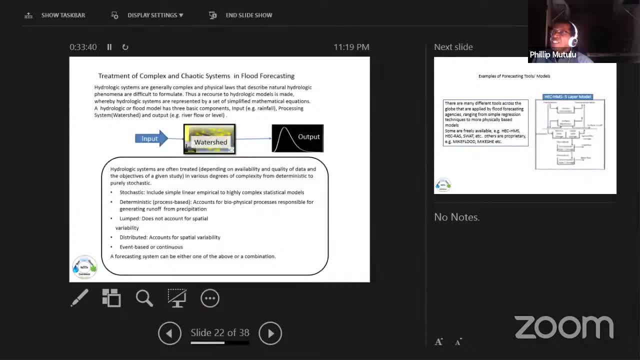 hydrologic phenomena are difficult to formulate. thus, a recourse to hydrologic models is made, whereby hydrologic systems are represented by a set of simplified mathematical equations. a hydrologic or flood model has three basic components. the first component is the input, for instance the rainfall. then, right in the middle, you have 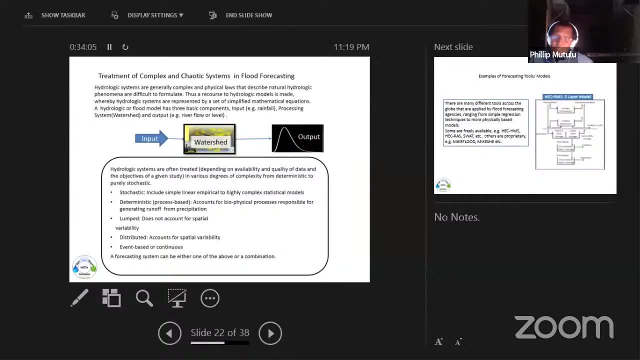 the processing system, which is called the watershed. so you are. it's like um the system, the watershed system, takes in input and then it processes that input and translates that input into output. that processing or that procedure of transformation is represented by a mathematical, can be represented by a mathematical model. 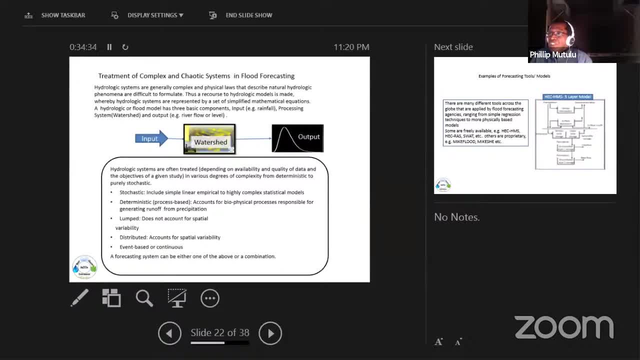 so you have input, then the watershed and the output to which you're inputting the information that comes out of the project. just to simplify, hydrologic systems are often treated, depending on availability and quality of data and objective of a given study, in various degrees of complexity. 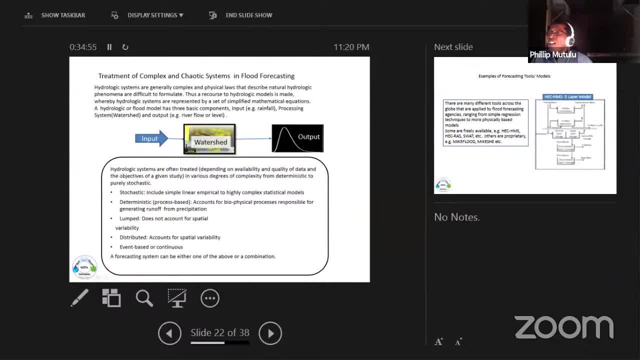 from deterministic to purely stochastic. um, stochastic- another word for stochastic- is uh probability of statistics, if you want to be to sound simple, but we are to use the word stochastic in uh floods and hydrological systems. This includes simple, linear, empirical to highly complex statistical methods. Some of the linear methods that you can use to forecast a flood from rainfall is building. 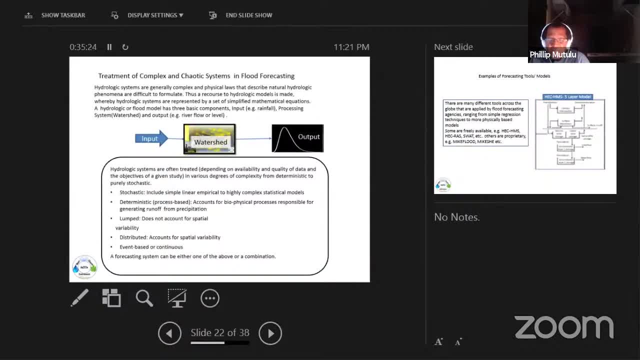 a simple linear regression equation. But then, because these hydrologic systems are not linear, you will find that your regression equation doesn't give a good forecast. So you want to go to the complex that describes what is happening in a hydrologic system. 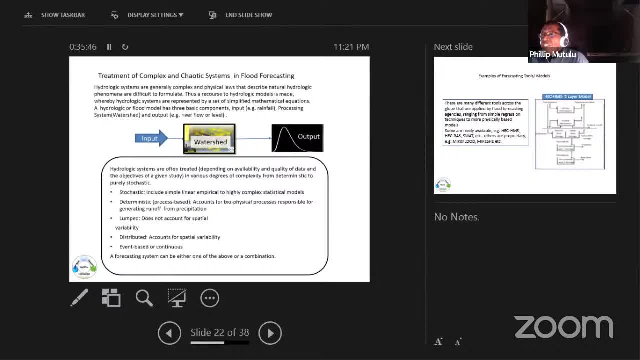 So, secondly, we have deterministic, which are so-called process-based models, And these are able to account for biophysical processes that are responsible for generating runoff from precipitation. Then you have LAMPT. These are type of models, And these are type of models that do not consider spatial variability. 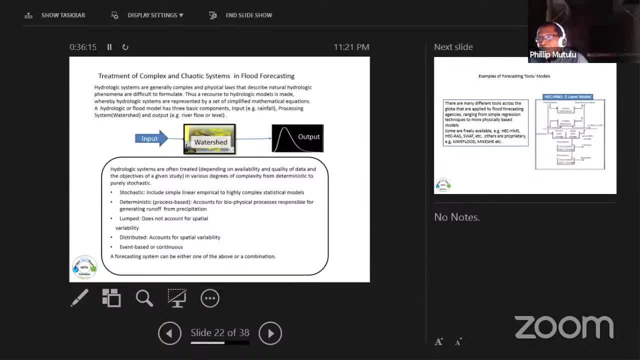 For those of you that are experts in GIS, you know how important it is to model spatial variabilities in processes in an environment, And therefore this LAMPT model does not account for that variability. But very interesting thing is that some of these LAMPT models do not account for that. 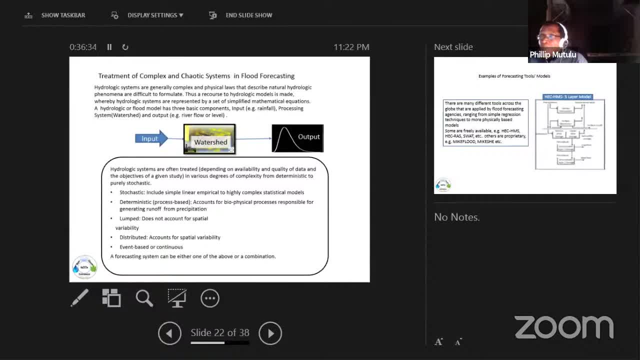 variability. These LAMPT models can even work better than some of the physically based models in some cases. Yeah, that's what we found when we are forecasting, And so that's why I brought it up there. It could be simple. It does not account for the spatial variability. 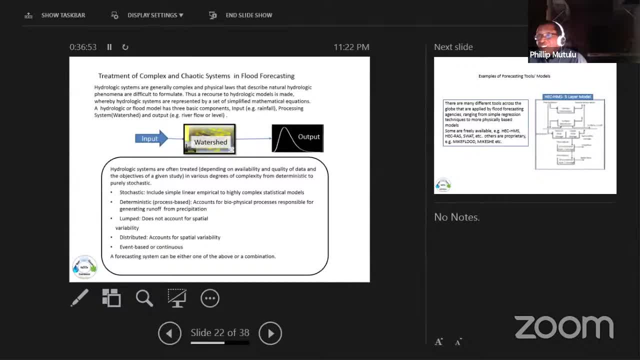 But during extreme flood events sometimes you find that they work actually pretty good. Then this distributed modeling: That is where you can account for variability: Spatial variability, Spatial variability in soil, vegetation, land use and so on. Then you also have event-based or continuous events. 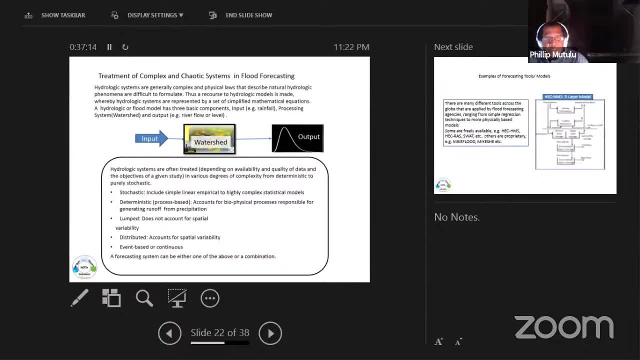 Event is something that happens like a short lasting storm which lasts only for six hours or 24 hours, And some of these intense events are actually responsible for very heavy flash flooding and so on. And so when you build a model, So you want to know whether your model is going to be forecasting just events like those. 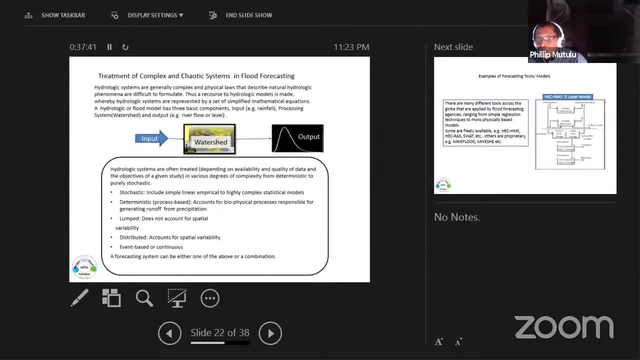 ones extreme events, or it is a continuous system. A continuous one will track moisture for a long time over the years, throughout the year, And then, when the rains are about to come, it will already be knowing what was the moisture in the soil three months ago. 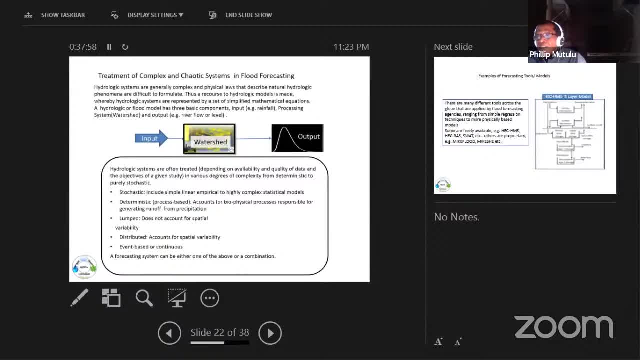 And therefore, when the rain comes, it is able to forecast what the flood, what, what, what type of flood and the quantity of flood will be generated from that rainfall event. So a forecasting system can be any of those, a combination of the above, and typically 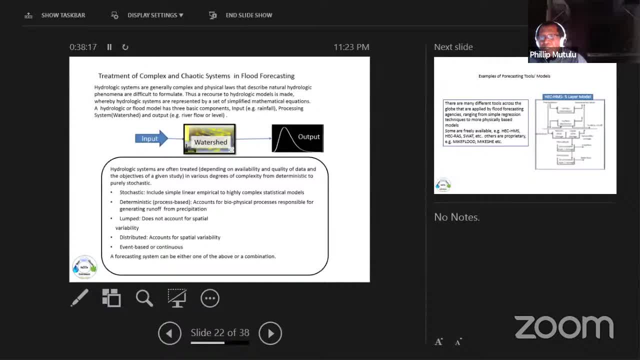 the recommended that you use combined methods, And that's where you'll find that in forecasting, there's not really a single forecasting technique that works, And that which works better seems to work better. And that's where you'll find that in forecasting, there's not really a single forecasting technique. 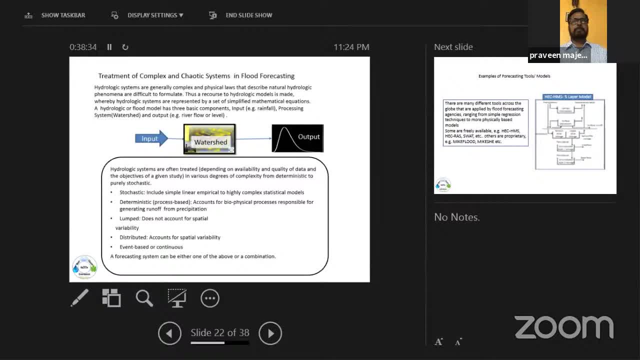 that works And that which works better seems to be a combination of any of the above, And sometimes, actually, when you are doing actual operational forecasting, you'll find that even your model doesn't work and you have to quickly do some calculations aside. 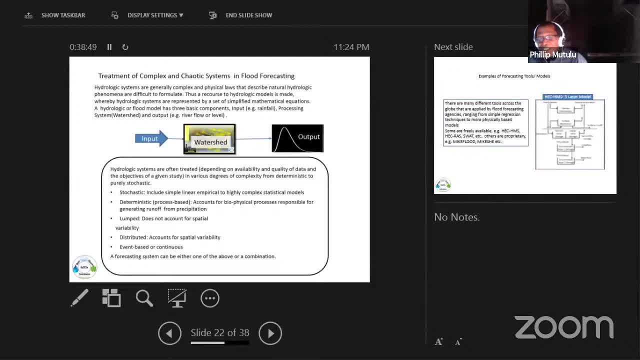 you know addition and subtraction here and division there and there to come up with with some numbers. because you know the hydrologic systems are very complex, as we have said, starting from the atmosphere to the ground, to the vegetation and so on. 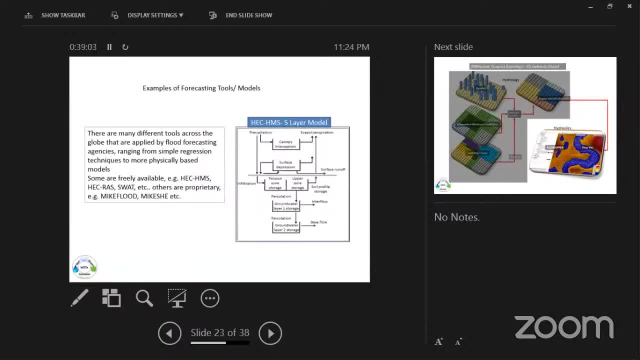 Some examples of these tools. There are many forecasting tools, And some of them are available for free. Others are propriety, And so it's upon every government agency to decide what they want. If they want very complex models, they may have to buy it for several thousands of dollars. 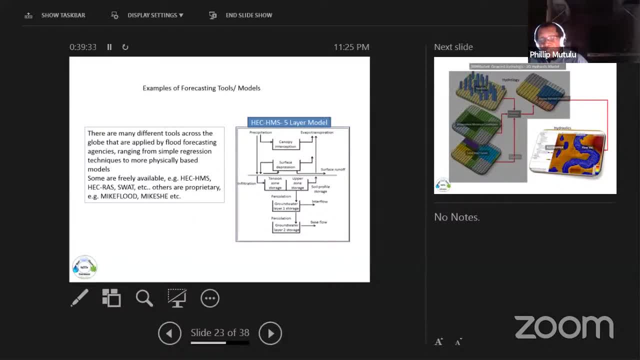 dollars, but still they can pro. they can also go for free software that is available on the internet for free, and actually some of these free software are being used very effectively, not only north america but in india. you know models like hms across and swat. you know that they are being. 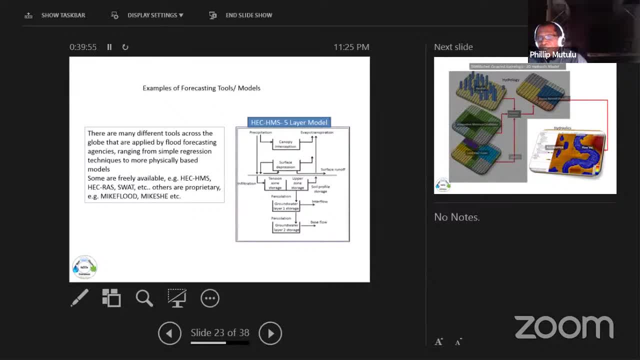 used by agencies in north america and india and other places, and these are all free, uh, others like mike flood, mike she, you have to buy them, but, um, you know they are expensive and typically what an agency wants to do is to test different forecasting techniques. uh, before, 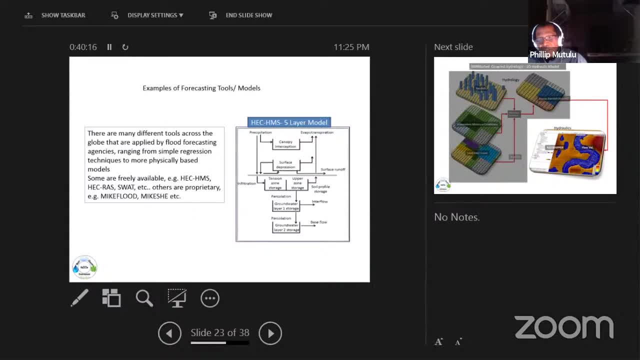 they can say: this is what works best. five years ago, i was involved in a project in canada here where we evaluated different forecasting methods and rated them, and we submitted that to the government, and so it's always important if a nation or a country is going to establish a 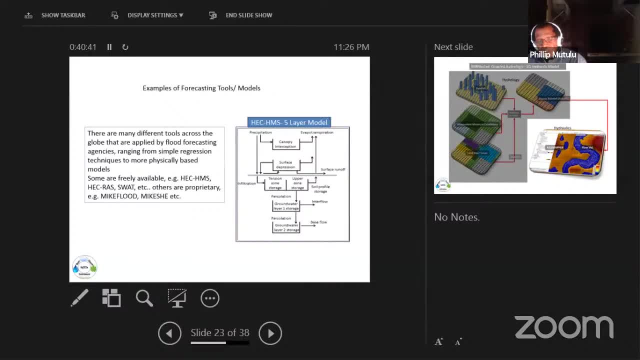 forecasting system. it is not wise for them to just call a consulting firm to establish a focus system, because it might not work. what they need first is to evaluate different forecasting schemes and see which one works best. then you can say, for example, if, for example, if- korea wants to do a lot of forecasting. 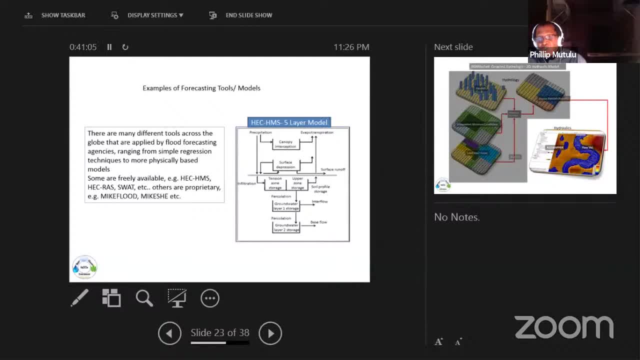 or nigeria wants to do a lot of forecasting, then if the investing wants to not work, then they need researchers from the university who can help them with research and research into tools that can be used as complementary methods to help them focus better. that's why we need research. 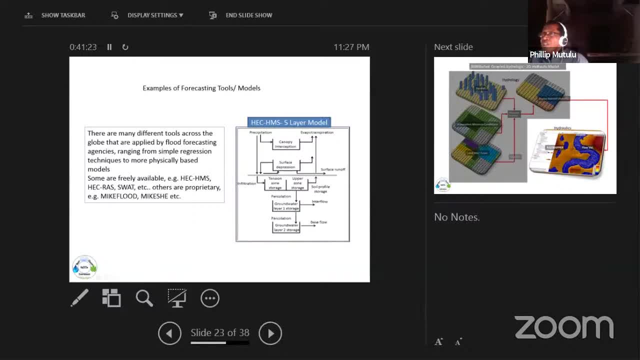 you remember i mentioned that one mandate of a forecasting center is to be involved in research for better tools of forecasting. uh, on your right hand side there you have one of the models. it's actually a simplified model but it's not a simple model. but if we look at the research examination, 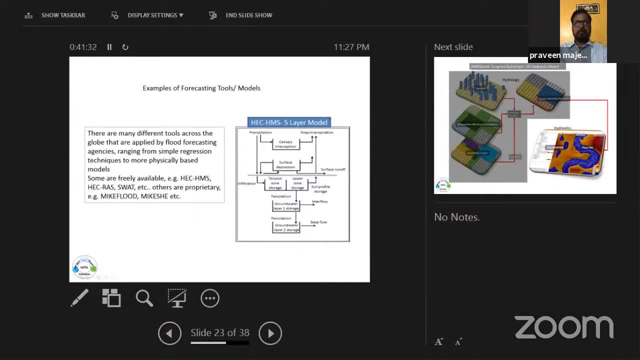 But a model like this one. you can see that it represents about five layers of the hydrologic system, starting from the vegetation, surface depression and surface zone percolation, groundwater percolation. All these processes are represented by mathematical equations for those that are familiar with hydrologic models. 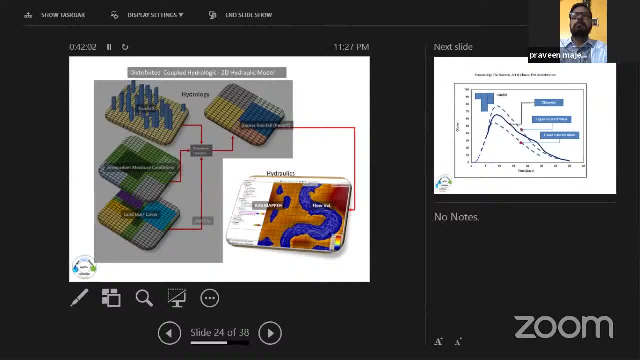 Currently, what's happening is that there's a push towards integrating what is called hydrologic models and hydraulic models, and that's one of the things that the Mike Chee and Mike Flatt do In this case. what I showed earlier on, I showed you a HEC-HMS model that is really hydrologic and it deals mainly with the hydrology. 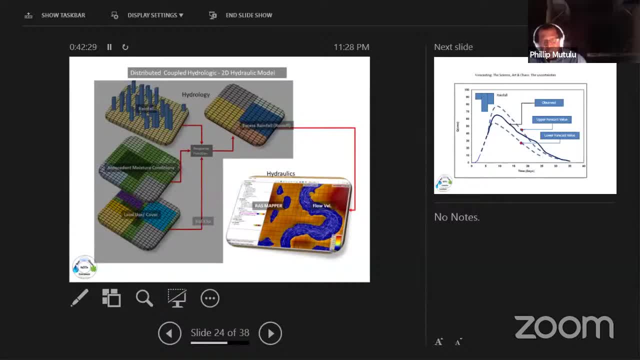 But when you want to see how water moves through channels, through pipes- if there are pipes or channels or canals in your system- then you want to use hydraulic models And therefore, what the push is currently is to couple hydrologic and hydraulics model. 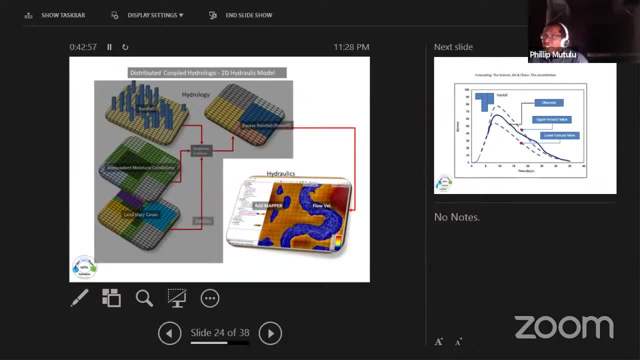 Here. I've showed an example here and the hydrologic model provides something like the surface runoff. Now, when it rains, some of the water infiltrates into the ground. some water evaporates. water remains after it fills the ponds on the surface. then some of that water becomes runoff. 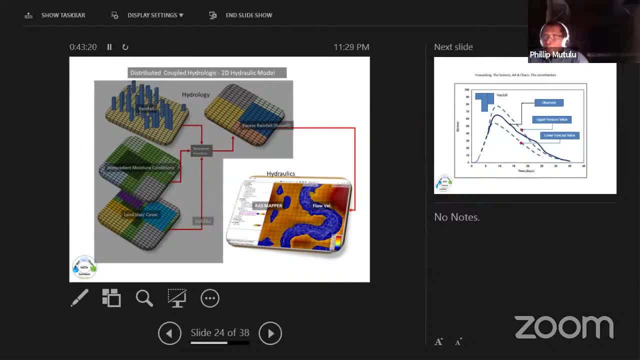 But then how this water is going to move through channels is modeled using hydraulics And you know we we can have several layers of this system in a hydrologic hydraulic model And these layers are well captured by using GIS system. 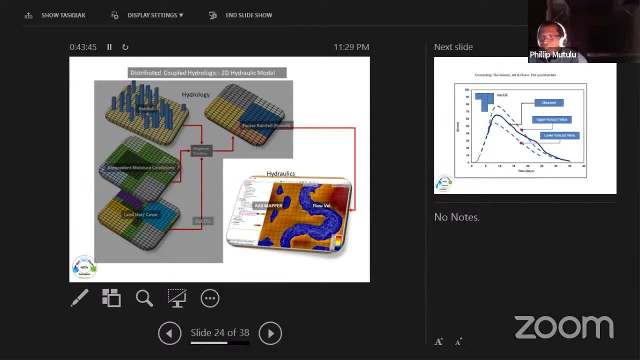 Dr Archner, of course, last time presented application of GIS, And so GIS applications are finding very wide applications in flood forecasting. Actually, there's no flood most of the flood forecasting, but there are some very interesting tools that are being developed today. 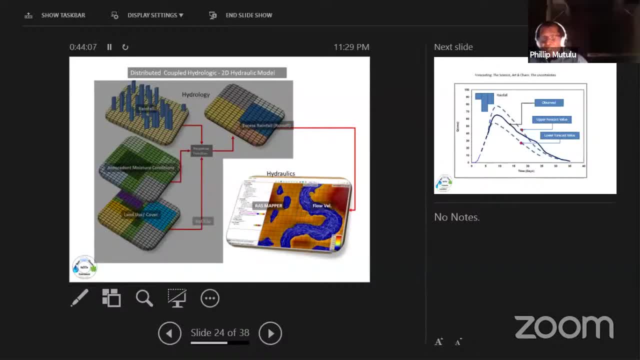 They have GIS components so that you can be able to integrate different layers of data and then operate, do some mathematical operations between these different layers so that you can come up with your flood forecast. So the first layer could be a layer of rainfall. 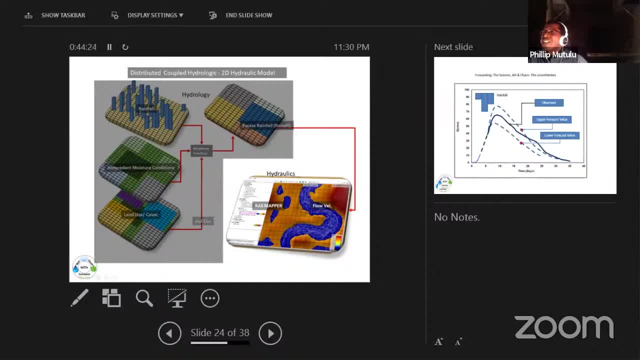 The second layer could be moisture, The third layer could be land use. After that you have a response equation there. And then the fourth layer is the excess rainfall or runoff, And that layer now is led into hydraulics layer down there. 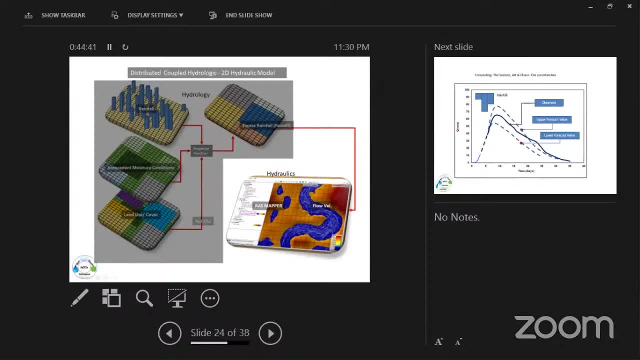 which routes the flow. So these layers operate on one another using mathematical models. I'm really sure those of you who have interest in GIS they exactly know what I'm talking about. So these layers can operate upon one another through mathematical equations, which are the models: hydrologic and hydraulic models. 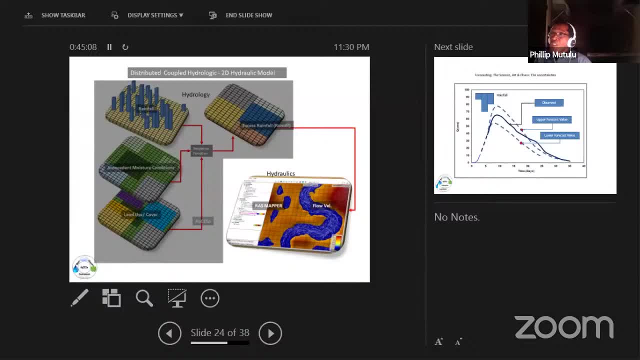 So this push towards distributed coupled hydrologic models coupled with 2D hydraulic models, because that's the only way we can capture the type of floods that we are getting today. We need to see them move in all directions. In fact, now these are pushed towards three-dimensional models. 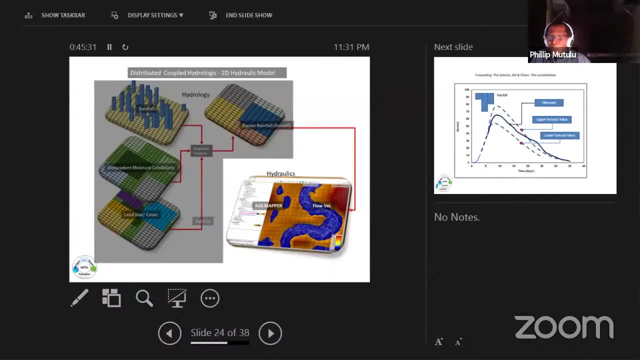 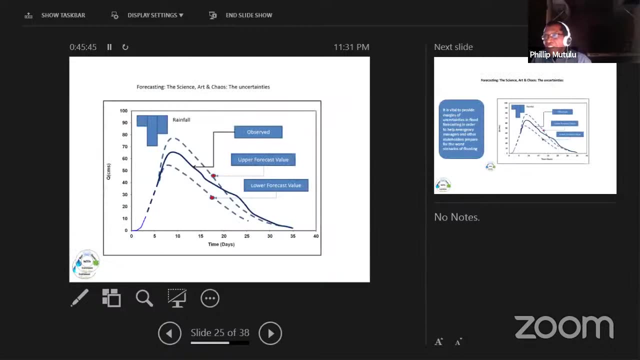 where you can be able to simulate the vertical motion of floods. But basically what is working out today is the two-dimensional, where you have the X Y, Z X Y variations. Now, when you are doing forecasting, there's something very important in this. 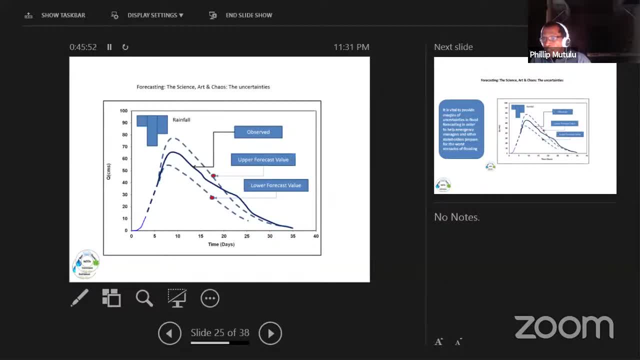 Because of the chaotic nature or random nature of the atmosphere in the hydrologic systems. you are not just going to give a single number. You need to tell the people who are receiving the forecast. yeah, this is my forecast, But because there are a lot of uncertainties because of data, 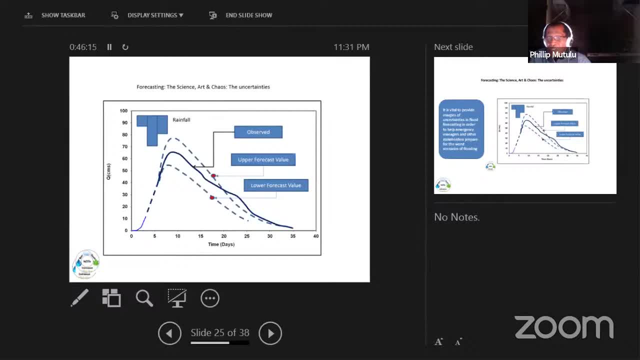 because of incomplete knowledge of the system. I think my range of focus should lie between these two points. So you give an upper range, the middle range and then the lower range, And typically that helps prepare the emergency preparedness. People know how to prepare for the worst conditions. 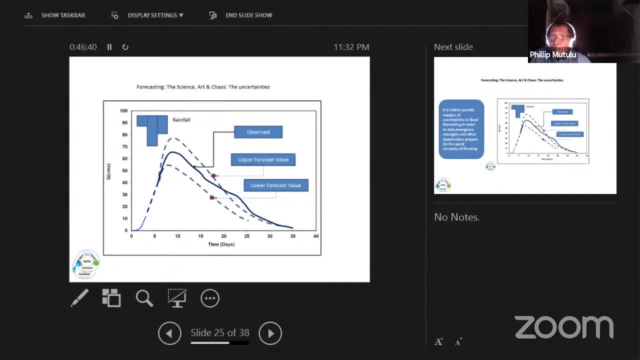 because you have told them the upper possible number of the flood volume that you can see. And so, when you are focused, be aware that you need to give provide information that will help people prepare for the worst. You know, even if the worst does not happen. 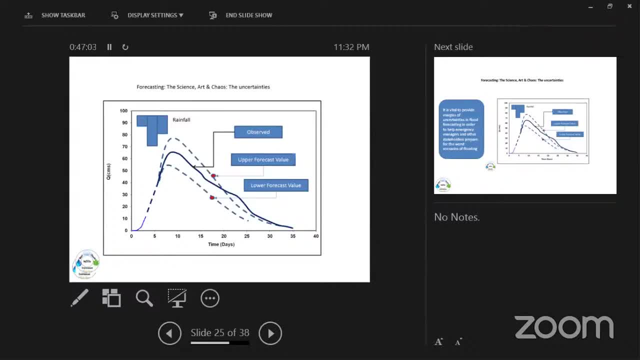 at least you are prepared. It's better that it doesn't happen, But if it happens, then you are going into danger, And that's where sometimes the meteorologists and the flood focus find themselves in danger because they focus something high and then people are evacuated. 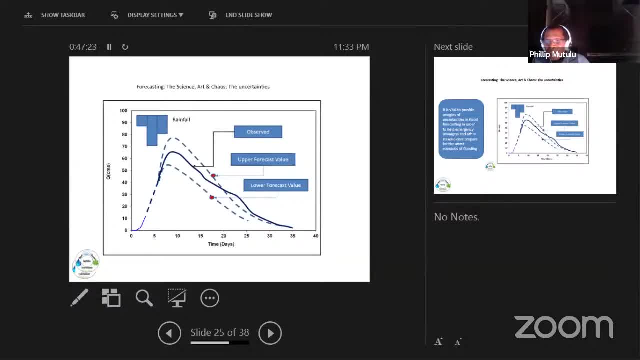 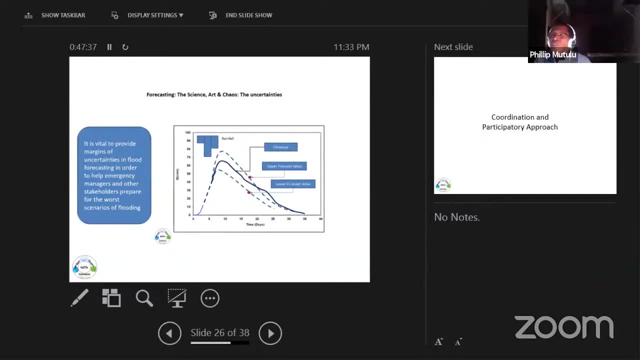 but nothing happens. But you see, the long-term gain is usually worth it. Always provide the largest number, Go partner. So it's vital to provide margins of uncertainties in flood forecasting in order to help emergency managers and other stakeholders prepare for the worst scenario. 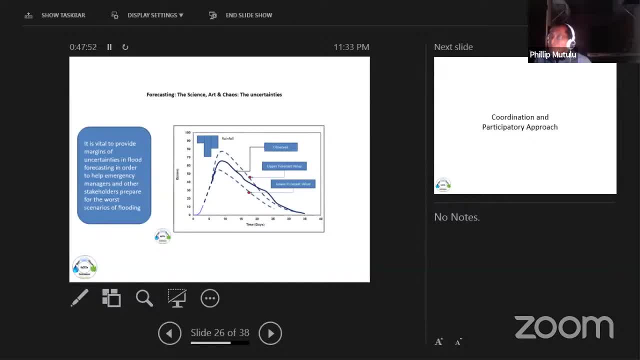 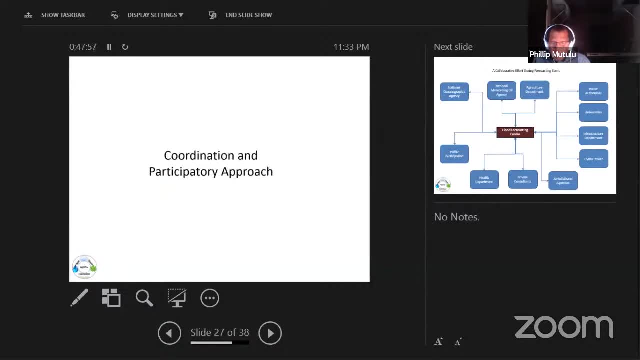 of flooding. Now, what you have seen in my presentation in the previous slides is a lot of information that goes into forecasting tool. So diverse information also means different groups of people that would be involved, And that's why there's a need for very strict coordination. 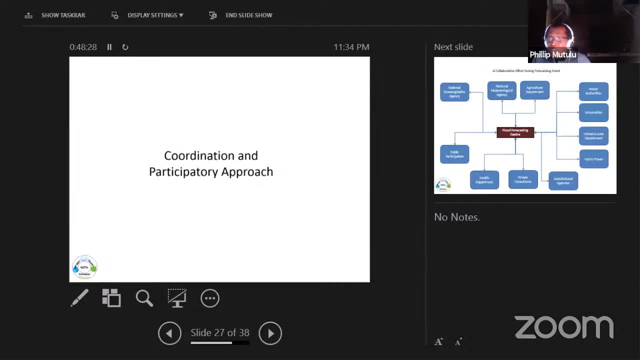 and participatory approach. This is a type of approaches that are becoming more popular, where forecasting agencies are now involving the communities in their forecasting systems, And I think one of the best forecasting systems, especially for flood forecasting, is the flood forecasting system, Especially for flash flooding, is in India. 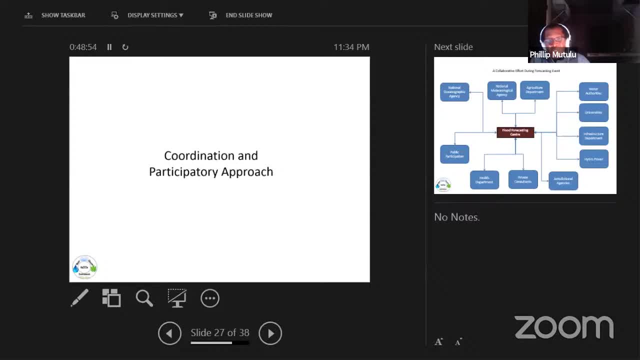 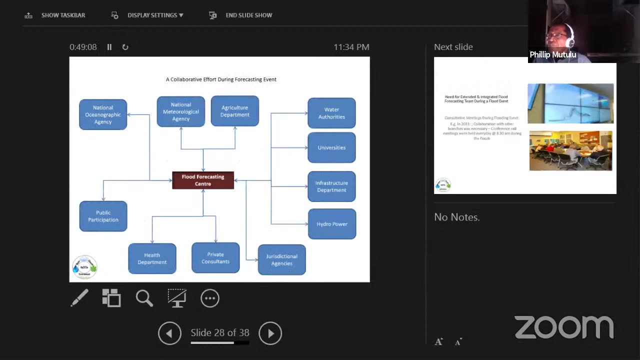 where they involve the local communities. Sometimes it involves even sending information about how is the river behaving in that local area. How is it You send that information? It is so integrated in forecasting system, So this chart here will differ from different agencies. 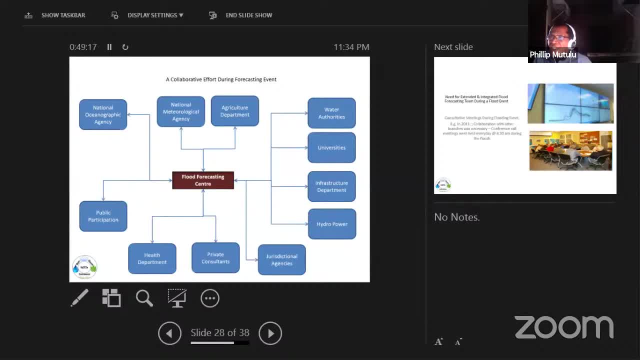 but it does just show the linkages or synergies between a flood forecasting center, different governments, sectors or departments, Because you cannot focus there as an entity. you really need to know what people need out there And as they give you feedback. 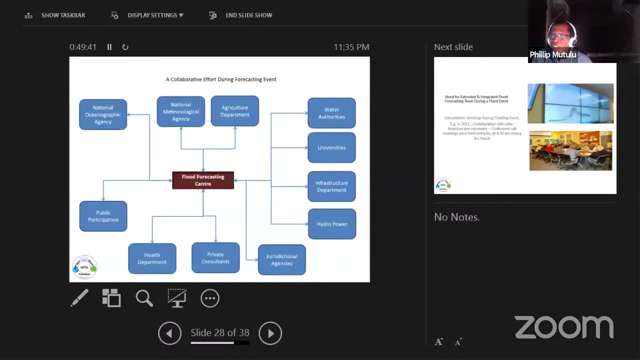 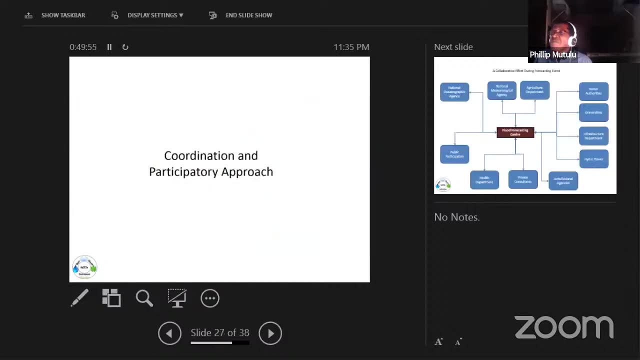 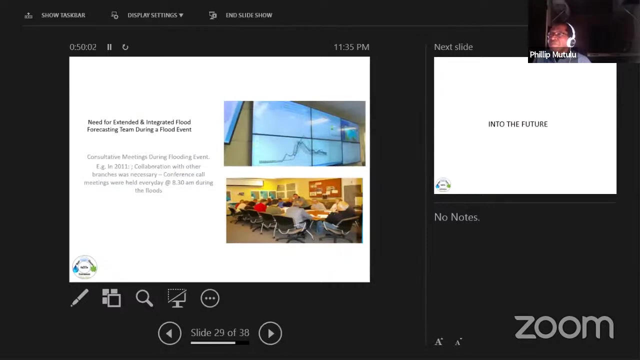 then you know exactly, you can tailor your information so that it is most useful to them. So you cannot work in isolation. It is a forecast that you need to. there is a need for participation of different agencies And then during the, when there is a flood event. 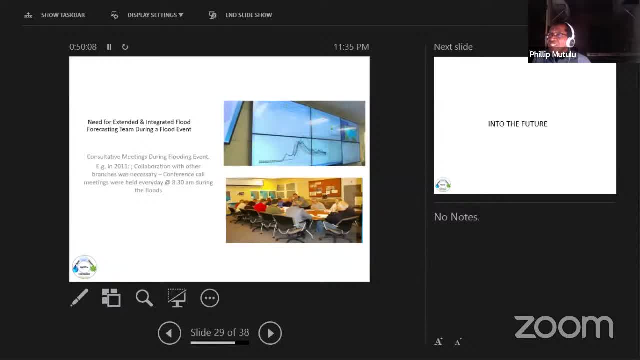 one of the things that happens is that there are frequent meetings of different stakeholders- consultants, emergency measures forecasters and so on- And that is something also that is popular in India, And all these people discuss as the flood event happens. the forecast will provide. 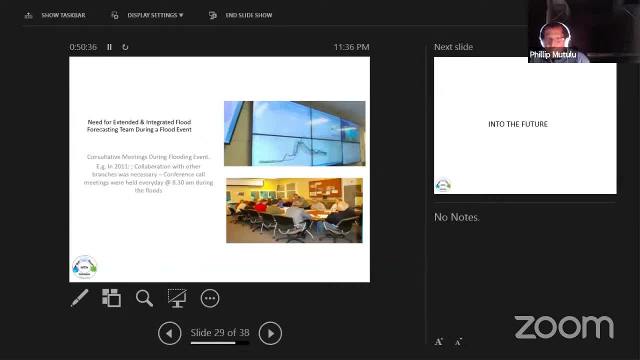 what is it that you are forecasting? Where are we going to need to evacuate people? Where do we need to operate our water control structures? And therefore, this is a picture where you might see me somewhere there, but it's a picture in our flood. 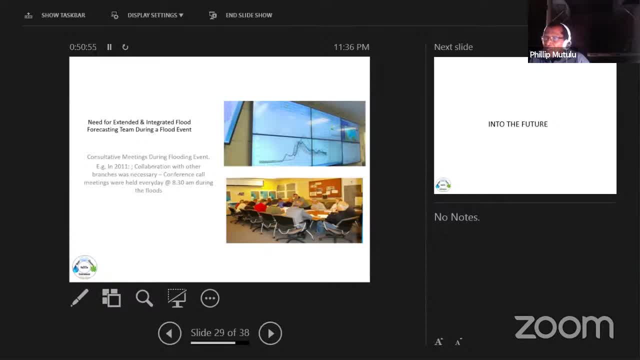 the flood forecasting center that I used to head Every morning at 8.30, we used to have consultative meetings And at that time there was a heavy flood and, you know, houses and properties were being washed away And it was very important that we consult one another. 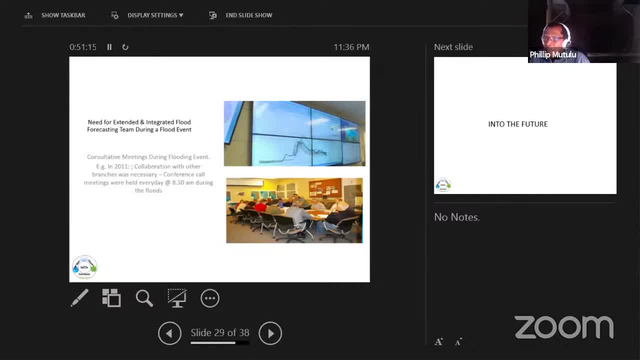 and make the best decision for that day and provide the information in a timely manner, And therefore it's almost overwhelming. This is not a job that a forecaster can do alone. He'll have to rely on other people to be able to provide the best product. 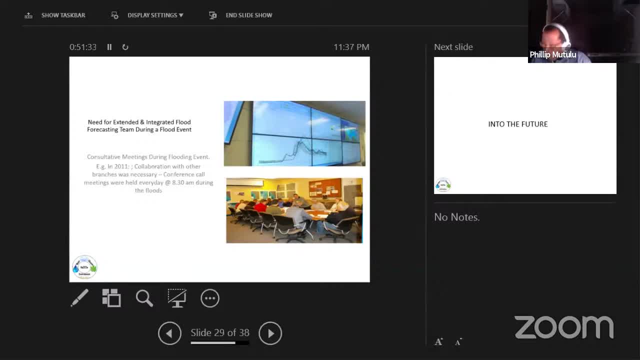 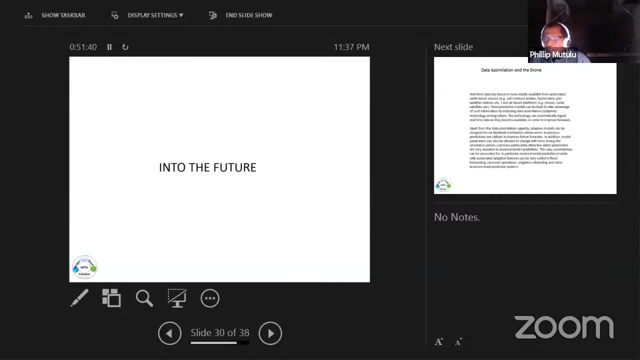 that can be consumed by the people outside there. So, as a recap, we have seen the need for data monitoring, investment that is required from the government, The need to combine this data into models, The need to build models or to test models specific for every area. 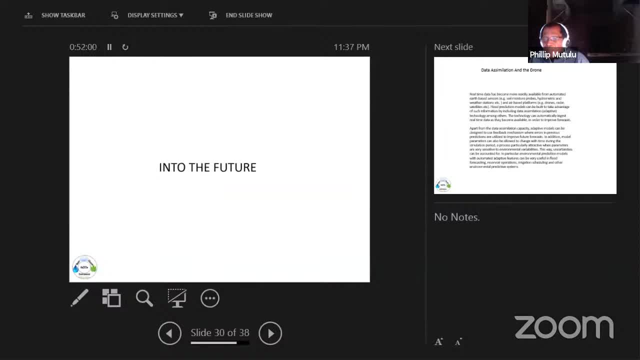 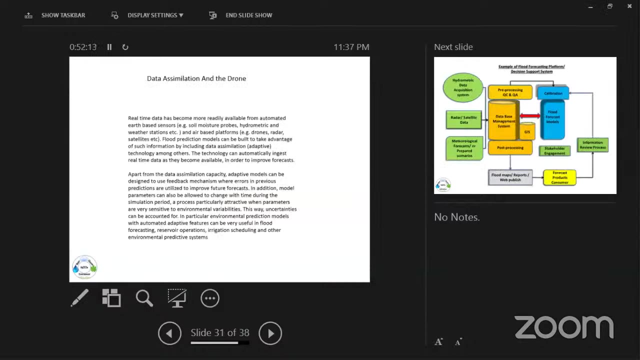 The need to collaborate with one another, with different agencies, so that you provide the right information in a timely manner to the people that need the information most. Now, looking into the future, a lot of information is now available, especially from different sensors that are being sent into the atmosphere. 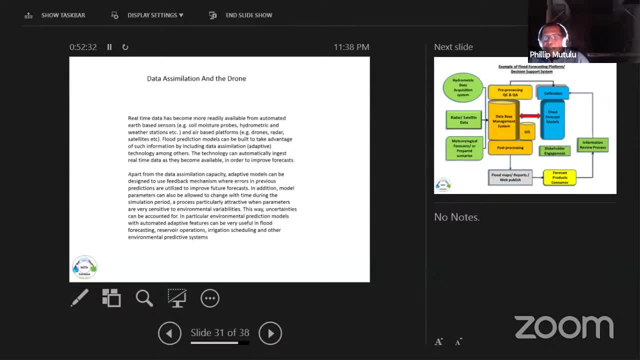 whether these are satellite-based or radar or the drone, And there's even a, a science or a specialty that is emerging of data. you know, big data, big data, big data. branch of education: I think they are already offering that in universities. 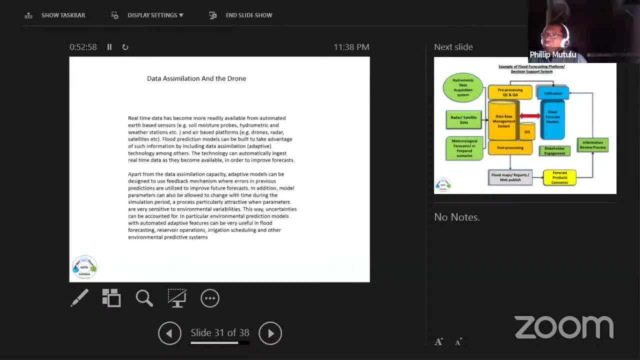 So data simulation- And I just put a drone there because it's become so popular and recently it is being used in flooding, not only in mapping, I mean, it is also providing focus and support. It is providing focus in some areas. 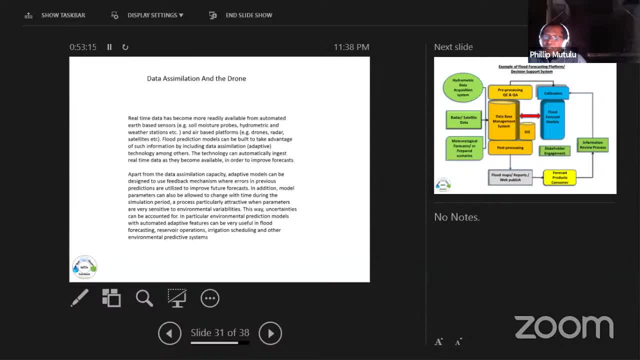 So I think I need to you know. moving to the future, the drone is going to be an aircraft that will become popular in a flood forecasting because the good thing it can be localized. You know there are a lot of drones. 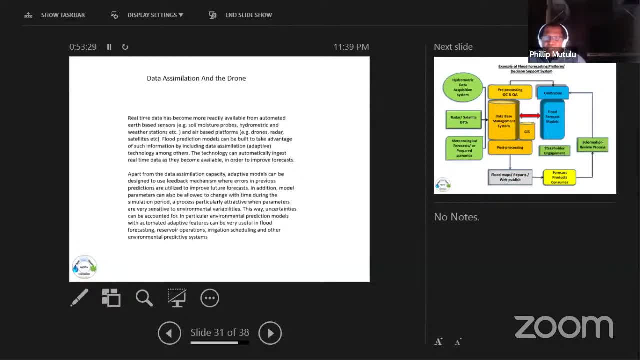 all around the globe and they can coordinate information with one another. They can receive information from the focus center, send pictures to focus centers, and so on. Anyway, real-time data has become more readily available From automated earth-based sensors, eg soil moisture probes. 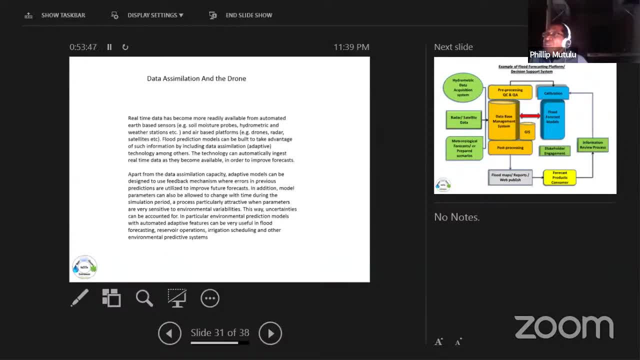 hydrometric weather station and so on, and air-based platforms, for instance drones, radar, satellites, etc. Flood prediction models can be built to take advantage of such information by including data assimilation That is called adaptive forecasting technology. 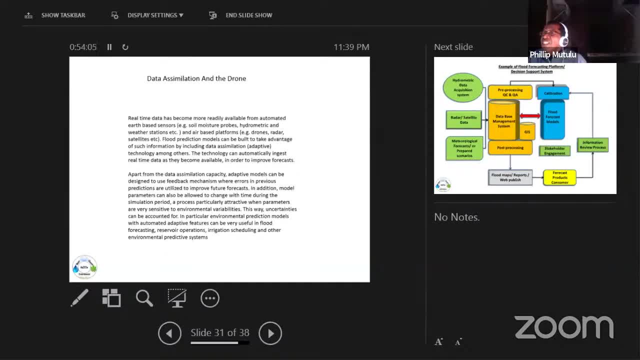 The technology can be automatically, can automatically ingest real-time data as they become available in order to improve forecast. So the technology that is being developed now for forecasting is to be able to be adaptive. The model can ingest data from the drone or from the radar directly. 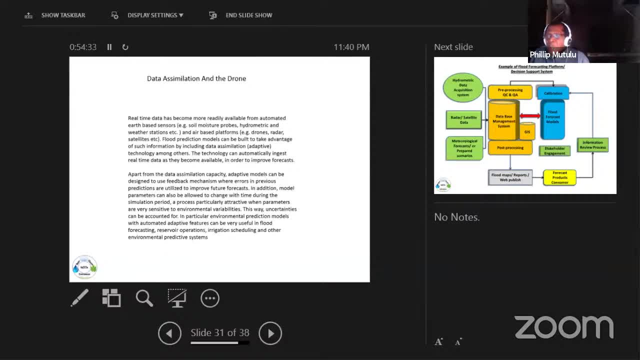 And then, as it gets that data, it updates itself and improves the forecast. The second paragraph there says: apart from the data assimilation capacity, adaptive models can be designed to use feedback mechanism where errors in previous predictions are utilized to improve future forecast. 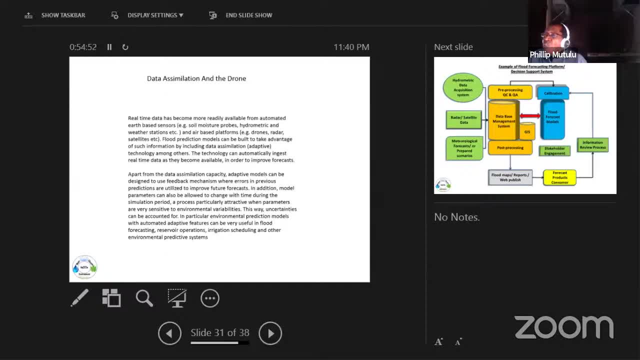 In addition, model parameters can also be allowed to change with time during the simulation period, A process particularly attractive when parameters are sensitive to environmental variability. This way, uncertainties can be accounted for. In particular, environmental prediction models with automotive adaptive features can be very useful in flood forecasting. 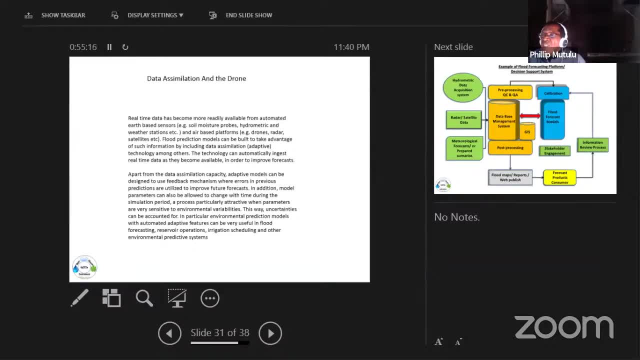 reservoir operations, irrigation scheduling and other environmental predictive systems. So here I have a system. The drone gives this system new data, So my model will update itself and then improve my future forecast. That's simply put, So the model is not a static thing. 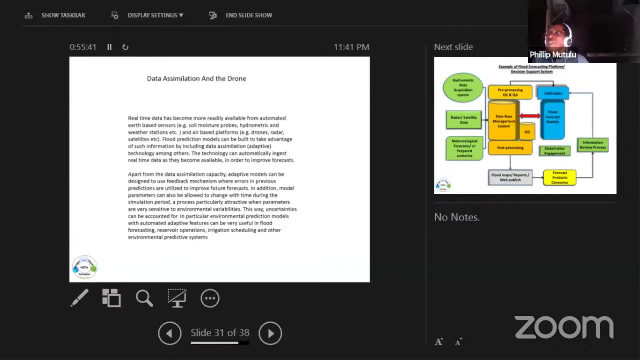 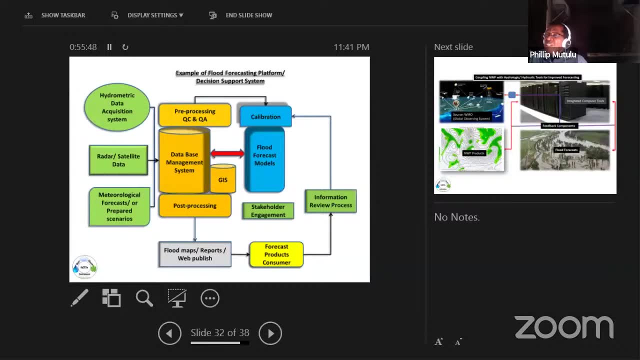 It can adapt itself, and that's where the future is moving to, And also the other thing that we are moving into future is the integrated technical components in the flood forecast, And this should be. this is a depiction of what a platform, a forecasting platform, should look like. 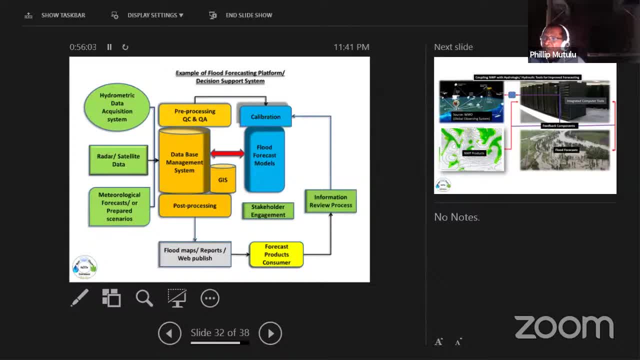 Some of them are already into this kind of platforms and some of the projects in India and North America already taken advantages of this technology, where you are putting different components together, integrating them so that you can- you can seamlessly provide a forecast. So we have a flood forecast model GIS. 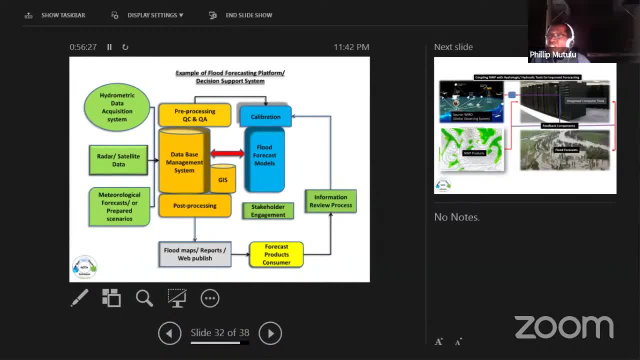 database management system, meteorological forecast, post-processors, stakeholder engagement information review process, flood maps, reports and so on and so forth. You can look at that diagram at your time, See what type of components we have. The other thing also. 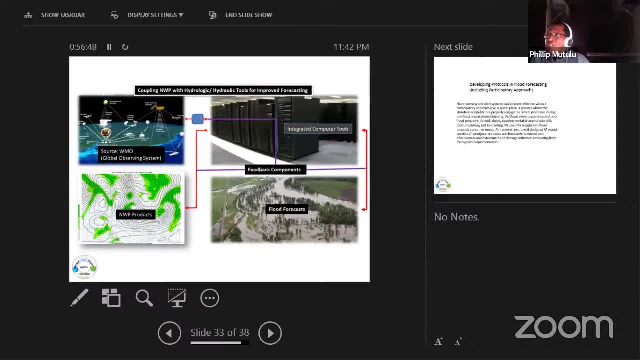 that they are trying to do is to seamlessly couple numerical weather prediction with flood forecasting models. So what you find is that now the weather forecast does not work as a separate entity, but what they have done is they have linked their tools directly to the hydrological flood forecasting model. 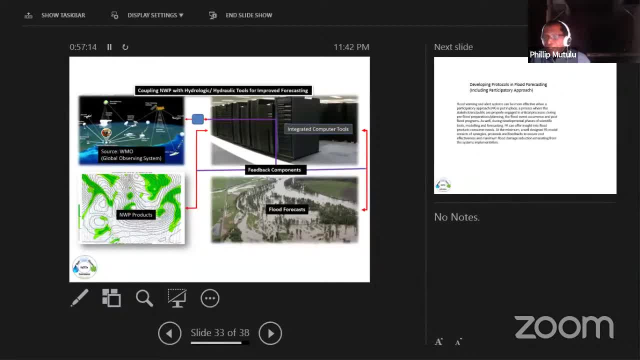 so that the data is streamed directly between the two systems: the numerical weather prediction models and the flood forecasting models. But these are not the only data exchanges that are taking place. The same flood forecasting model is also receiving data from the river level measurements. 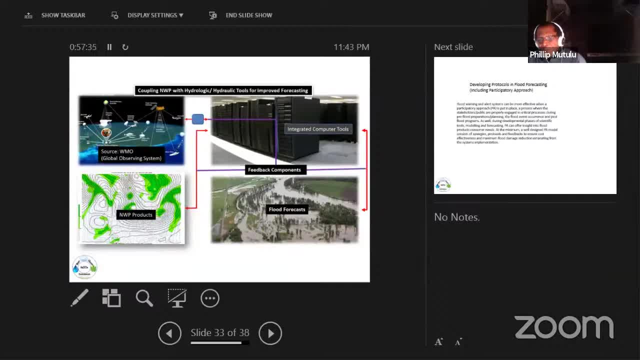 and also from the air-based airborne satellites and so on and so forth. So it's an integration of a lot of information And on that diagram there you see on the right-hand top, those are supercomputers, because it's not possible. 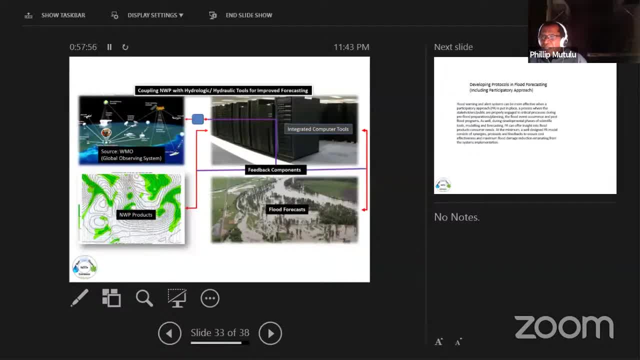 to do a forecast of weather or very advanced flood forecasting without those supercomputers. These are systems that are capable of computing trillions of data computation within just a millisecond. These are called supercomputers and they have actually to be cooled down. 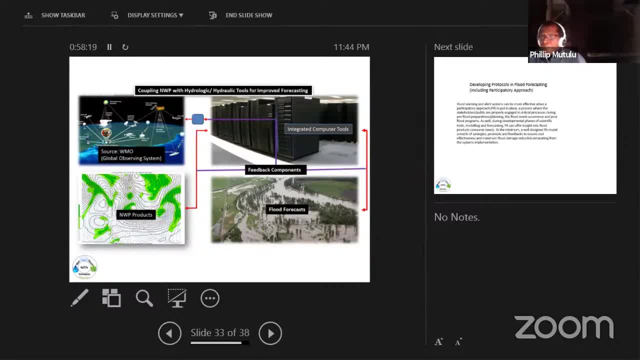 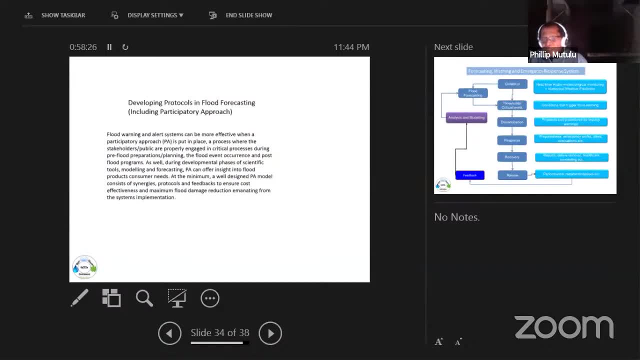 by cooling system because they are so huge. Now, one of the things is that, because of the complexity of flood forecasting, the future is looking at developing very well-defined protocols, And these protocols will ensure that nothing is missed out. no information is missed out. 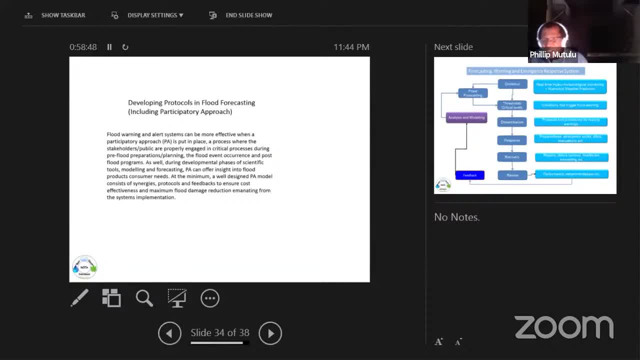 These good synergies feedback systems within the flood forecasting system. So the paragraph there reads: flood warning and alert systems can be more effective when a participatory approach is put in place, a process where the stakeholders- public- are properly engaged in critical processes. 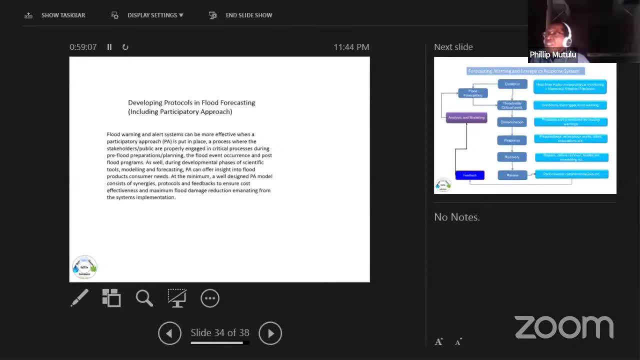 during pre-flood preparation and planning, the flood event, occurrence and post-flood programs, As well during developmental phases of scientific tools, modeling and forecasting. participatory approach can offer insight into flood products, consumer needs. At the minimum, a well-designed 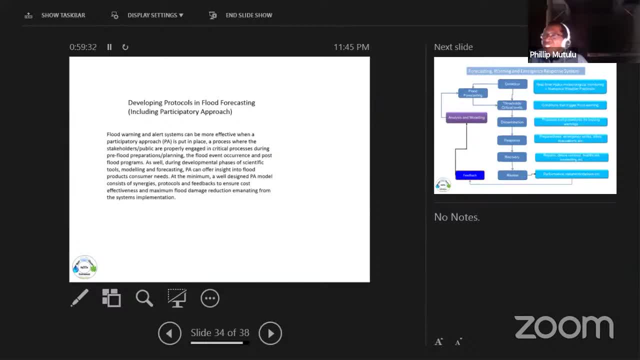 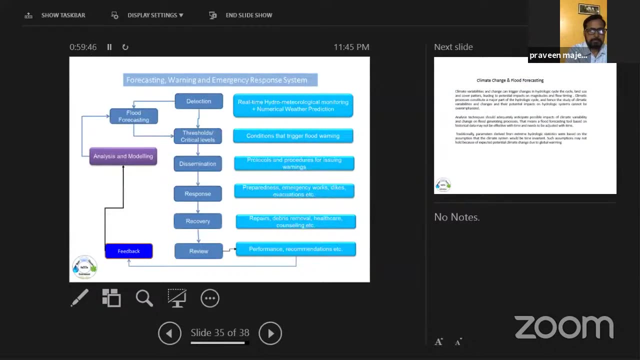 participatory approach model consists of synergies, protocols and feedbacks to ensure cost effective and maximum flood damage reduction emanating from the system's implementation. So this is what a simplified protocol should look like in a flood forecasting system. So right there on the 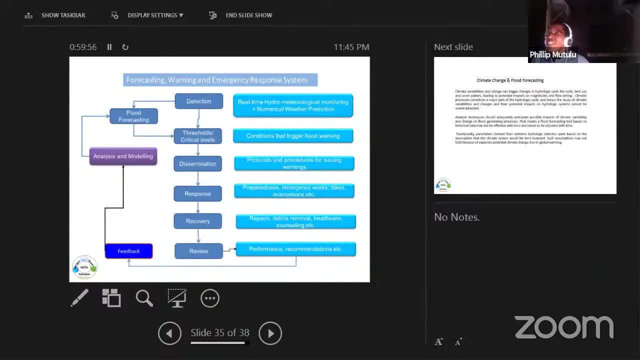 top left-hand side, you have the flood forecasting center. But now the flood forecasting center is not going to stand alone. It's going to be surrounded by a lot of stuff. There will be a detection. Detection involves a system which sends the signals. 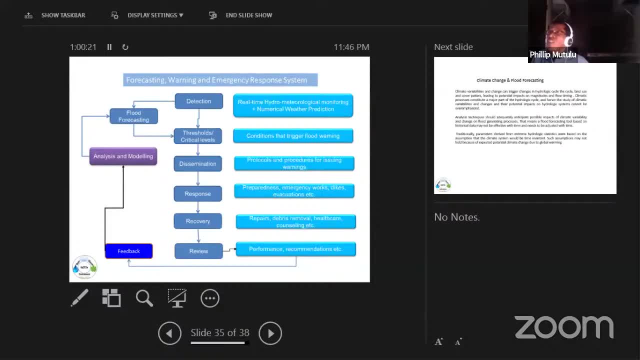 when we need to activate a flood focus system and is ready to trace old or critical levels. Also, critical levels involve the calculations of the time when we need to provide a forecast and so on, And so it's a complex system, But one of the things 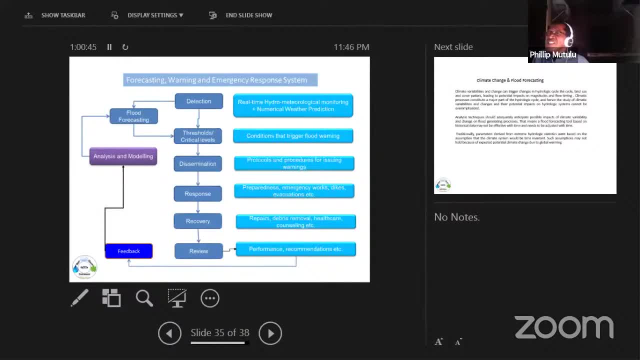 that I wanted to reiterate there. this system includes a response, component recovery, review, performance recommendations, repairs, preparedness and so on and so forth. It's a system that helps the flood forecaster to improve their system because they are getting feedback. 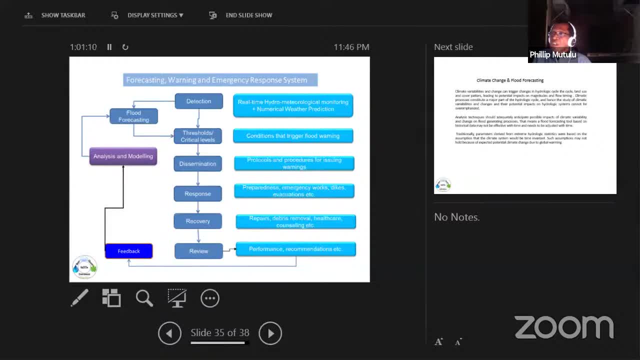 from different components, from outside of themselves, And that way they are able even to provide information that again, as I repeat, information that is tailored to the consumer and the right information And information that is understandable When you are providing a forecast. 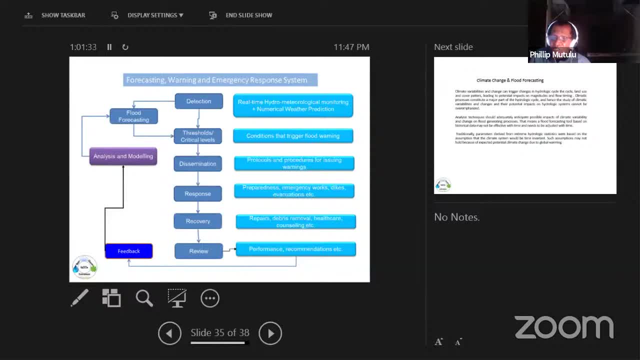 you are not going to start talking about mathematical jargons. You need these protocols, these synergies and feedbacks to let you know, no, you are not providing information that is consumable because you don't understand your mathematics. You need to simplify. 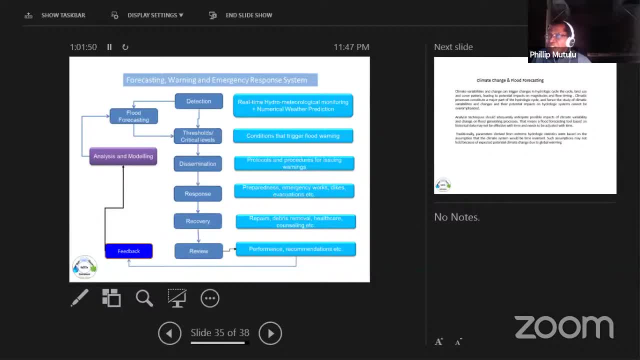 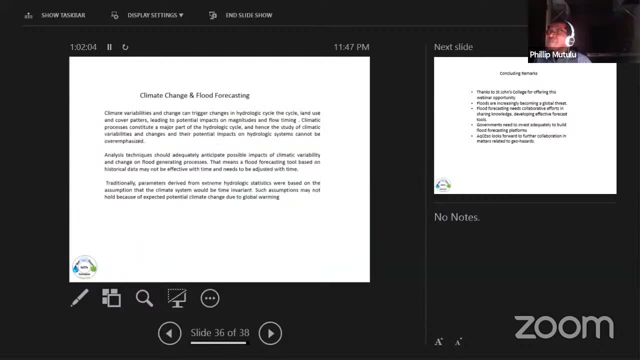 that information. So all this feedback will help us improve our forecasting system Again. this is a bit complex diagram, but when you go through it later on during your time, you will see it will make sense Now. so what have we seen? 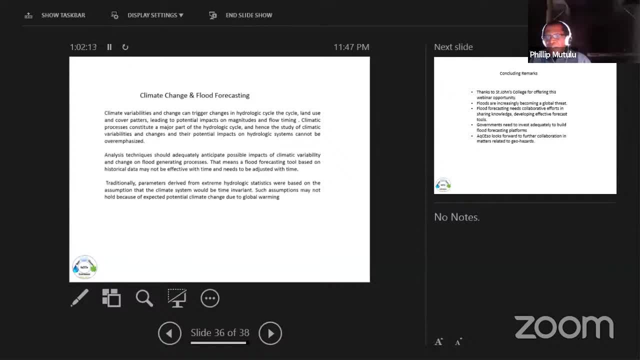 The previous slide was about linking different components in a flood forecasting system. that will be beneficial and eventually lead to reduced flood damage And proper response, and so on and so forth. Now the other challenge here is the climate change in flood forecasting- Climate variabilities. 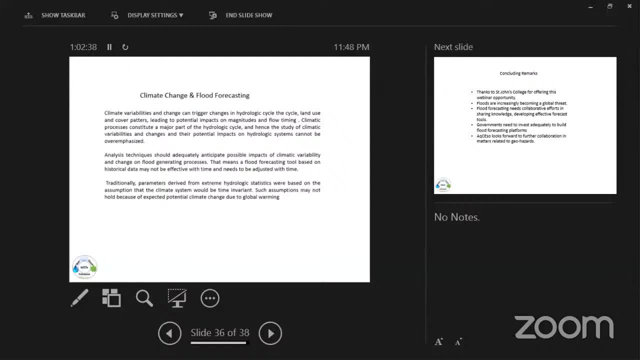 and change. When I talk about variability, normally this is a short-term variability. So you see, like a diurnal change, that's a variability. Diurnal change or weekly variability of a climate parameter, that is a variability, But a change is something that. 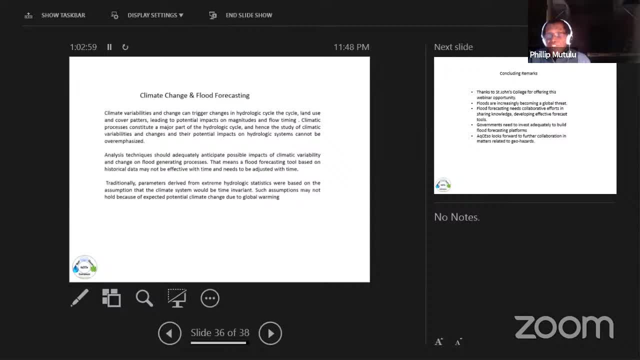 can be measured in terms of at least 30 years. That's when, then, you can start talking about change. Climate variabilities and change can trigger changes in hydrologic cycle, Land use and cover patterns, leading to potential impacts on magnitudes and flow timing. 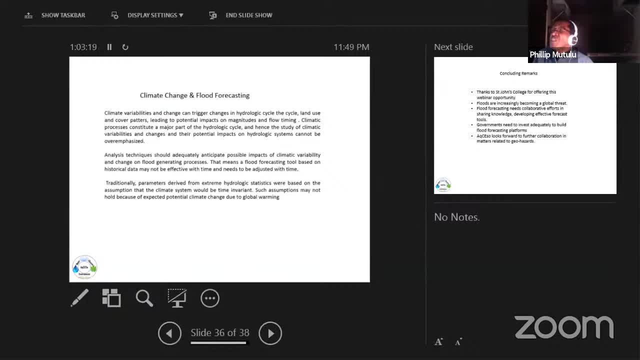 Climatic processes constitute a major part of hydrologic cycle, and hence the study of climatic variabilities and changes and their potential impact on hydrologic systems cannot be overemphasized. Analysis techniques should adequately anticipate possible impacts of climate variability and change on flood generating processes. 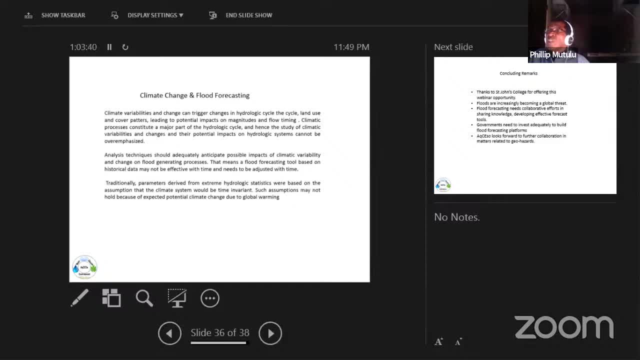 That means a flood forecasting tool based on historical data may not be effective with time, and it needs to be adjusted with time. Something that I would have talked about, but I didn't have time, is a model contains parameters, and these parameters are usually calibrated based on historical data. 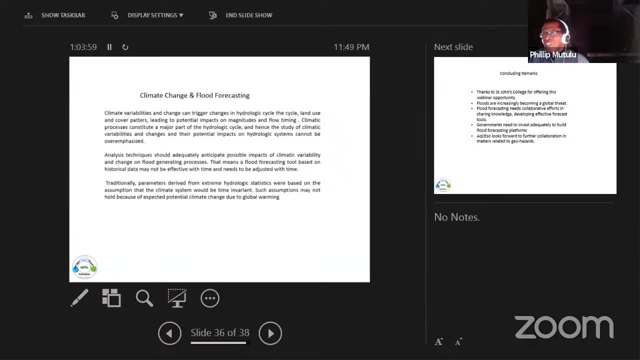 But if you are willing just to use historical data, that model may not work in future if there is a climate change effect in flooding, because the parameters will not reflect that, because they are based on historical data. That's why the current models have now to have the capacity. 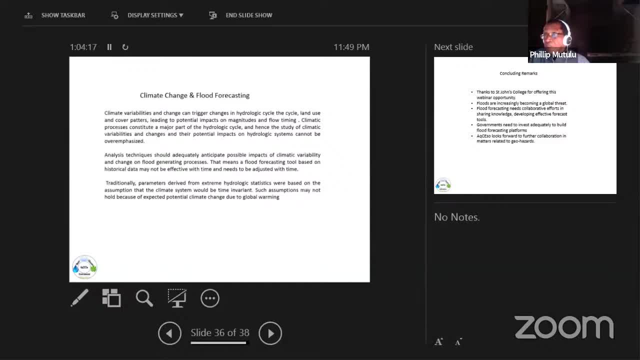 to adjust themselves to climate change. So you mean the current models have now to have the capacity to adjust themselves to climate change? Yeah, And therefore the models that we are using are kind of constructed to be able to do that, to be able to factor. 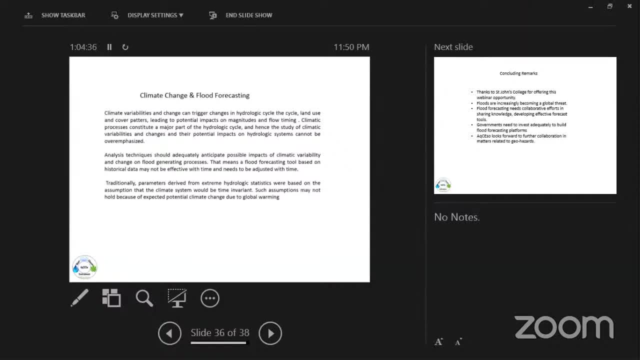 in climate changes. Traditionally, parameters derived from extreme hydrologic statistics were based on assumption that the climate system would be time invariant. A climate system that is time invariant is a system where the mean, for instance the average conditions will not change. But now, with climate change, 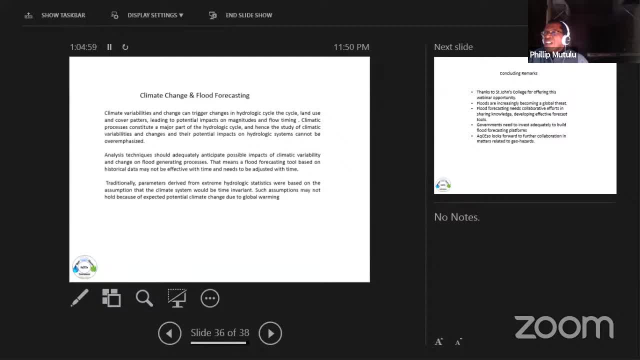 those are going to change and therefore the system is no longer time invariant, but it's now varying with time. It's a non-stationary system, So assumption of stationarity or time invariant may not hold because of expected potential climate change due to global warming. 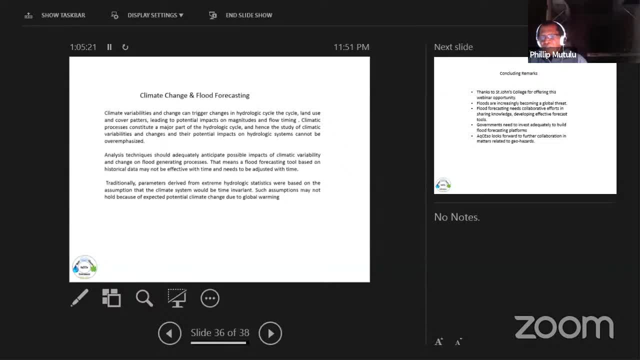 And so some of the things we are doing here is to adjust flood forecasting models. if we are expecting temperature to change by this March, in the next 30 years, How should we adjust our model? Because, by the way, a flood forecasting model is not just used. 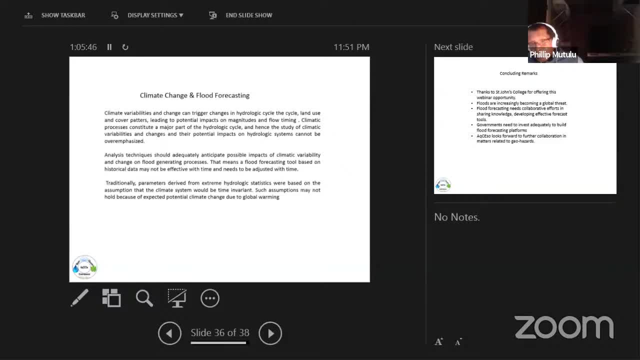 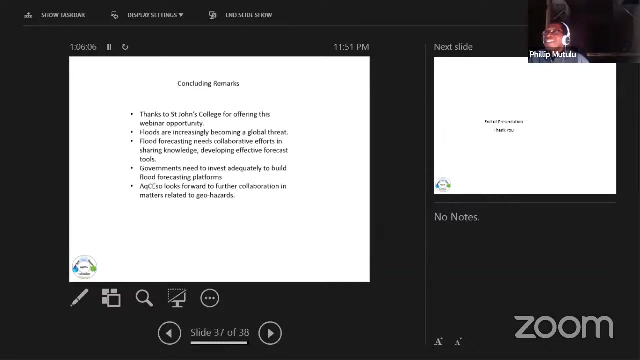 for short-term forecasting, but they are also being used for long-term forecast, so that you can also have long-term planning. That's why we need forecast models that take account of potential climate changes. So, after my long story, I want to conclude, and we 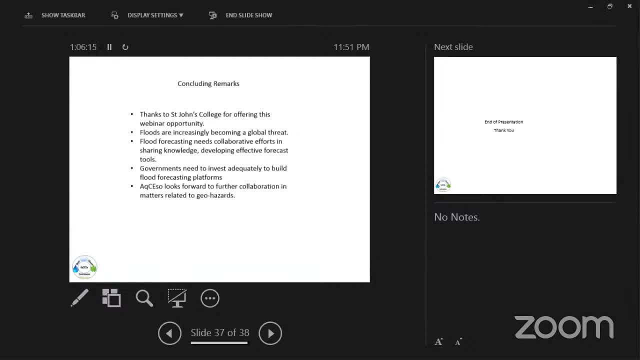 have looked at the examples of damages that are caused by flood forecasting models. We have looked at the hydrologic cycle as basic knowledge that you need to develop your models. We have looked at chaotic nature of models and their uncertainties. We have looked at the need. 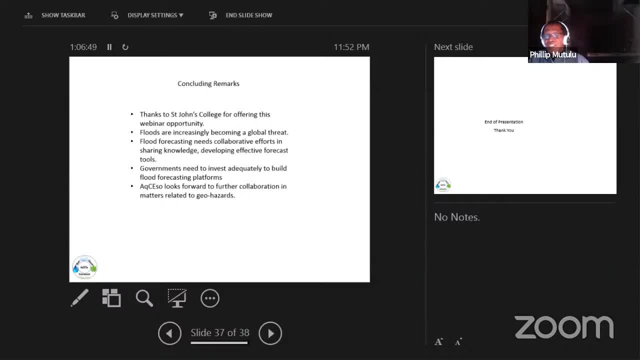 to collaborate between different agencies, and we have also looked at the problem of climate change. In conclusion, I want to thank you for offering me this opportunity. We see that floods are increasing and becoming a global threat. Flood forecasting needs collaborative effort in sharing knowledge. 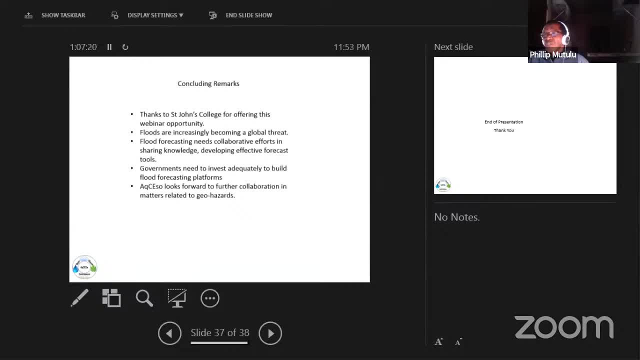 and developing effective strategies to address climate change. I believe today we have seen flood forecasting is a very wide subject. Sometimes you might have thought it is a very narrow bounded discipline, but it is not. It is a conglomeration of a wide range. 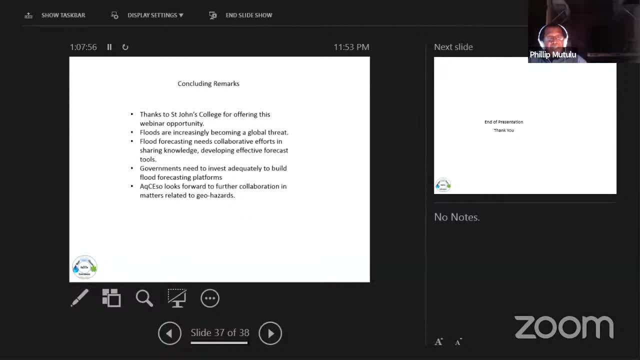 of factors that affect flood forecasting. It is a very complex system and it is a very complex system. It is a very complex system and you can develop and evaluate flood forecasting models and so on and so forth. It is an area which integrates different knowledge. 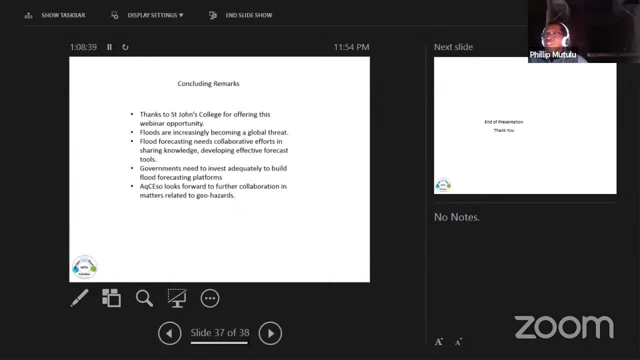 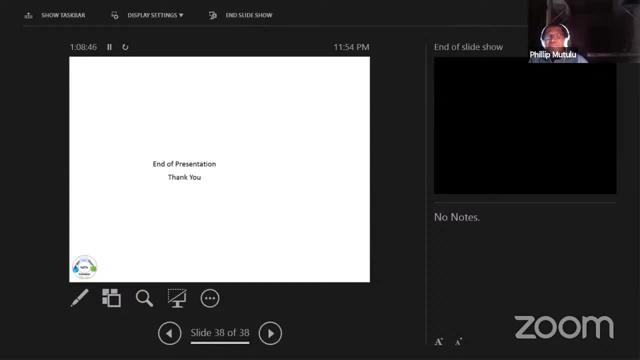 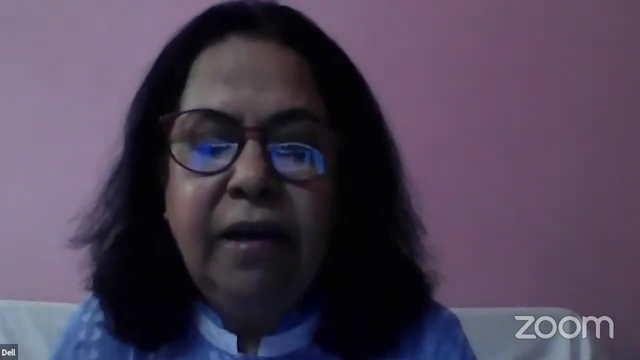 and expertise, so different professionals are useful in forming a part of flood forecasting. Thank you, sir. Thank you, Dr Philip. You have touched upon flood forecasting from you, have looked upon it from every detail and have given us a very exhaustive and detailed view of 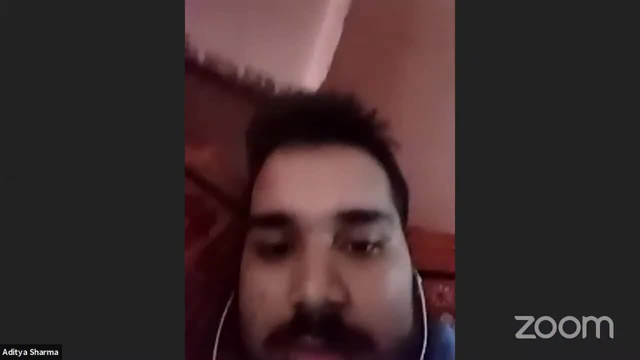 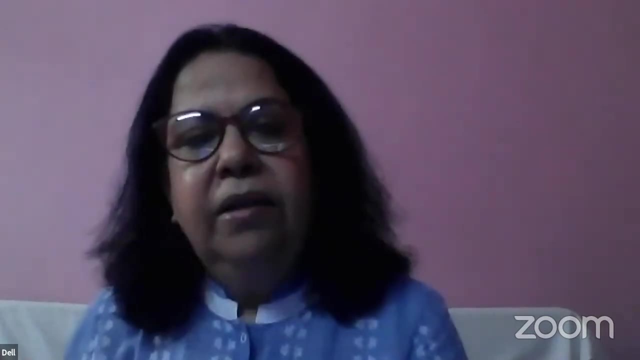 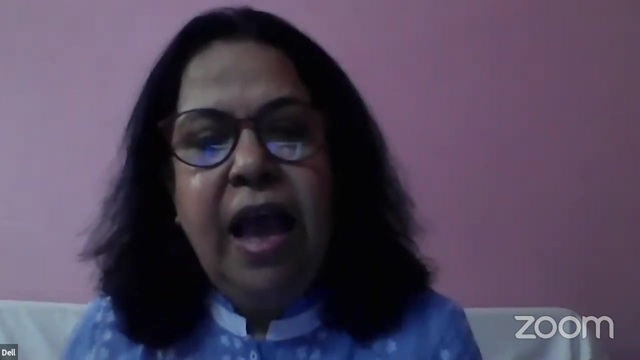 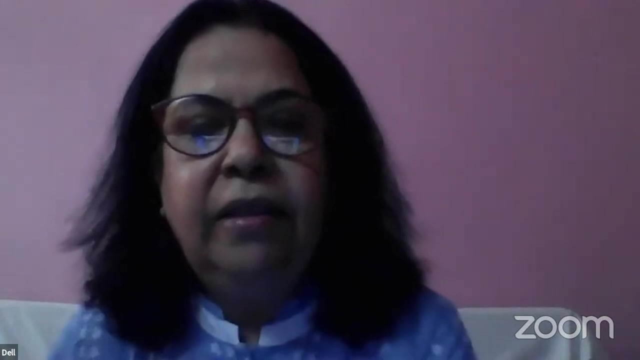 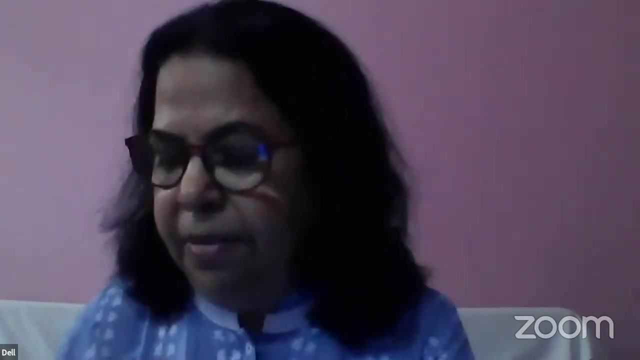 flood forecasting The tech team. can you please put me on the screen? Dr Muthulu, you picked your objectives from the scriptures and here in India, as well as globally, when we are facing the locus, the pandemic, the flood is a very powerful tool and 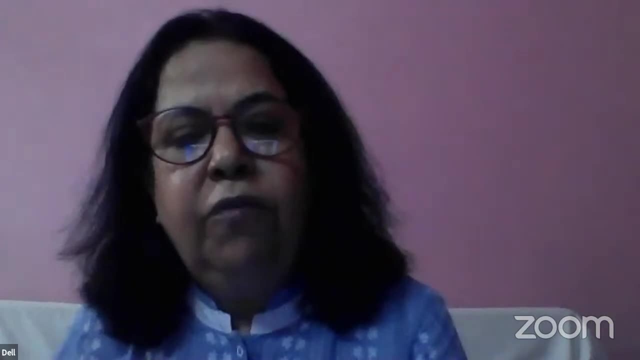 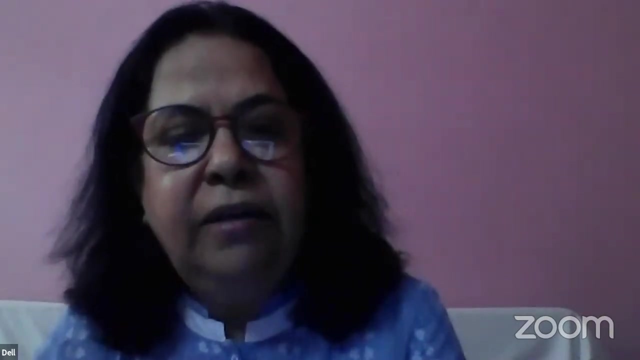 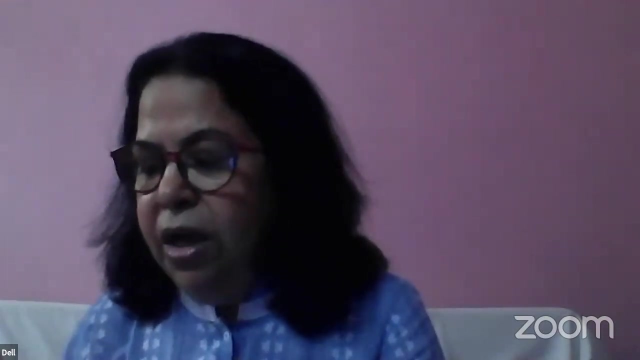 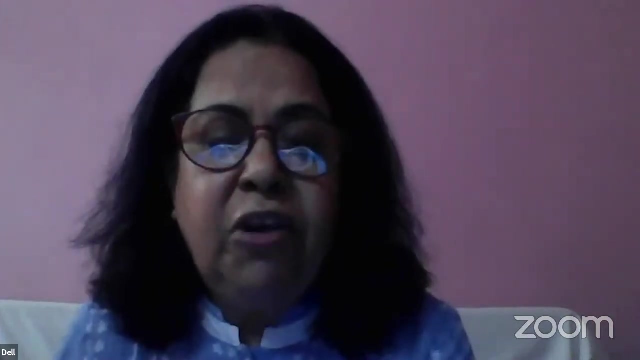 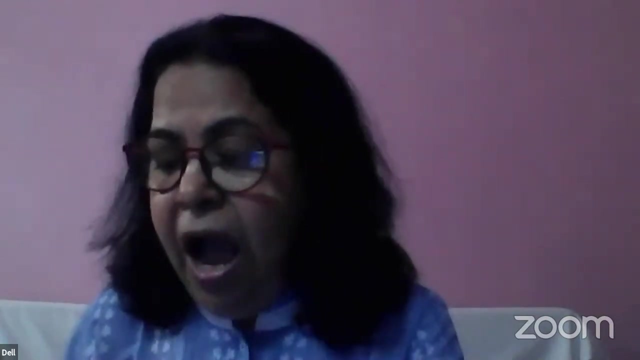 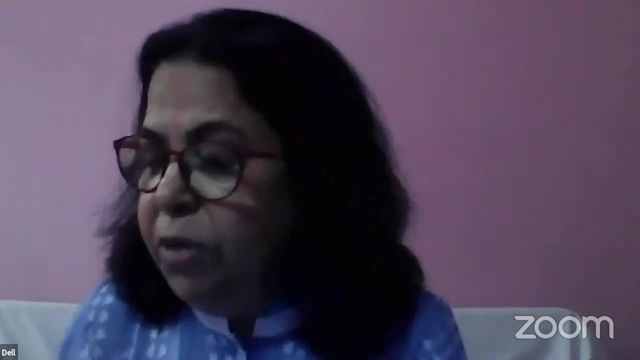 it reminds us all that is written in the bible. You also explained the hydrological cycle- for the ones who are not familiar with the recent flood situations, especially the floods in Australia, the severity and the frequency of floods and how conducting data analysis, modeling and forecasting, and what 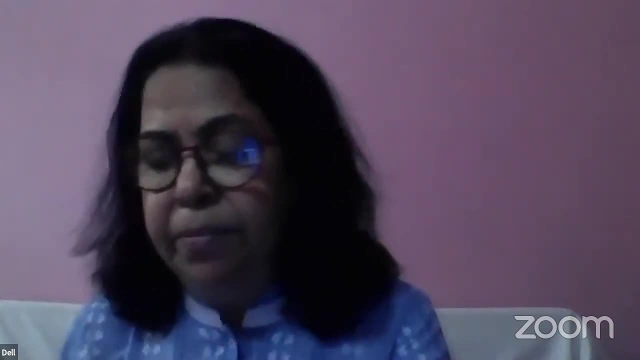 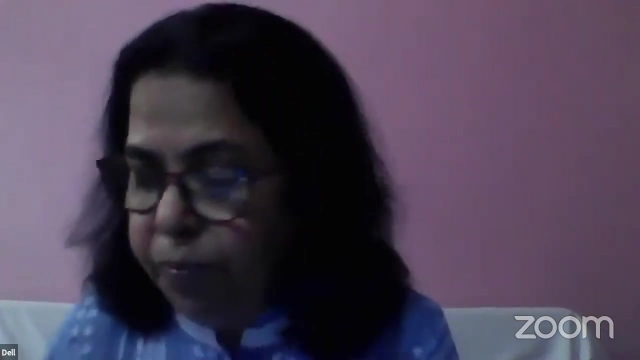 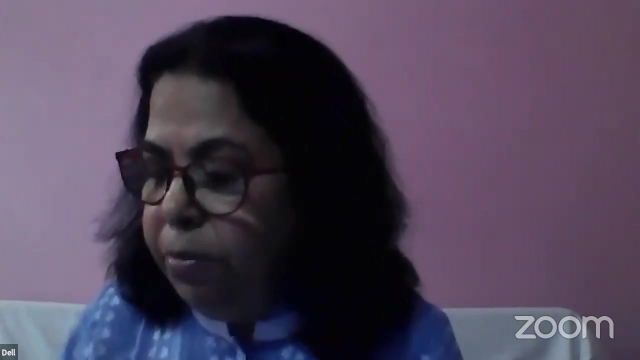 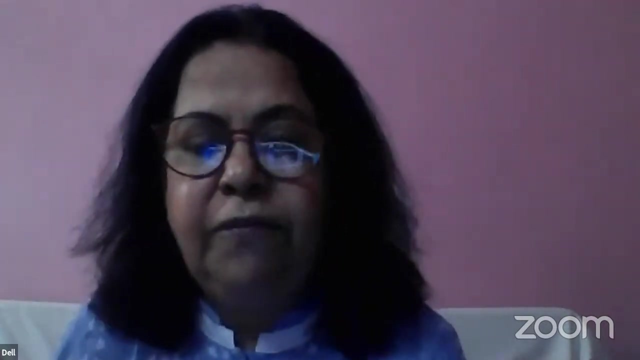 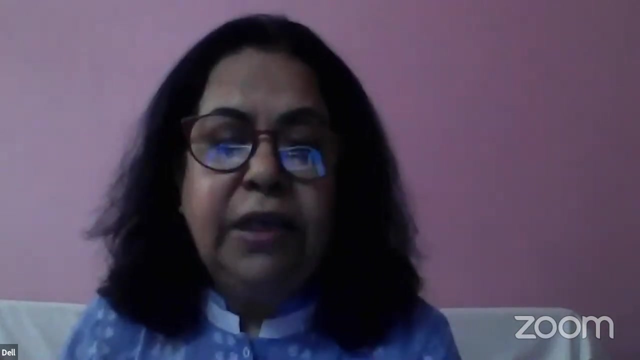 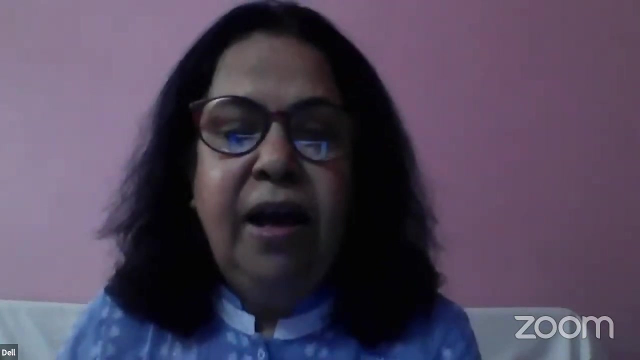 are the missions of flood forecasting centers, both for the science and arts background, people that with informed, along with flood analysis, informed instincts and social judgments, can save so many lives and biospheres, with both the combination of arts and technology and the natural environment, and the environment and 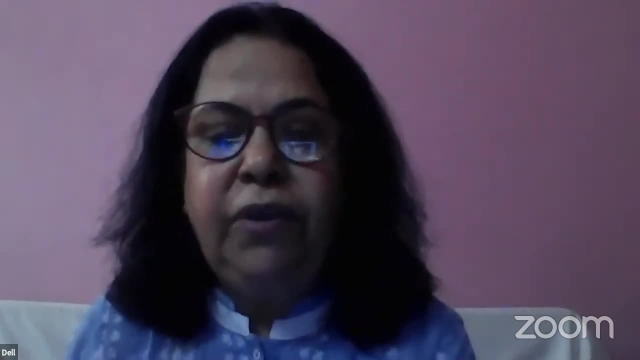 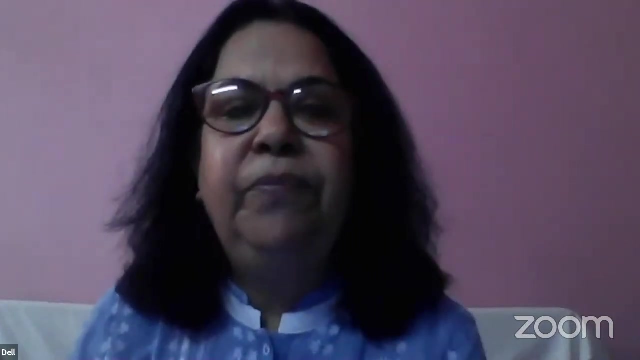 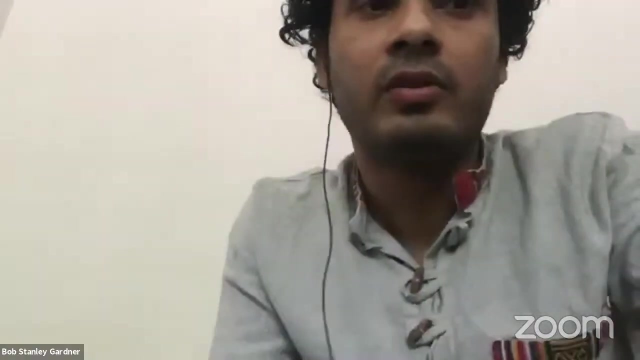 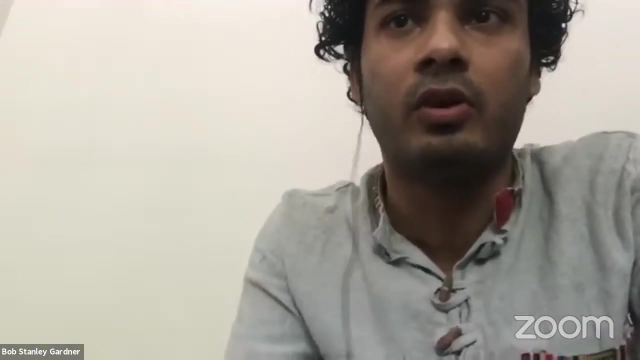 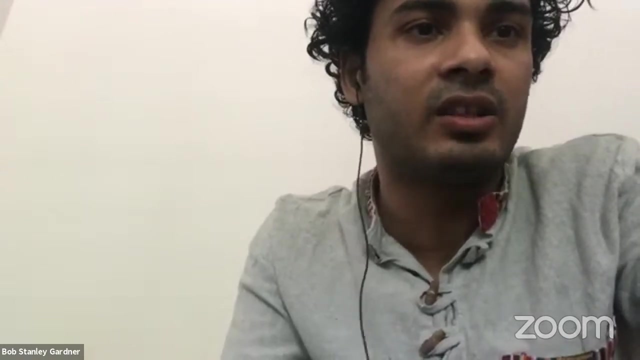 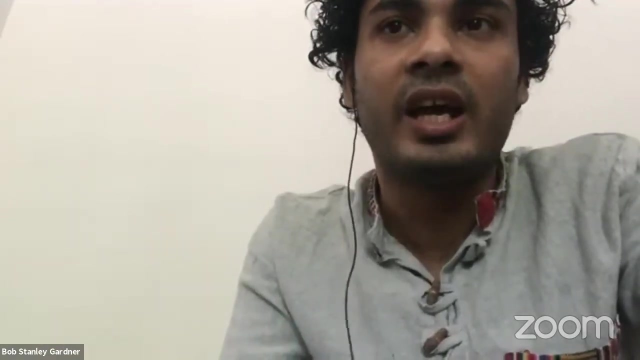 the environment and the environment. so these are the things that can be used in the future and in the future. so I have some questions. one is that you were talking about formulating a model for flood modeling, right? so I have read some studies and whenever we are 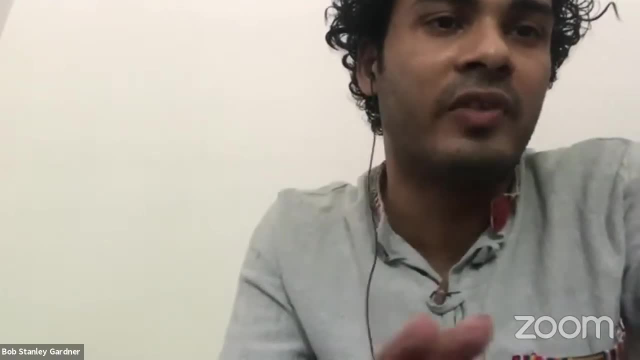 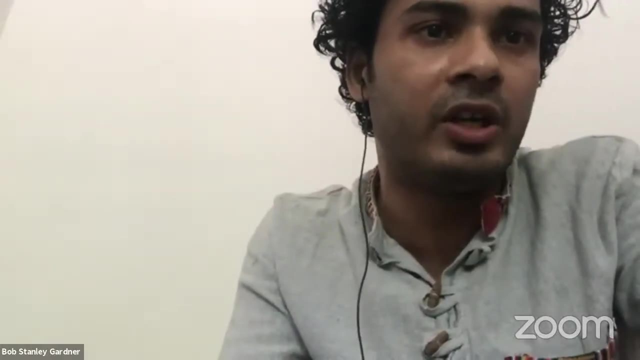 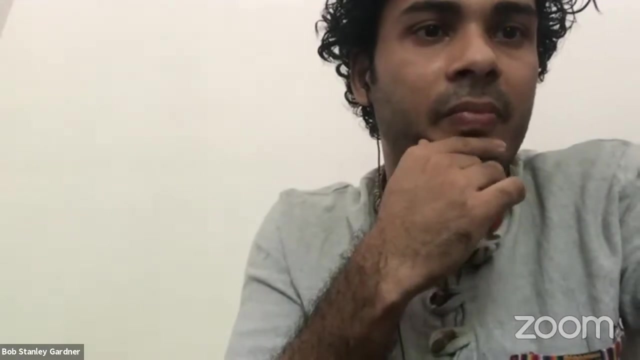 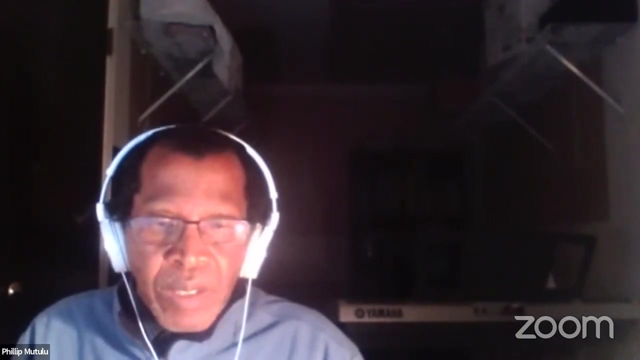 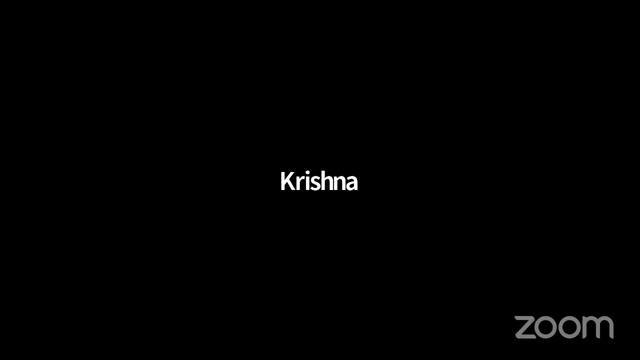 considering modeling, flood modeling and its mitigation. so do you think weightage should be given to social and institutional factors also when we are talking about mitigation? yeah, perhaps then you are familiar with the conceptual approach to building model. the conceptual approach brings in other areas I agree with. 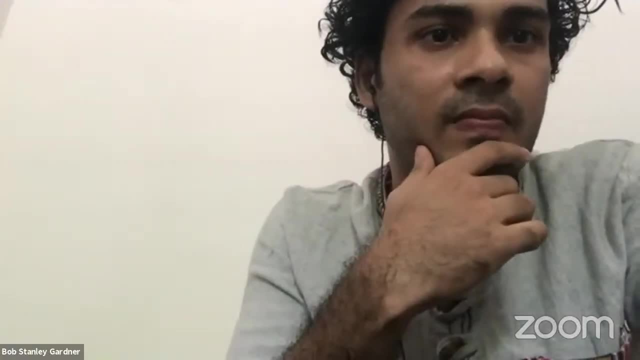 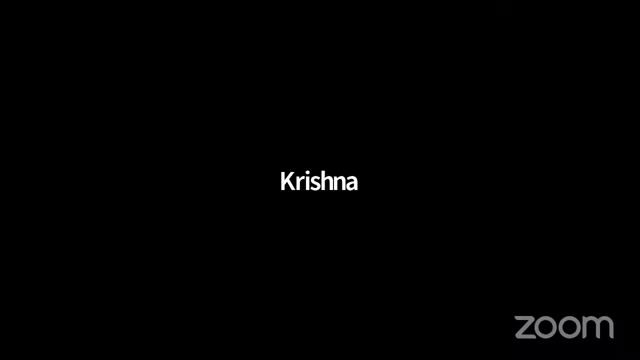 you. yes, sir, put your mic on, please. can you mute your mics? participants, please mute your mics. and I request, sir, please unmute your mic. sir, you are muted, you have to unmute yourself. so am i good now? yes, yes, okay, okay, yeah. what i'm saying is that 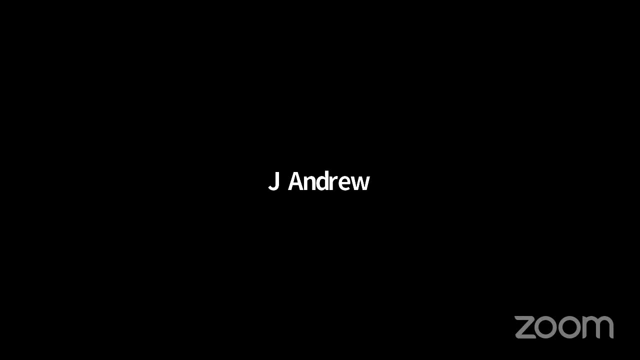 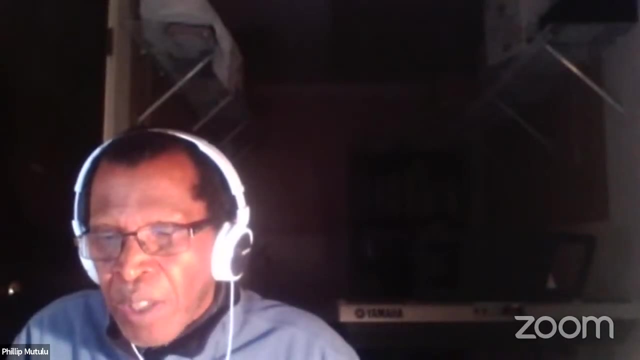 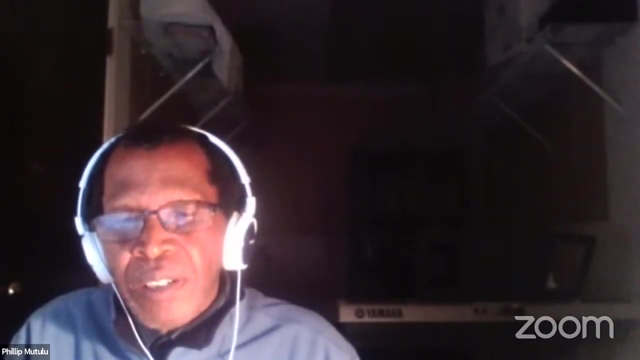 the approach today is called concept modeling, where you bring groups of different people together and then every group comes with a component and these components are put together to form what is a conceptual flat forecasting model, and therefore this involves sociologists, response health practitioners, mathematicians, economists and so on. it's a very complex approach. 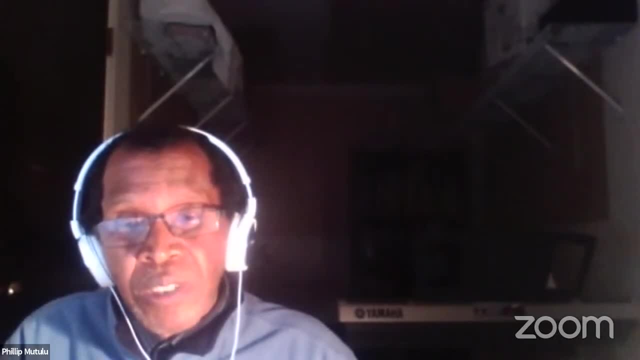 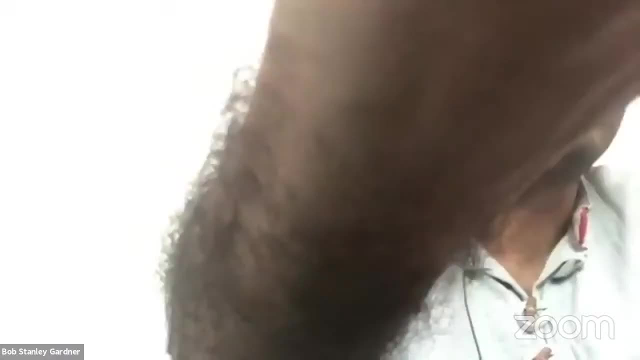 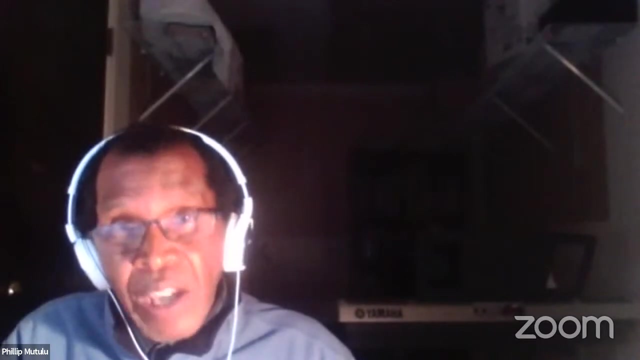 but i think it's an approach that we cannot avoid, because the ultimate goal of flood forecasting and mitigation is to save lives and we cannot just save lives by mathematics alone and physics- no, uh, we need to know human behavior and response to floods and how do they conceptualize risk, flooding and that kind of stuff. so actually you find that in: 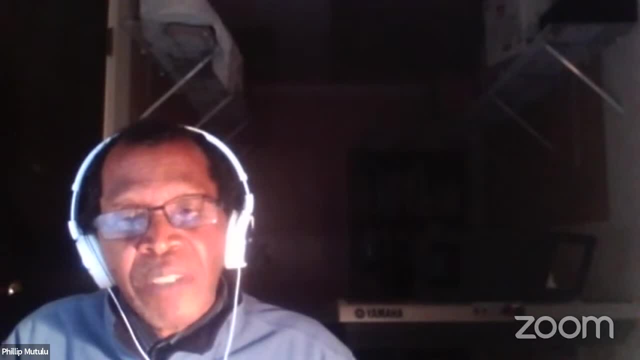 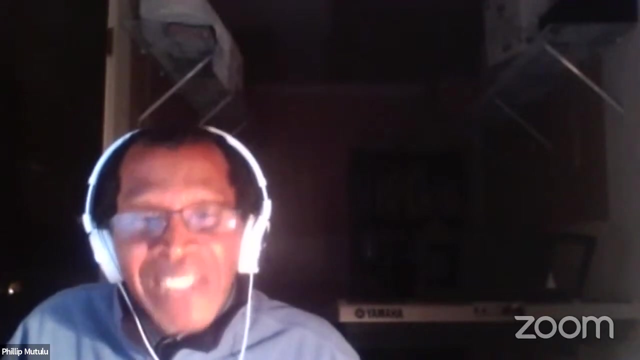 the subject of flood risk, there is something called cognitive studies, where you know, you study the behavior or the behavior of a human being in terms of, conceptually, what does he think a flood is? how far can he remember? does he think a flood is going to happen soon? and, using his mind, he can say: i think there's going to be a risk. 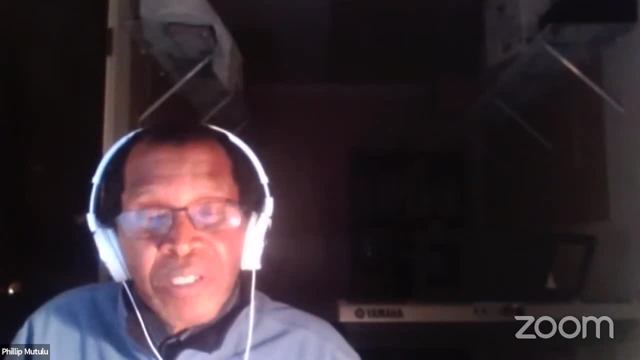 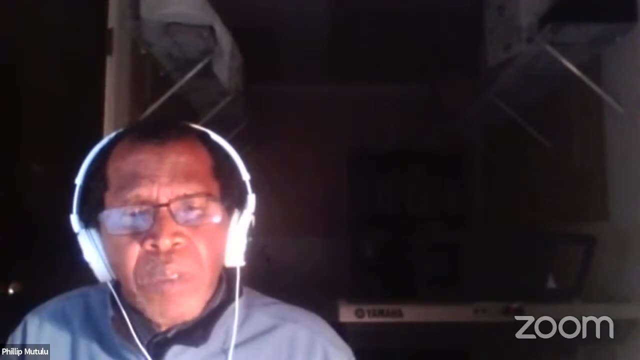 of high flood this year. and why does he think so? because you know, in his thinking it does this already inbuilt cognitive uh process that can be used to provide a focus. i remember my grandfather, my before he died. he actually used to focus weather very accurately. i would say um, and it would just be observational. 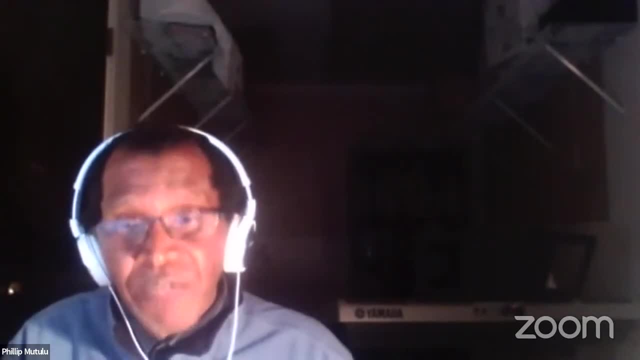 from his past experience, even from feelings, his body feelings, he could tell it was to rain in two months, and so on and so forth. so this is a process that we can use to provide a focus, and i think there are a lot of traditional knowledges even that are being incorporated into this model. 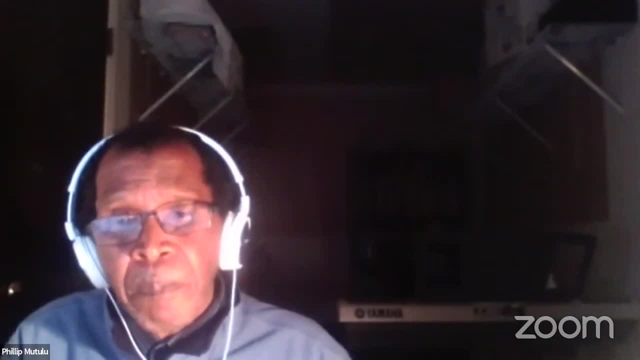 indigenous people, in fact, now are becoming a big part and parcel of these systems. they are being invited to conferences to provide, to give purpose, on what is the best way. for instance, do you think we should manage lands to be able to avoid flooding? yeah, so these things are, you know they? 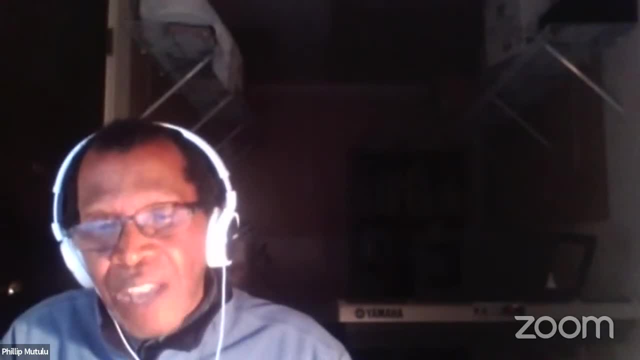 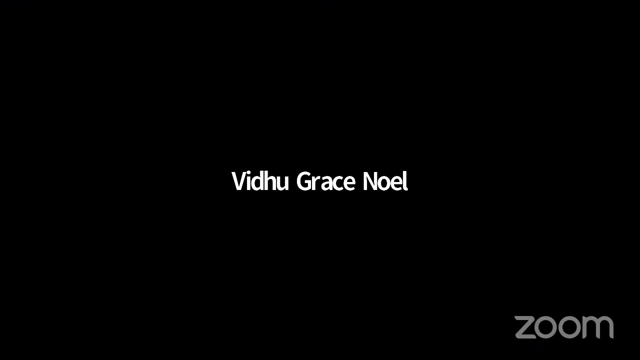 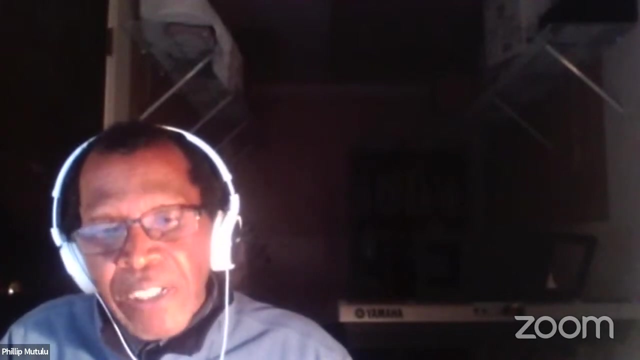 are picking up speed every corner and i said the ultimate goal is to prevent damage, to minimize damage and to be sure that we are providing specific information to people that need that information, and that information must be provided in a way that those people can understand in simple terms and can effectively apply that. 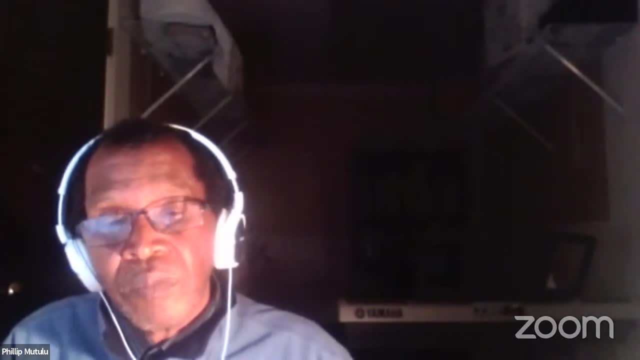 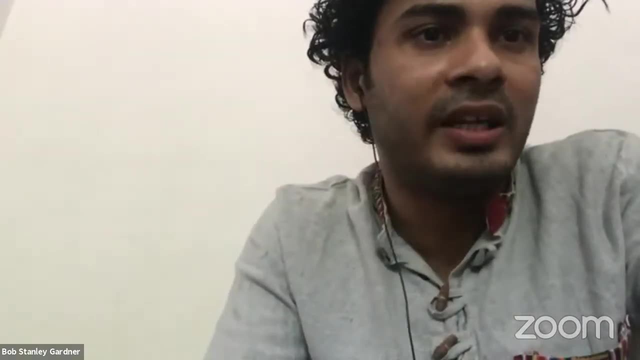 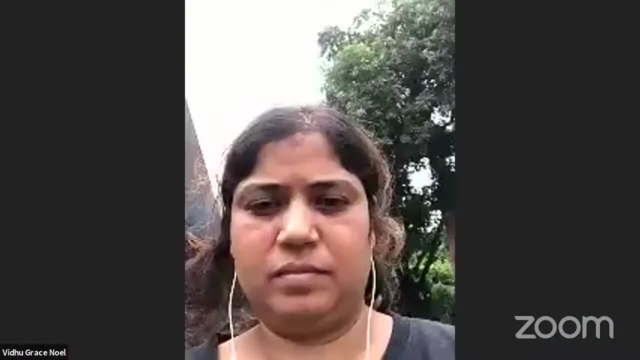 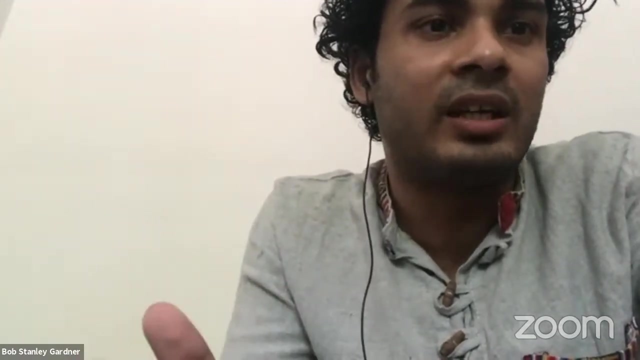 information. okay, so, uh, i i had one question, uh that, uh, when we are talking about the probabilities and when we are talking about predictions, then that means we are going into inferential statistics. so i just want to quickly uh, if you can just guide me through that, uh, what should be the assessment that we should look upon, like when? 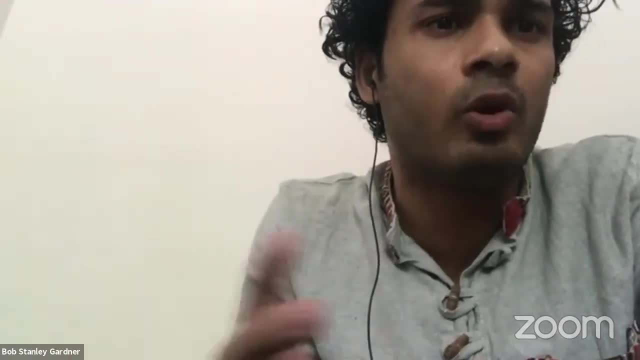 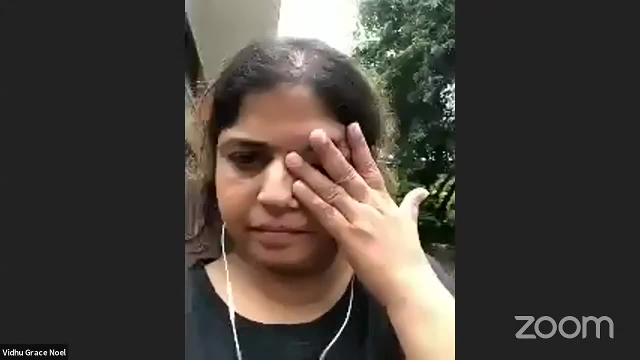 we are going for probabilities. what are the percentages we are? i know nowadays it's all done in softwares. we are using swat and gis and all those softwares. it's majorly done in softwares. so i just wanted to quickly, uh, if you can just guide me through, what should we? 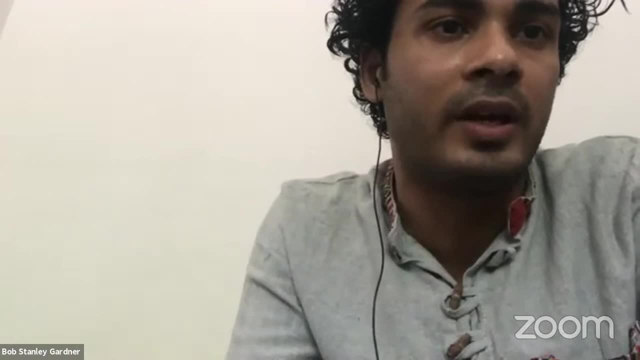 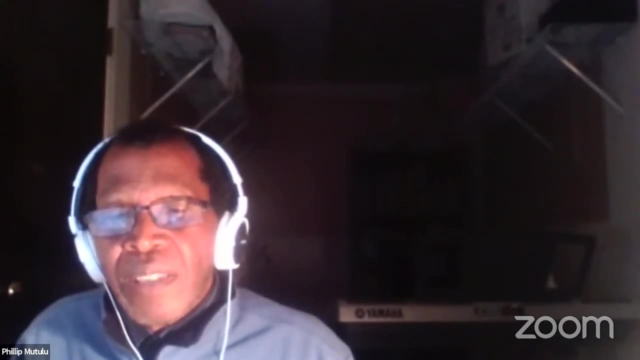 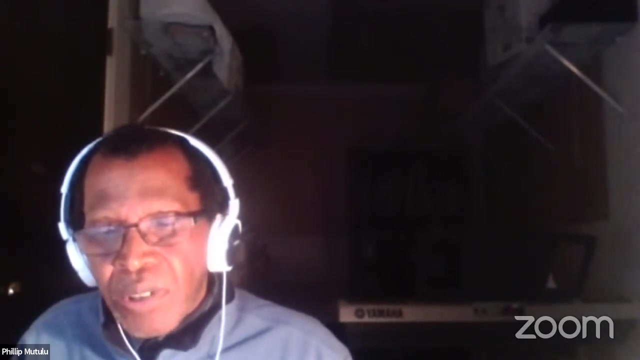 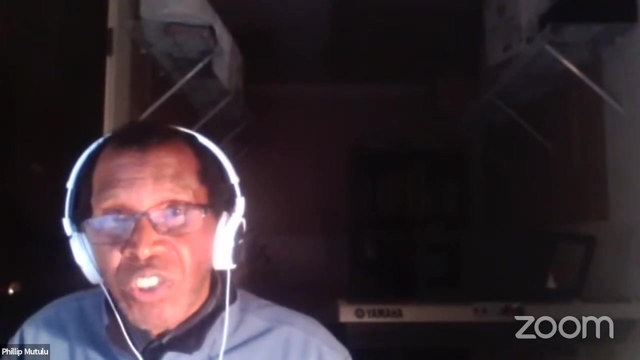 be looking upon when we are developing statistical probabilities. there are different things. one way of building a stochastic model is to look at time sequence of rainfall runoff data and you can look at this time sequence and determine how the mean or standard deviation is changing with time and you can use the mean and standard deviation as your predictors for future. 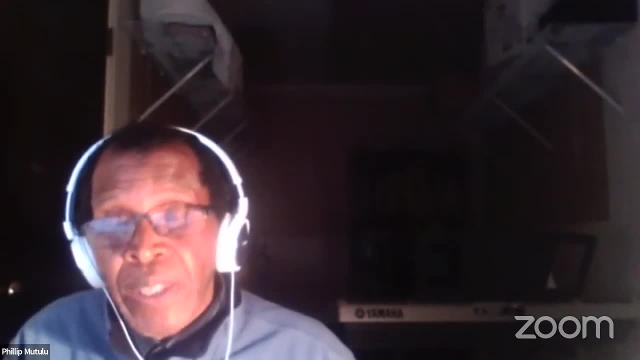 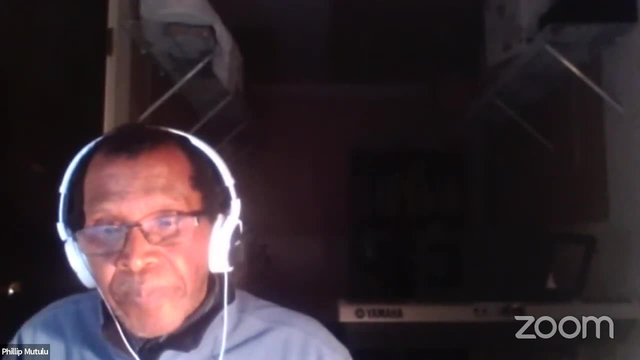 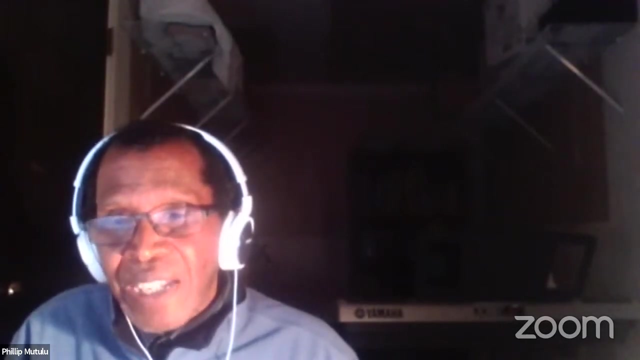 that's an example of a probabilistic model. another example of a probabilistic model is looking at the frequency of big events. you can look at data and do analysis to determine this magnitude of flood- when is it again likely to occur in future? and you can factor this information into your flood forecasting model, your flood forecasting. 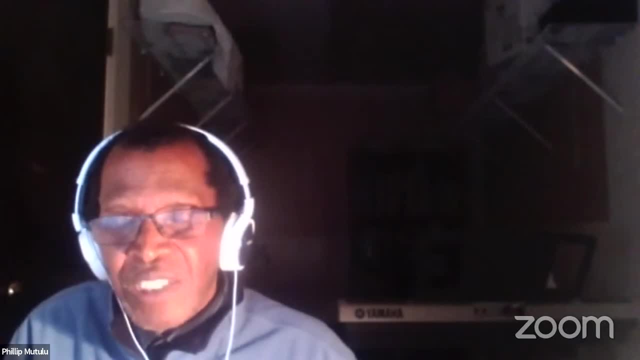 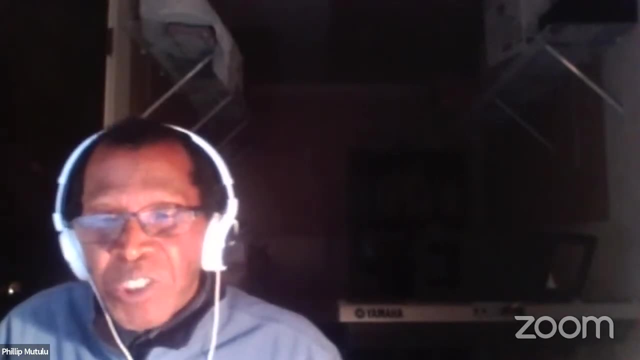 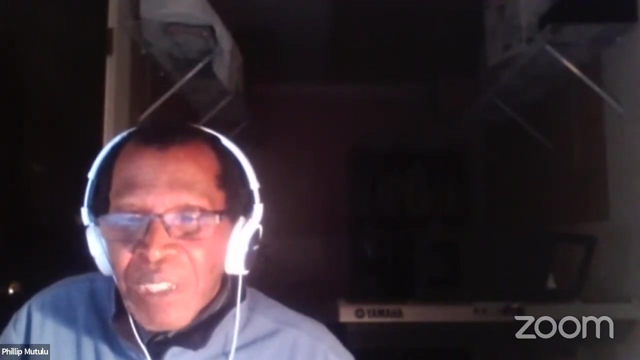 model uh in the physics one. the physics base will just tell you: oh, i'm using this equation, this physical equation, because i know loss of motion. will tell me that the the water that come in there are similar. the level of the water that comes in, some of it evaporates, another one some. 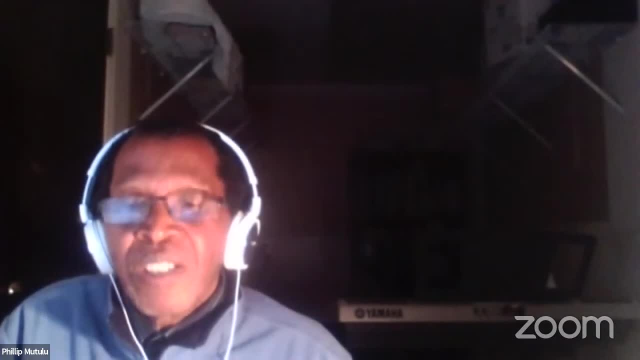 other component in. if it gets, what is left is the runoff. so i'm going to use those runoff equations to produce my flood magnitude. so that's what i can. uh, a physically based model will tell you, but the probability models will basically depend on historical data and just calculate. 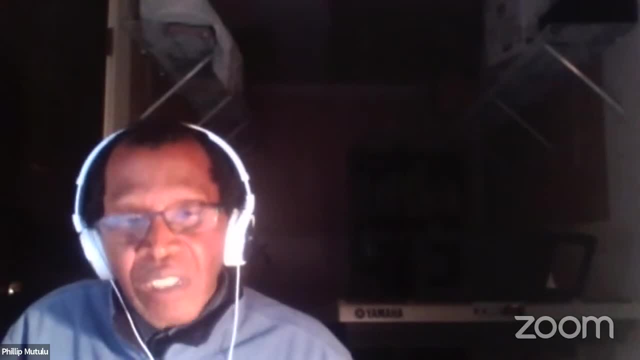 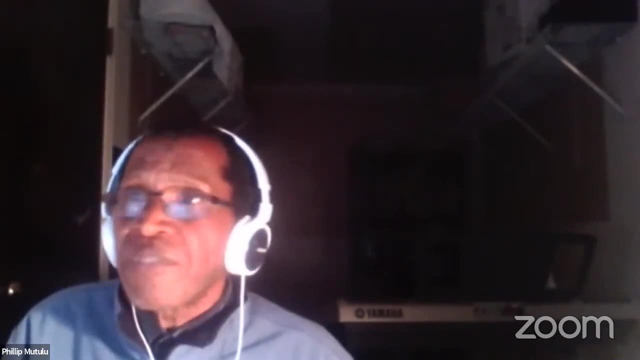 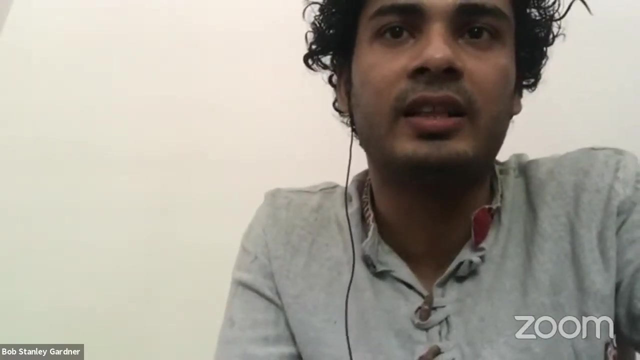 parameters like mean, standard deviation and so on, so that they can be calculated based on data that they are given to them can focus for the future. um, yeah, if you want, i can send you some some references that you can look at. yeah, so i'll contact you regarding that. uh, if i'm allowed to ask one more question, 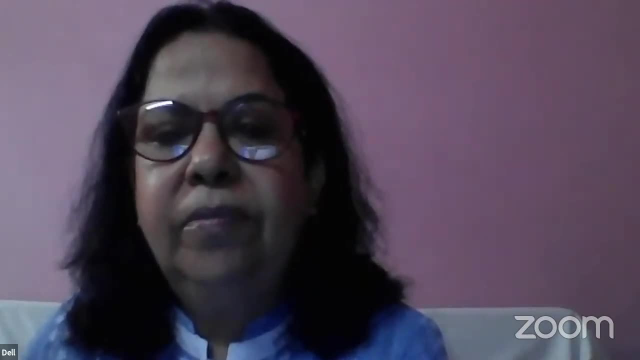 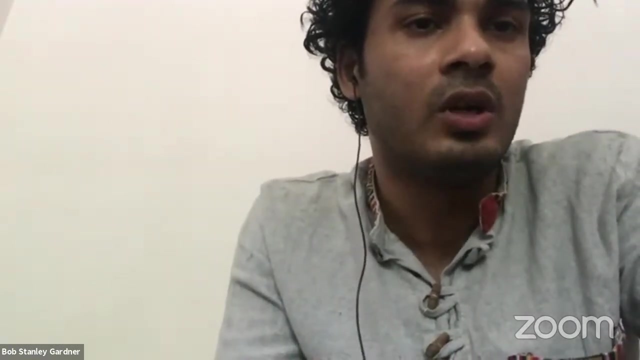 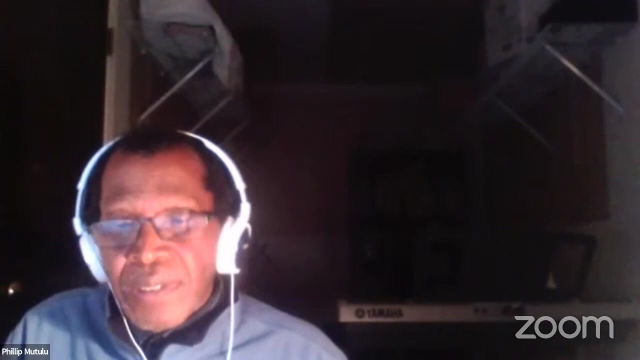 yes, yes, please, yeah, okay. so, uh, we were also talking about uh land use, so i just want to ask that: what are the parameters that we are looking into when we are assessing land use? uh, land use. um, you can look at land use from two perspectives. the first one: land use can also refer to land cover. 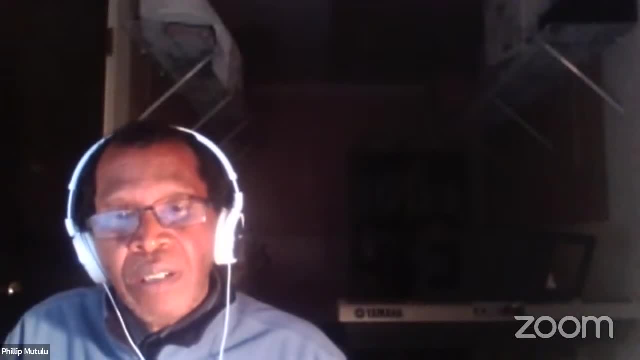 so land cover can be a particular type of soil or vegetation and this type of soil has got some particular infiltration characteristics, while the plants they have particular characteristics of evapotranspiration. so if you know the type of soil and the type of plant that is in a particular area, 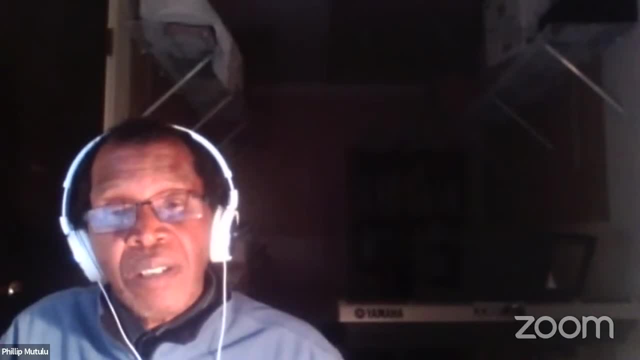 then you can use mathematical equations to calculate how much water for this plant is lost to the soil in the environment and the soil熱ting is lost through infiltration. for example, if the rain sanc is lost through infiltration through those soils, or all much is evaporated into the atmosphere, um, or if the land has been stripped of vegetation and maybe 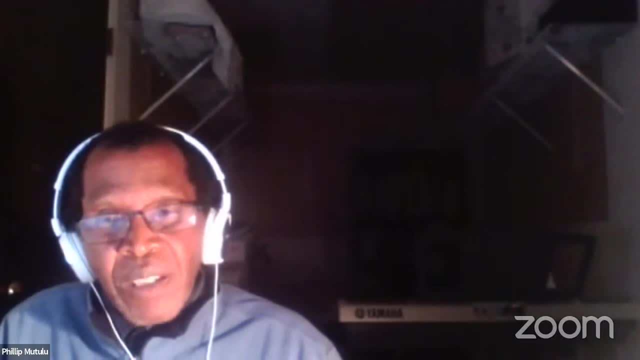 it has been paved, uh, with, you know, hard termic, then no, what is going to in in, if is going to run off, is going to form a flood, apart from little evaporation. but, by the way, evaporation is not a very critical factor during floods, because floods happen very quickly unless you are looking at long-term soil moisture variations. evaporation does not really matter for short-term uh forecast, but when you are doing long-term tracking of soil moisture, they do tell us: okay, our soil moisture, because of evaporation, it is experiencing moisture deficits. so if we get 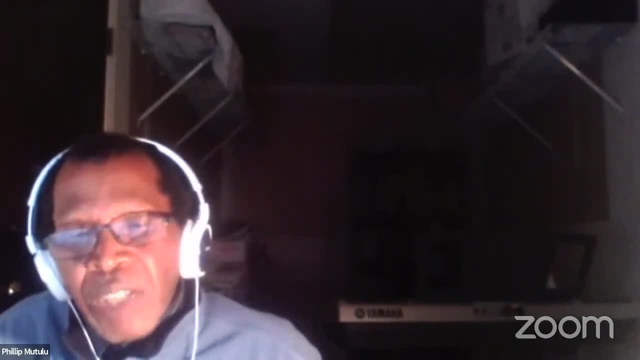 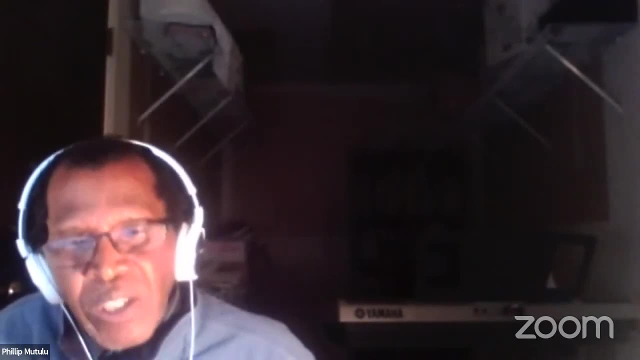 amount of rainfall of this amount, then we are not going to get a flood. but if there's a lot of soil moisture already, a lot of moisture in the soil, then if we get this amount of rainfall we are going to get this amount of flood coming from this type of land use. so land use mainly is infiltration. 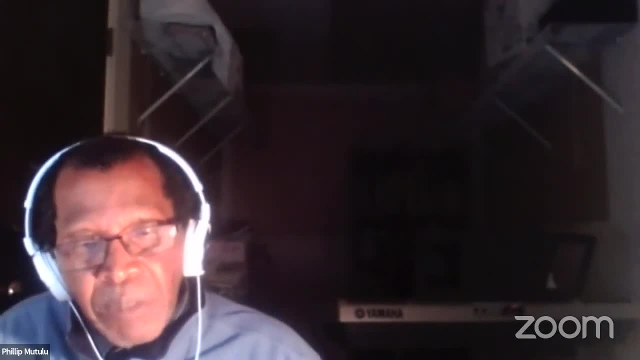 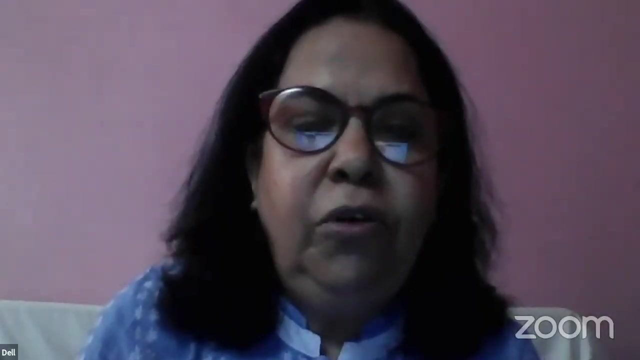 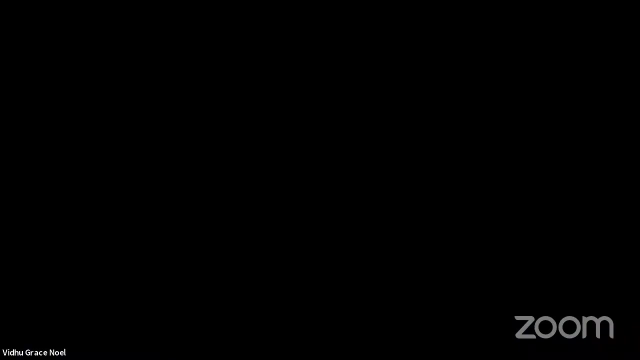 slope and cover, and sometimes on long term, which considers evapotranspiration. over to you, ma'am. there is, if dr muthulu will allow, there is time for one more question, if anybody has, dr mahima. yes, ma'am, ma'am, i have one question. yes, yes, dr vidhu. 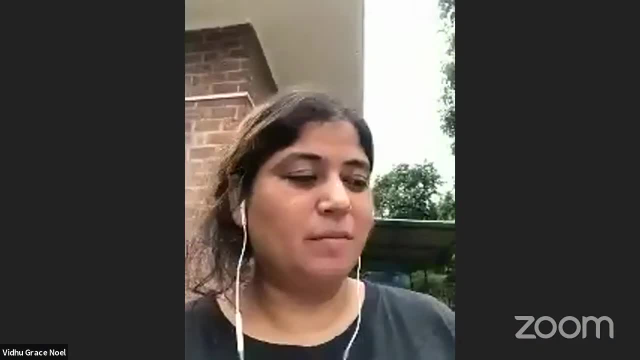 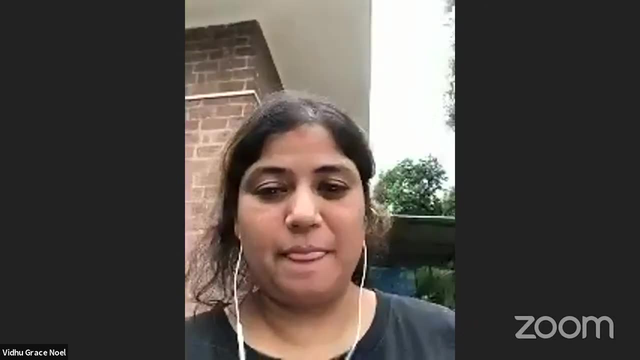 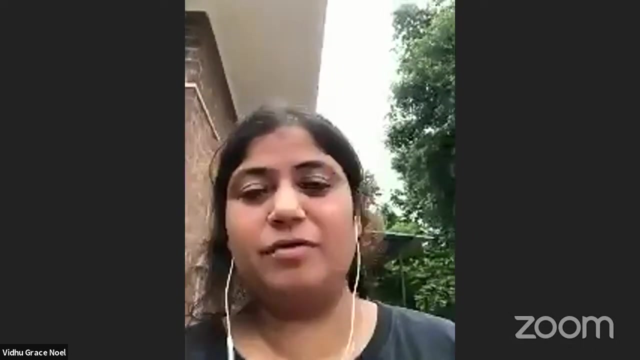 thank you, ma'am. ma'am, a question has come up that what is the meaning of 100 year flood and how is it used in flood forecasting? a student has asked: what is the meaning of 100 year flood and how is it used in flood forecasting? yeah, a hundred year flood, for instance, would mean. a flood with a magnitude that, on average, would occur after every. But it doesn't mean that if a flood of maybe 500 cubic feet per second occurs today, it will occur again after 100 years. No, it is not. It is not going to mean that It is an average number of how frequent such a magnitude occurs. 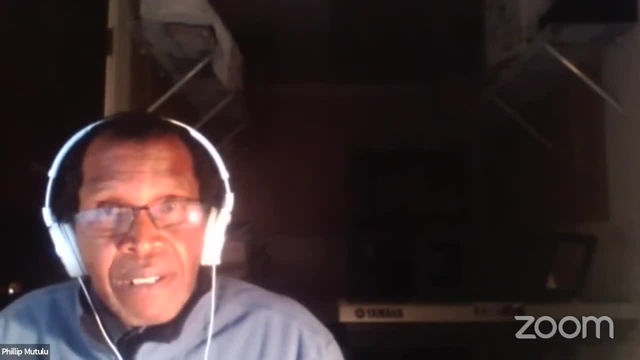 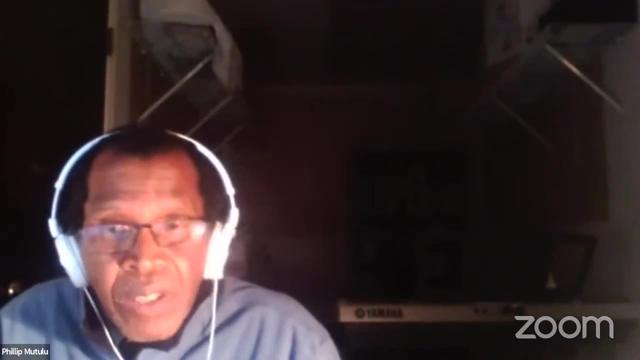 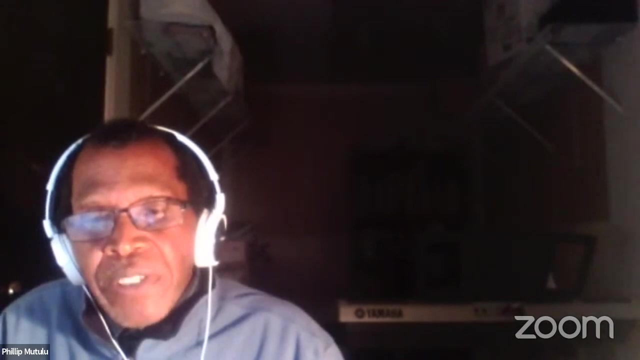 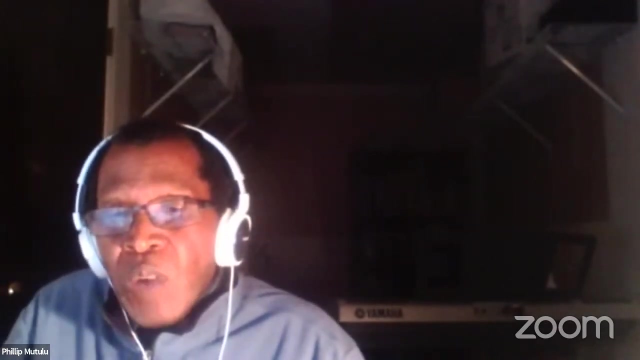 But it is mainly used in design, designing capacities of things like a dam or a culvert. So, for instance, if you want a dam to design a dam, you'll want that dam to have a life, maybe 500 years. 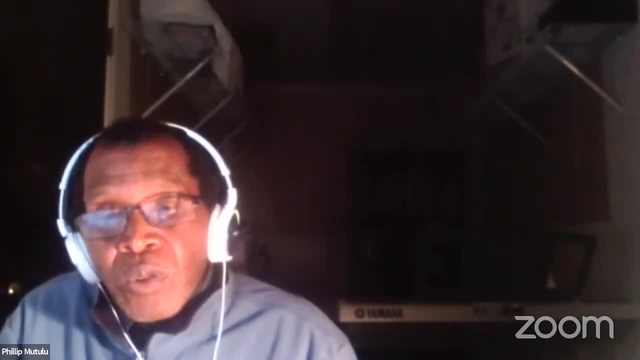 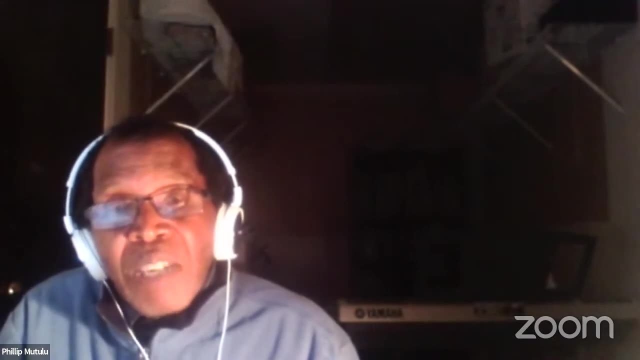 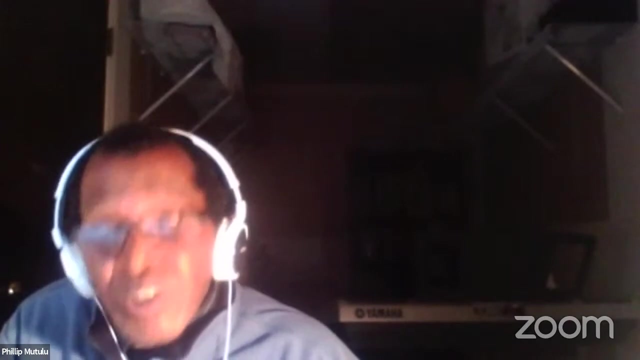 So you would like that dam To be able to have capacity which is sufficient to hold floods that are able to occur during that period of time. So you might want to design your dam to hold to be a 500 year return period, so that a flood that is likely to happen within a span of 500 years will not overwhelm the dam. 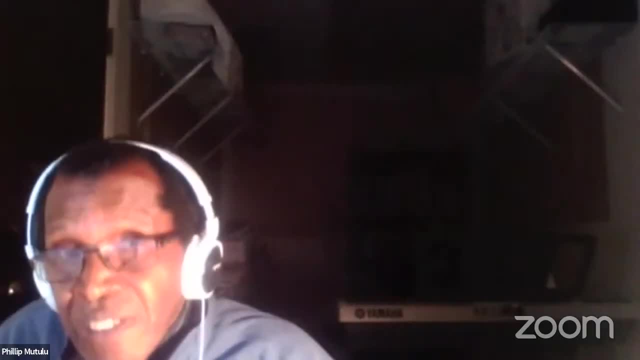 So this time you're not forecasting. It's a kind of a focus, yes, but it's a decision. It's a decision to size your capacity Of your water control structure. So typically, when it comes to forecasting, we don't use return periods, We use the models. But if we are designing any hydraulic structure, then we use return periods because 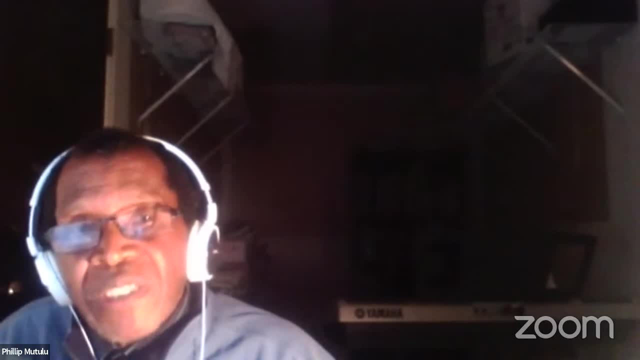 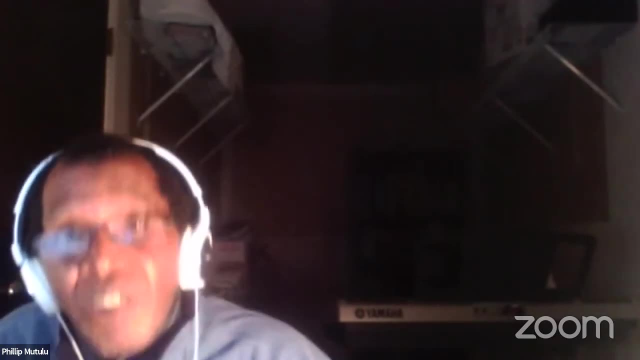 they help us determine the size which is sufficient to hold a flood. But if we are designing any hydraulic structure, then we use return periods because they help us determine the size which is sufficient to hold a flood of a certain magnitude which has an average occurrence of, for instance, 100 years. Okay, 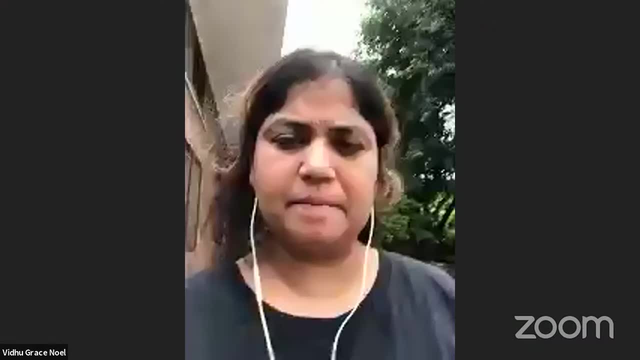 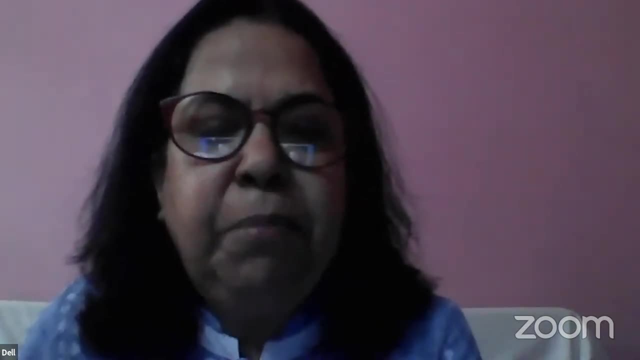 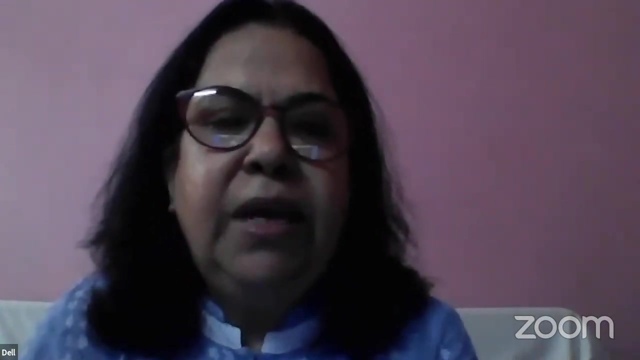 Thank you, sir. Thank you so much Over to you, ma'am. Thank you, Dr Muthulu, for taking all the questions and explaining them in detail even at this late hour in your country. And now I will request Dr Rohan D'Souza. 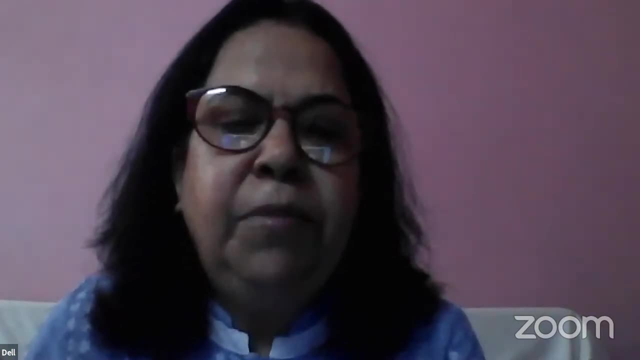 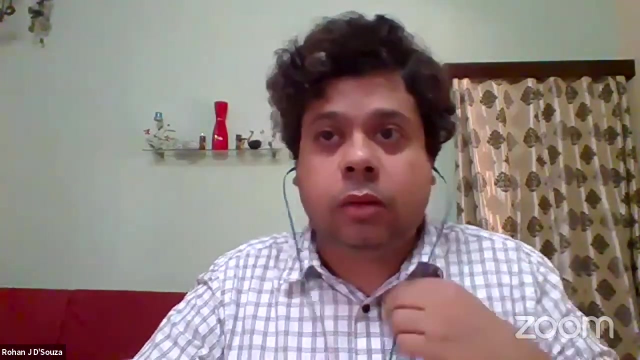 And now I will request Dr Rohan D'Souza and Associate Professor from the Department of Botany, to say the vote of thanks. Thank you, ma'am. Thank you, ma'am, I hope I'm audible. Hello, am I audible? 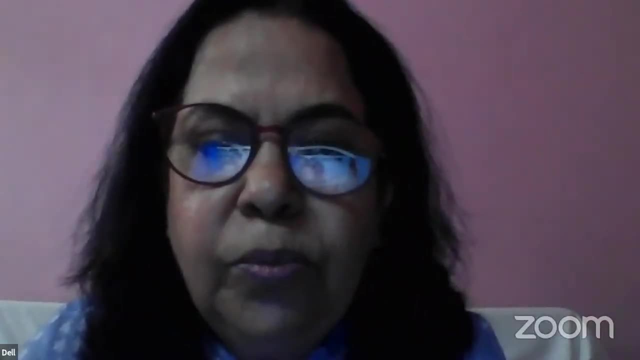 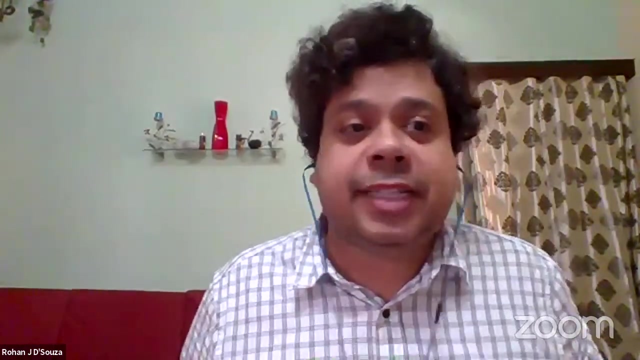 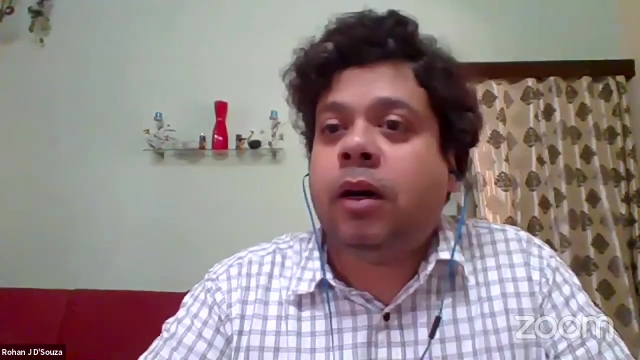 Yeah, Thank you, ma'am. Respected Dr Philip Muthulu, our resource person for today, Professor SP Singh, our Professor SP Singh, our principal, Dr Pierre Majid, the chairperson, Dr Niliya Chauhan, the convener, all our co-conveners and, of course, the participants. 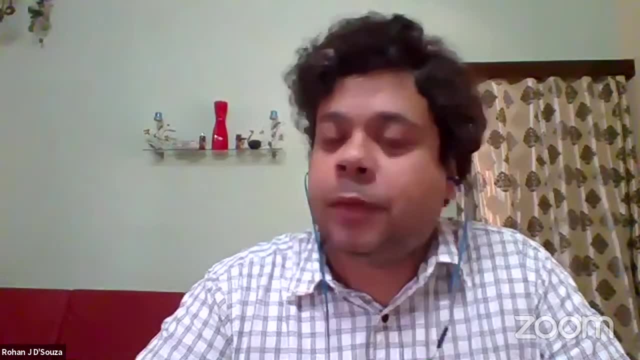 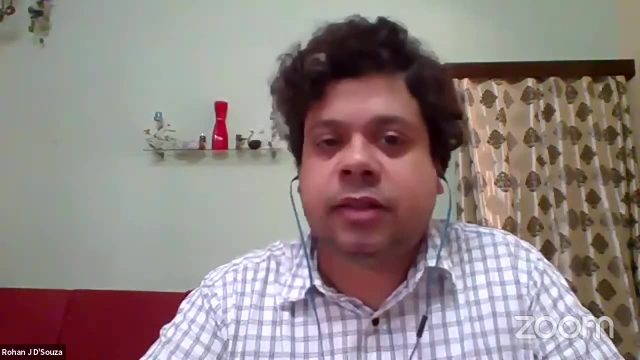 A very good morning to you. A very good morning to you. All good things come to an end, and so has this webinar, And now it's the privilege to propose a formal vote of thanks to such an elite panel of academicians today. 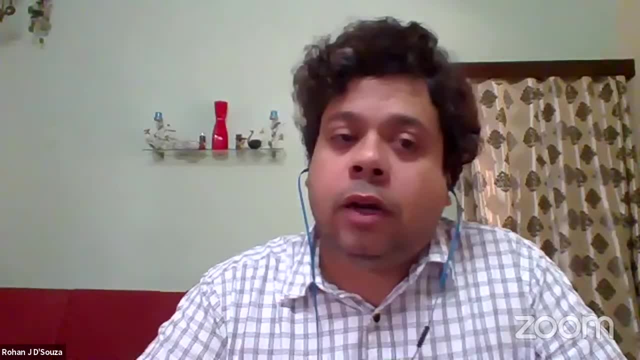 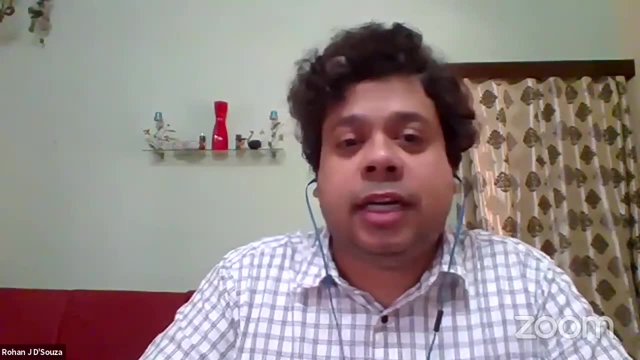 At the onset we all give glory and honor to Almighty God for his many blessings, many blessings, and for keeping us all safe in these precarious times. and this has indeed been a most, uh, informative session, sir. i'm sure dr philip's wonderful slides and lucid presentation. 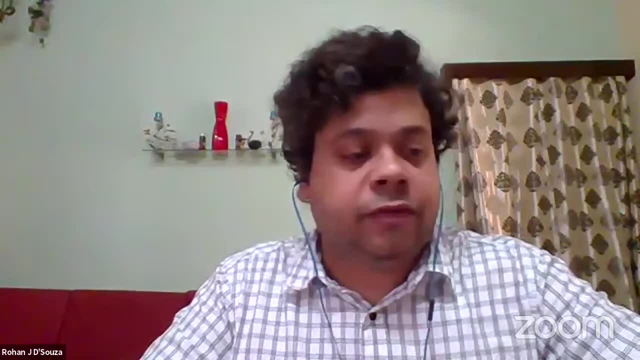 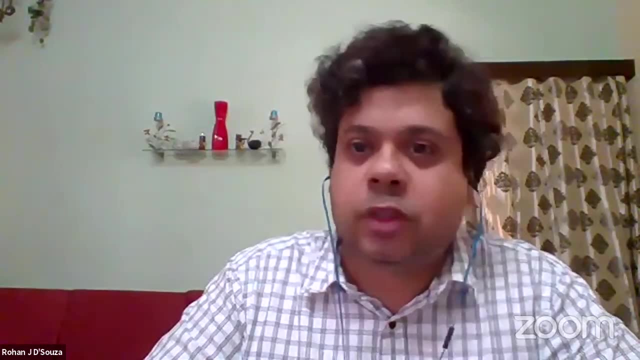 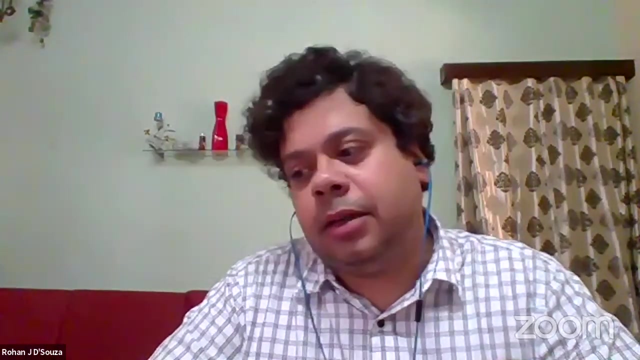 have reached one and all uh, irrespective of their uh fields of work, irrespective of their grasp of the subject. we are happy to have him with us. uh, again, he was with us about a fortnight ago where he talked about flood mitigation and floods. yes, have they? have indeed been a climatist uh. 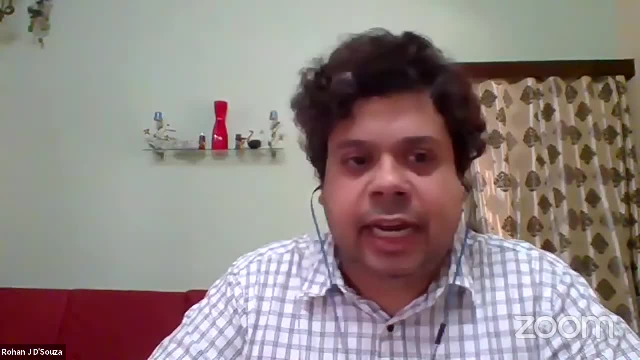 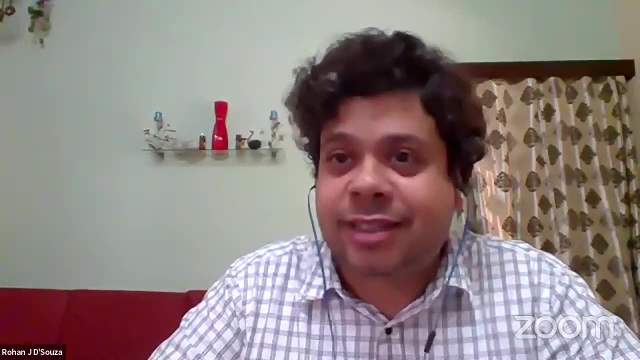 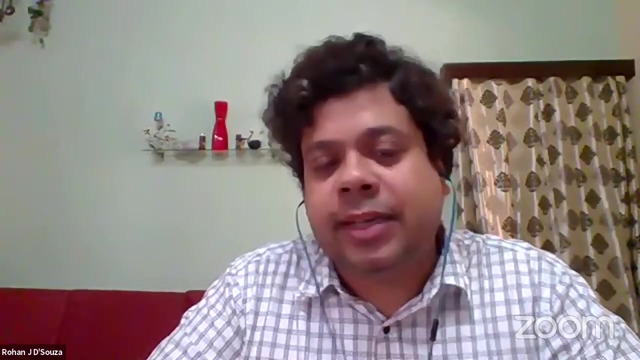 calamitous proposition for mankind, uh, since ancient times, and they find mention in almost all our historic texts, including the bible, and i, for one, was totally engrossed in this uh presentation. on behalf of saint john's college. sir, i take this opportunity to thank you for 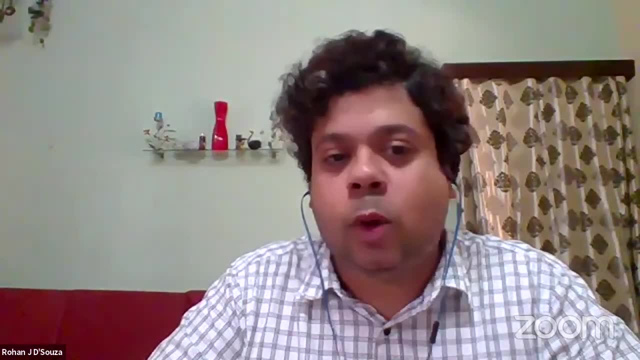 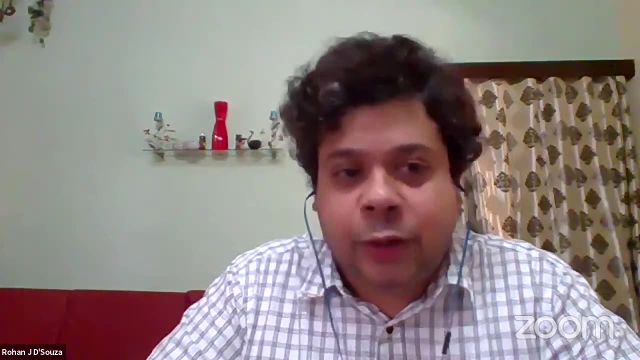 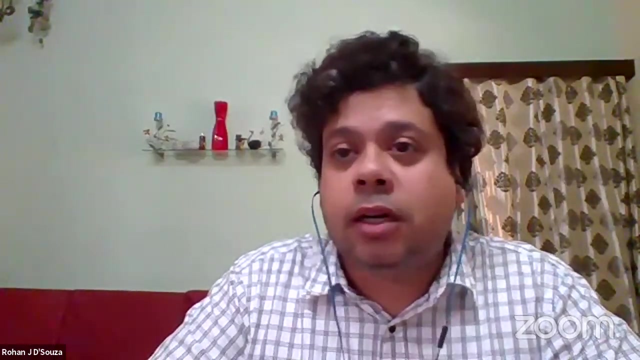 accepting our invitation and for being connected with us at what must be quite a late hour in um in alberta. i suppose it must be almost midnight for you over there. thank you, um. we are deeply indebted to our principal professor s p singh, who, who always has time for us um, however packed his. 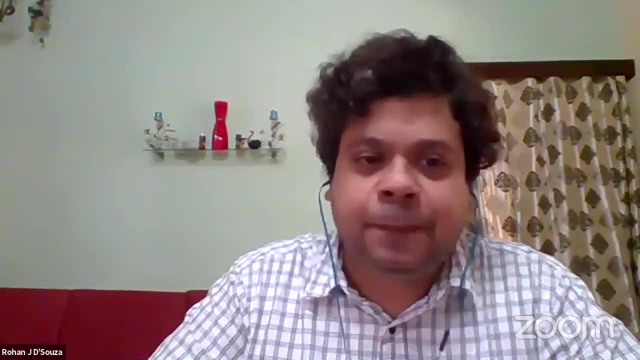 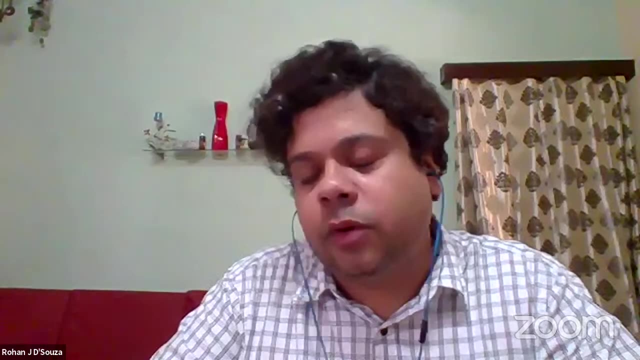 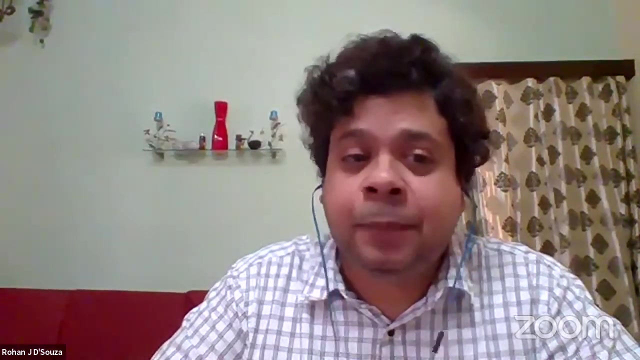 schedule so is a constant source of motivation moving on. uh, any event of these, of this, of such proportions, can of course, not be the work of a single pair of hands. we need the cooperation of many minds, many hands behind the scenes, and heartfelt thanks goes out to our chairperson. 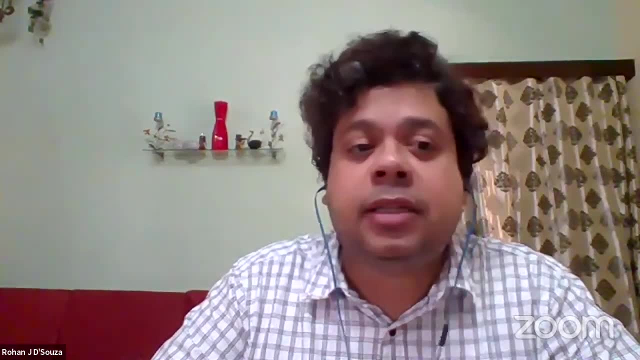 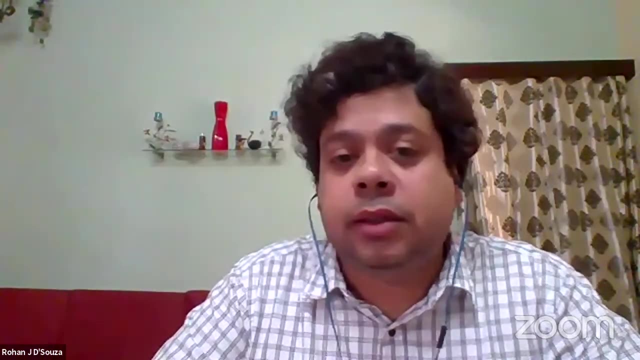 dr p a majid, the head of the geography department, and the, and our convener, Dr Nelia Chauhan, and also a professor in the Geography Department, for being at the helm during this entire webinar series. They've been up at all hours. 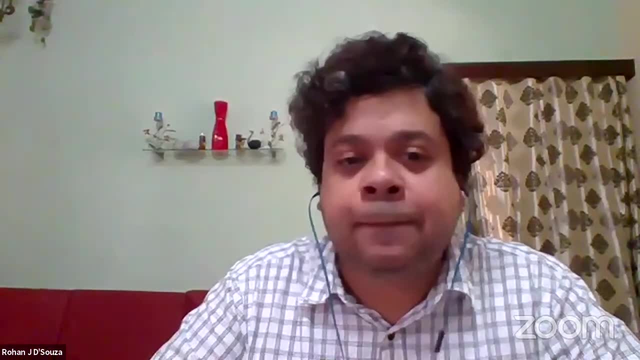 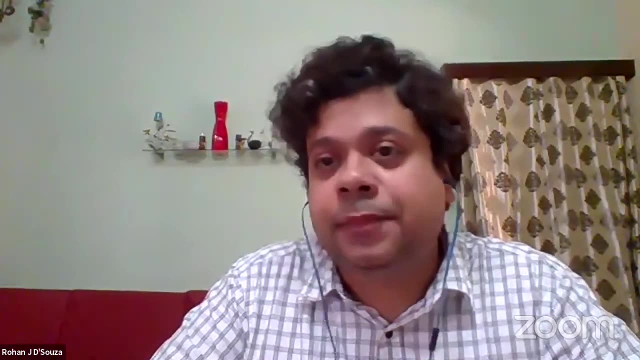 incessantly sharing, collaborating, planning, executing, And to all our co-conveners for their tireless efforts and diligence that have made this webinar successful. a big thank you goes out to you too, And I also thank Mr Sandeep Nayak and Mr Rohit Johnson. 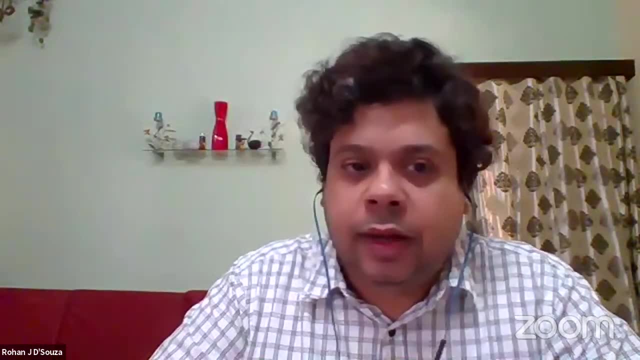 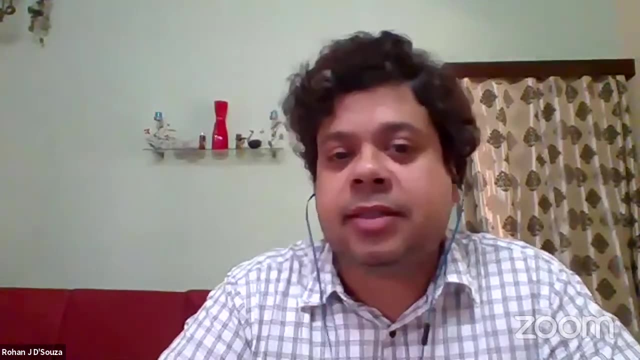 the technical maestros behind today's session. How can we forget all our participants who have joined us from various parts of our country today? But for your presence, this endeavor would have been futile. Thank you for joining us today. Hope you had a fruitful time with us here. 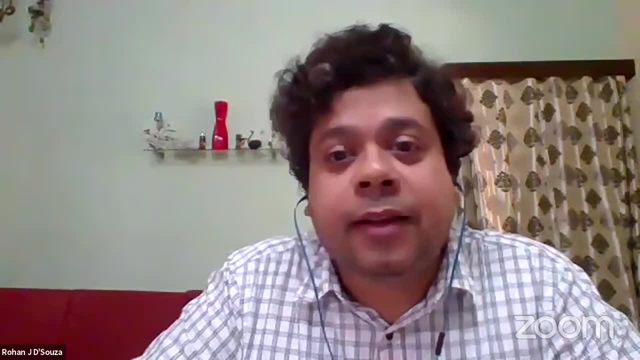 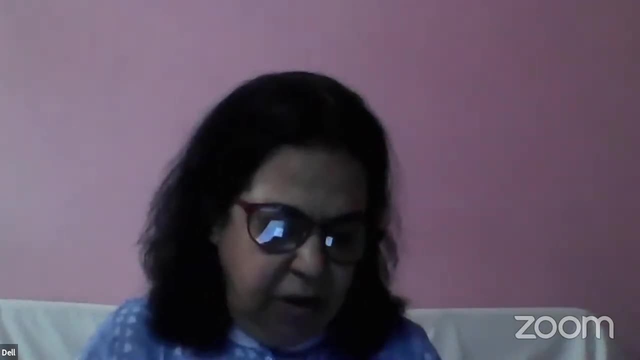 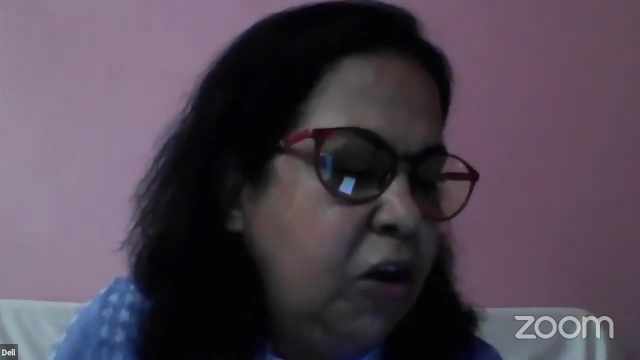 Thank you. Thank you once again. Have a good day. Thank you. There is an announcement: Next Tuesday, there will be a lecture by Professor Atikur from Jamia Miria, Islamia, And he will be. He will be speaking on environmental disaster issues and concerns. 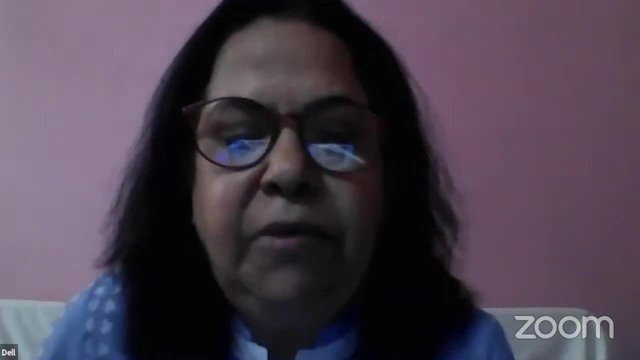 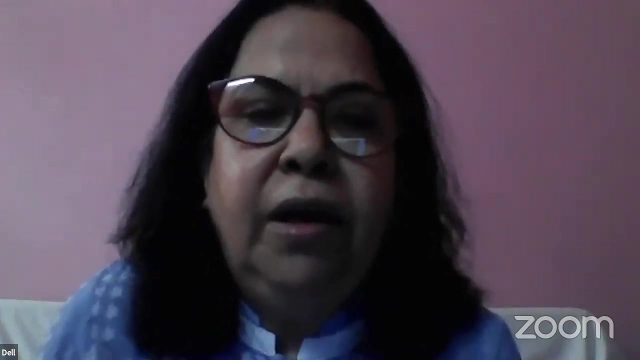 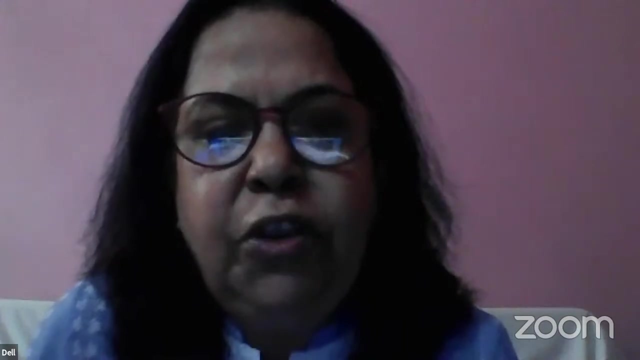 a global perspective at the same time 10 o'clock, And thank you, Dr Muthulu, for being so generous to share further knowledge. I will be in touch with you and we will use your expertise in the future. Thank you. 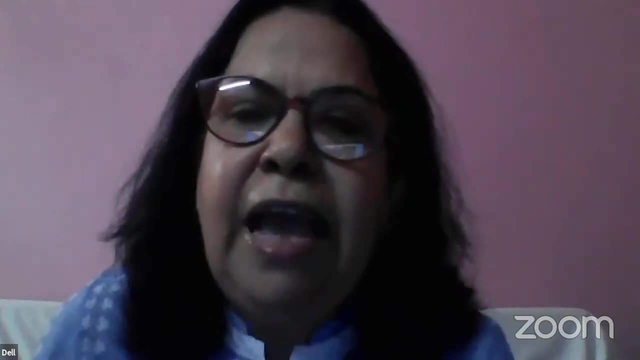 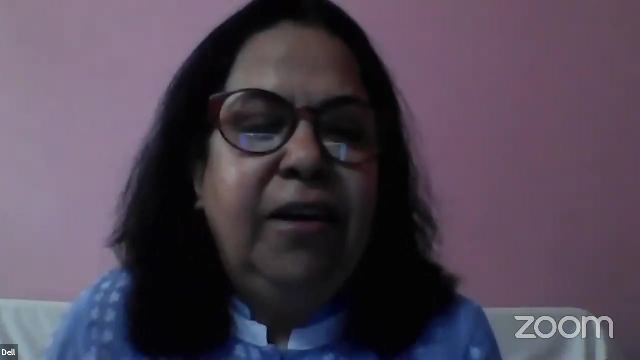 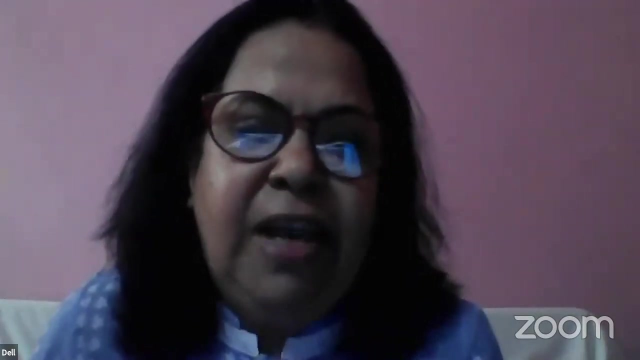 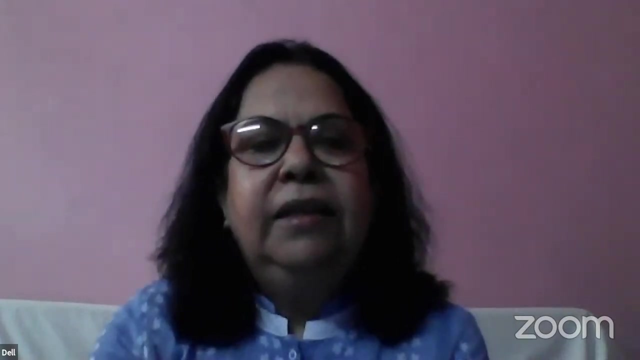 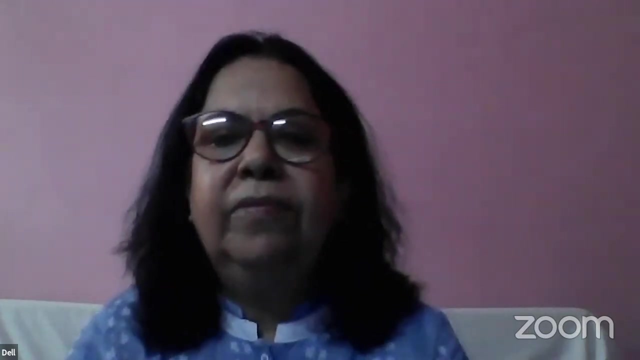 And before we all sign off, we must also thank all our family members who stay muted for so long, And a special thank you to our principal for giving us so much of extra time. Thank you very much, Thank you, Thank you, Thank you very much. 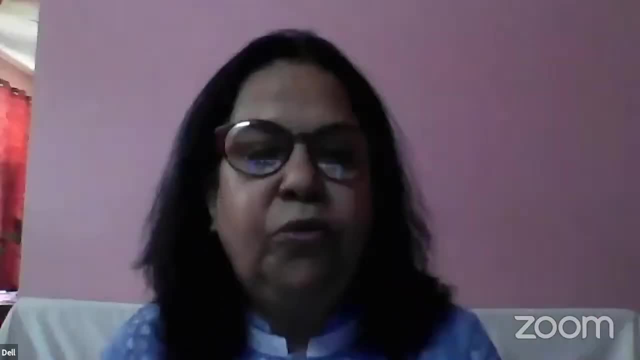 Thank you, sir. Thank you, Thank you, ma'am, And good night to you. Good night, Dr Muthulu. Good night I'm talking to you. Good day, It is 12, 1215 here. 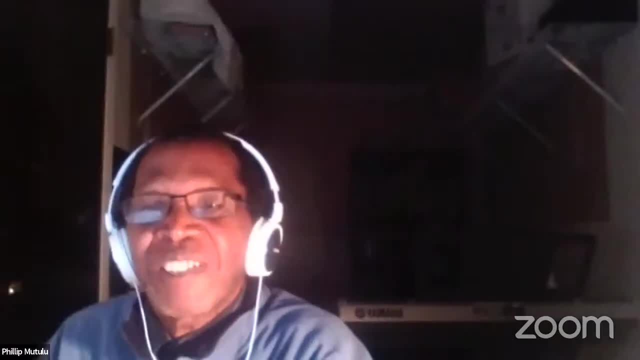 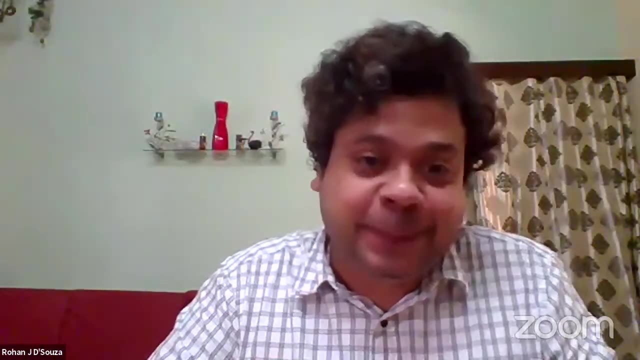 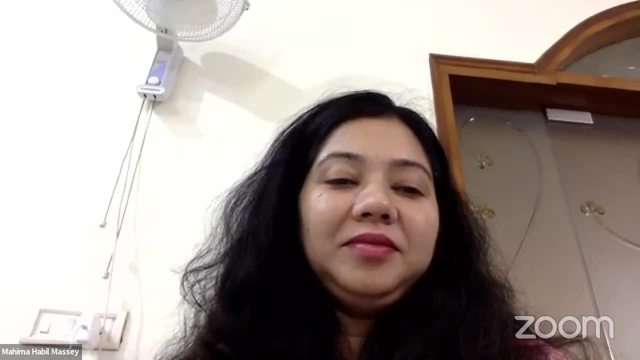 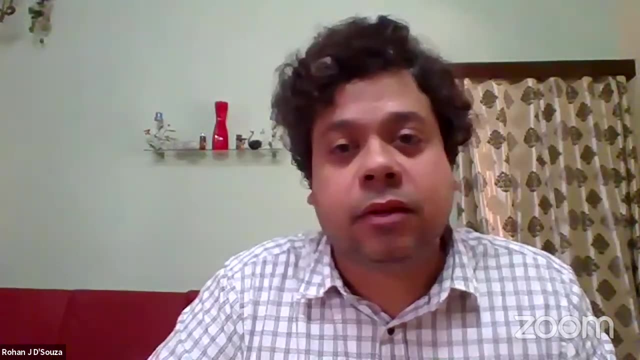